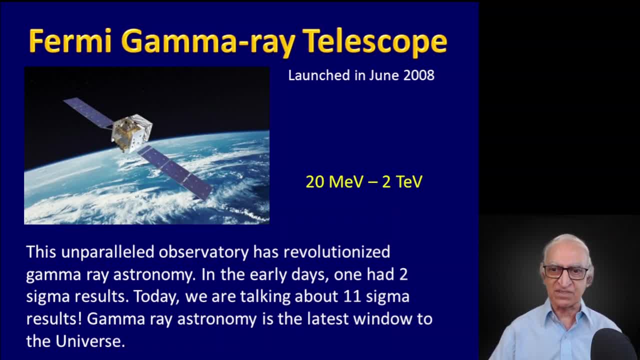 power 12 Ev, So it's an enormous energy range. It operates in the energy range 20 MeV to 2 TeV. 1 TeV is 10 to the power 12 Ev, So it's an enormous energy range. 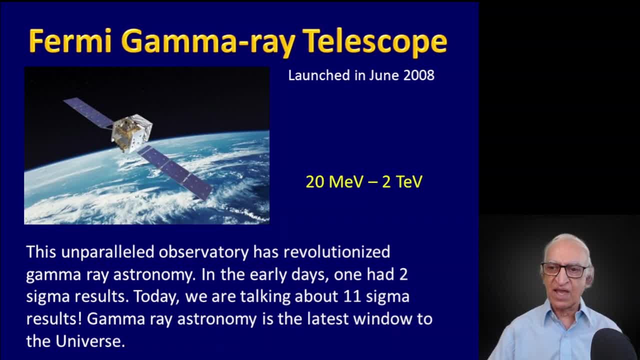 Now this unparalleled observatory has revolutionized gamma-ray astronomy. As I said, till the Compton Gamma-ray Observatory was launched, most of the detections were one sigma or two sigma results. You really need five sigma results before you can be absolutely sure of the detection. Today, with the Fermi-Gamma-ray Telescope, we are talking about 11 sigma results. 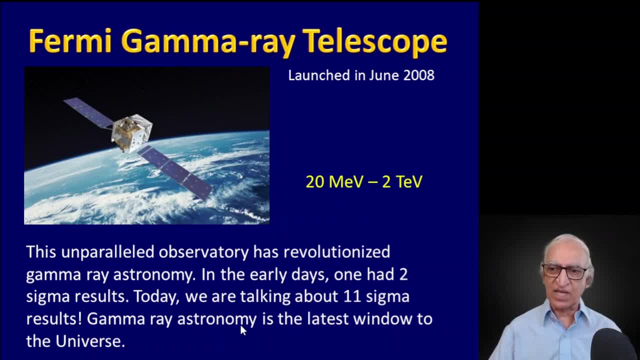 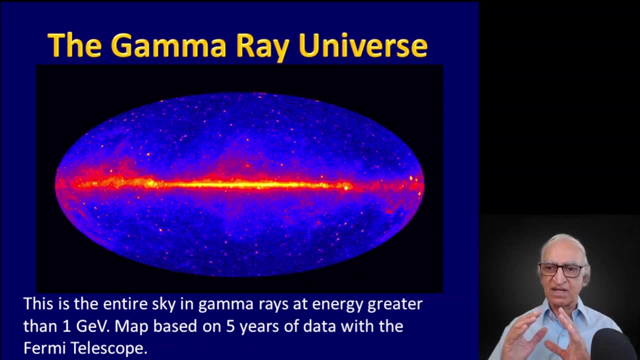 Today, with the Fermi-Gamma-ray Telescope, we are talking about 11 sigma results. So gamma-ray astronomy has come of age and is now the latest window to the universe. Now this is the gamma-ray universe. This map taken based upon five years of continuous data. 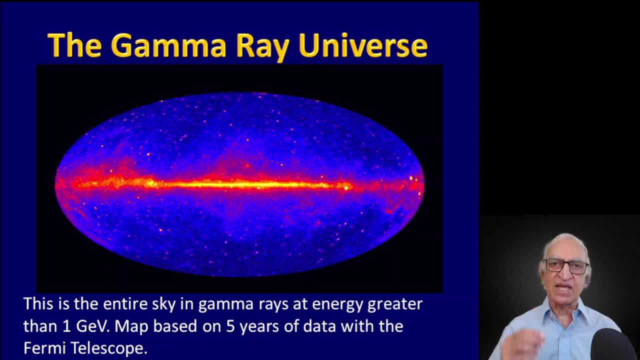 with the Fermi Large Area Telescope, is the entire sky, the entire universe in gamma rays at energy greater than 1 TeV is the entire sky, the entire universe in gamma rays at energy greater than 1 TeV is the entire sky, the entire universe in gamma rays at energy greater than 1 TeV. 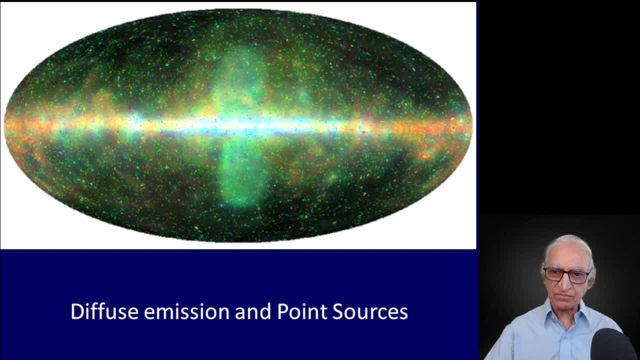 Now let's look at this a little more carefully. Now the gamma-ray emission of the sky can be decomposed into two parts. One: there is diffuse emission and then there are point sources. In this slide you clearly see diffuse emission and then you see thousands and thousands of point sources. Let us see. 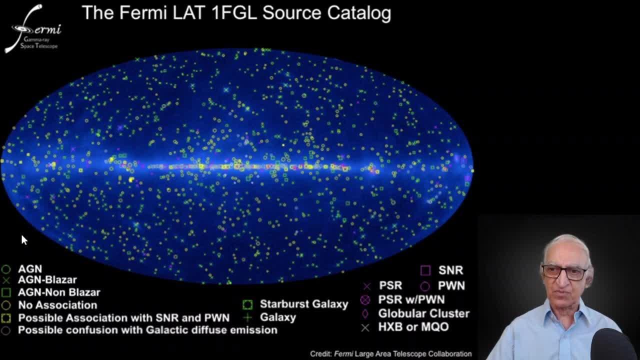 the point sources a little more clearly. Let us see the point sources a little more clearly. In this slide, what you see here are active galactic nuclei in this slide. what you see here are active galactic nuclei, blazar's supernova remnants than supernova pulsars, global clusters, high-mass X-ray binaries. 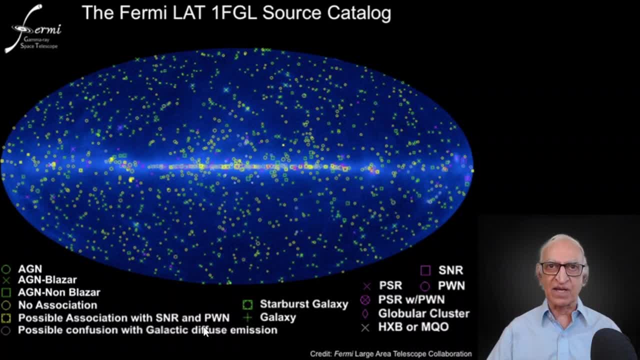 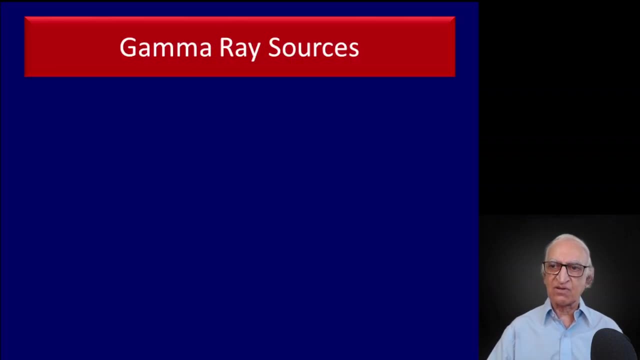 galaxy starburst galaxies, diffuse emission from galaxies and what-have you? galaxy starburst galaxies, diffuse emission from galaxies, what-have you? This is a catalogue of the Fermi Large Area Telescope, a catalogue of point sources. Now let us dig into what are these gamma-ray sources? They are either young pulsars, as I said. 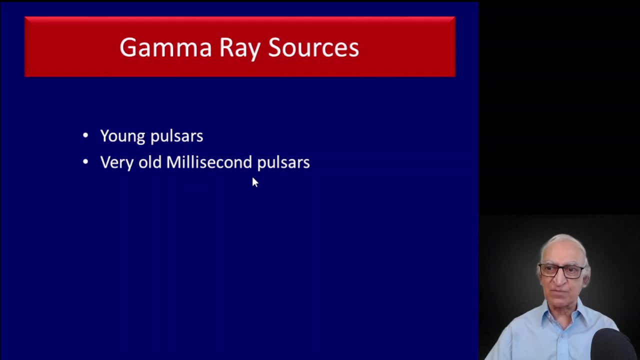 very old millisecond pulsars, supernova remnants, the interstellar medium of our galaxy and external galaxies, active galactic nuclei, quasars and, of course, gamma-ray bursts and, more recently, gamma-ray bursts from two neutron stars spiraling in, emitting. 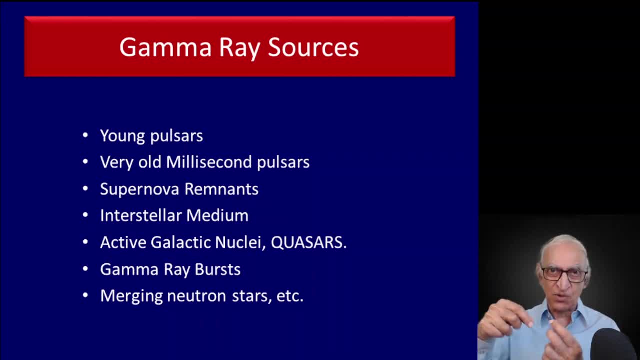 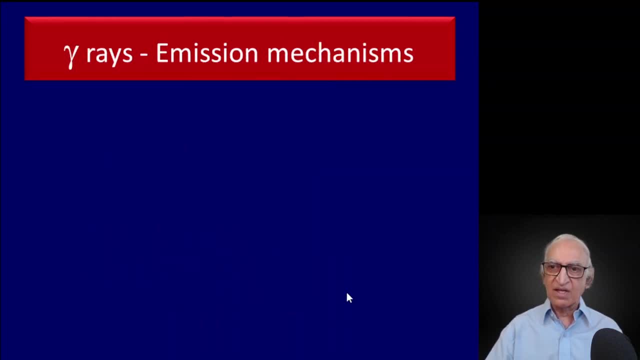 gravitational waves. Now, what are the emission mechanisms that produce gamma-rays? Well, there is our good old synchrotron radiation, where relativistic electrons are gyrating in a magnetic field. We saw that the Crab Nebula emits gamma-rays. The Crab Nebula emits gamma-rays. 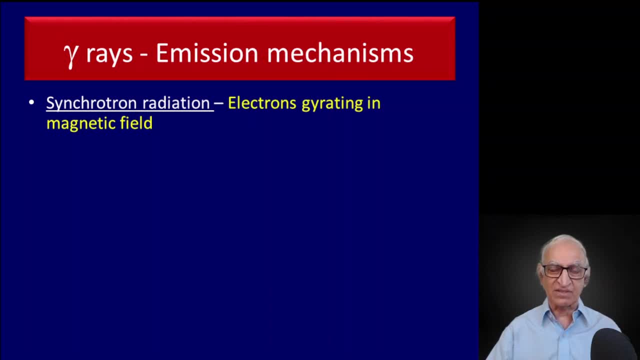 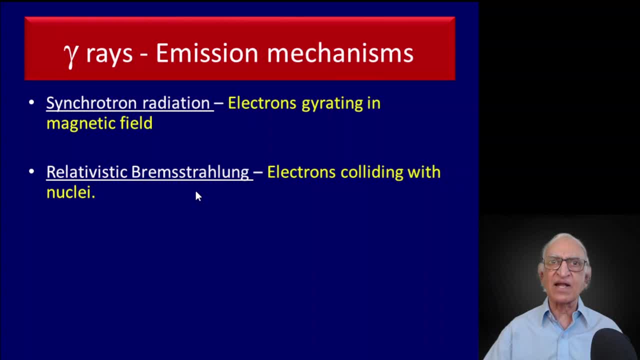 is also synchrotron radiation. Then you have relativistic Bremsstrahlung electrons, relativistic electrons colliding with ions, Coulomb collisions. Then there is a very important mechanism, which we shall now discuss, which is the decay of neutral pie meson. 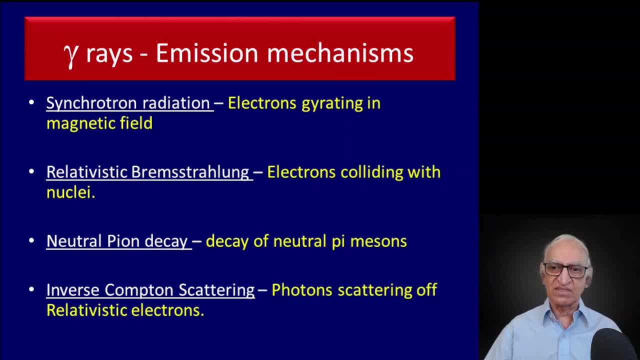 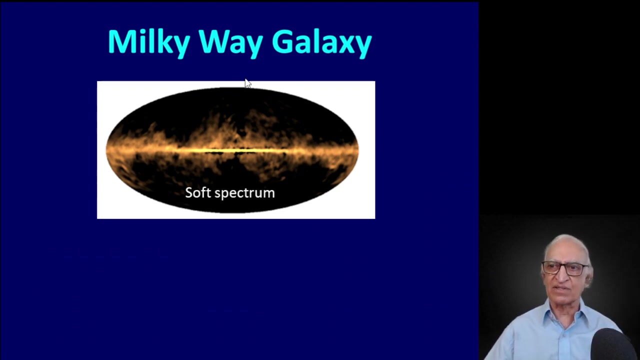 And finally, there is inverse Compton scattering. There is nothing inverse about it, but it is really Compton scattering, and we shall spend a good fraction of this lecture discussing Compton scattering, which is the photon scattering of relativistic electrons. All right, now let's look at the gamma-ray emission from our galaxy, the Milky Way galaxy. 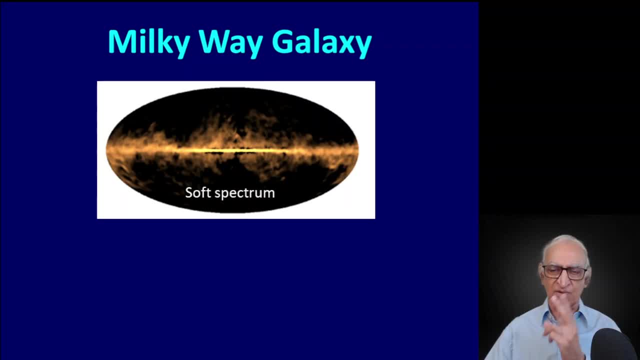 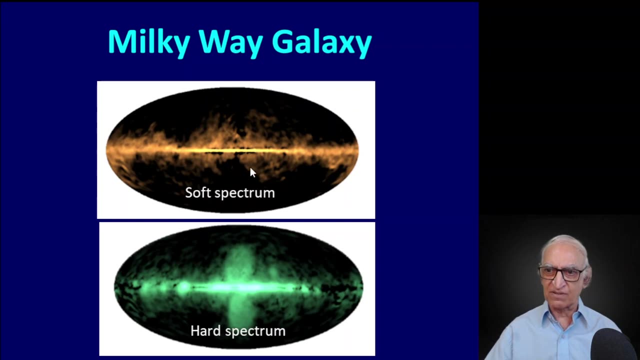 There are two components to gamma-ray emission from our galaxy. One: there is a soft spectrum that means the energy range in this picture is lower energy- gamma-rays- And then there is a hard spectrum which looks very different. If you compare the two, it looks very different. 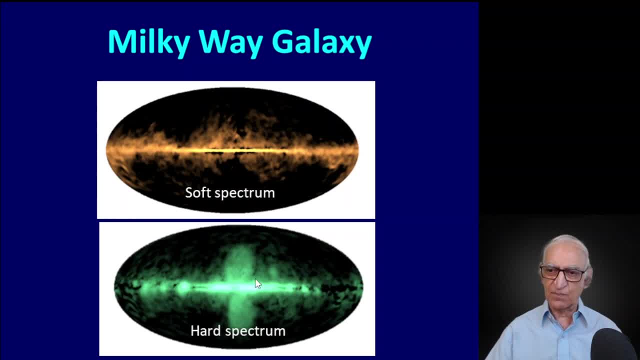 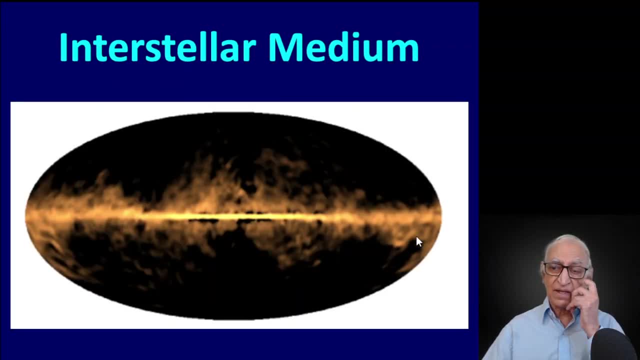 Most noticeably, there is this dipole-like structure at the center of the galaxy. Now let's look at gamma-ray emission from the Milky Way galaxy. This is the interstellar medium of our galaxy, the Milky Way galaxy, and that's what is shown. 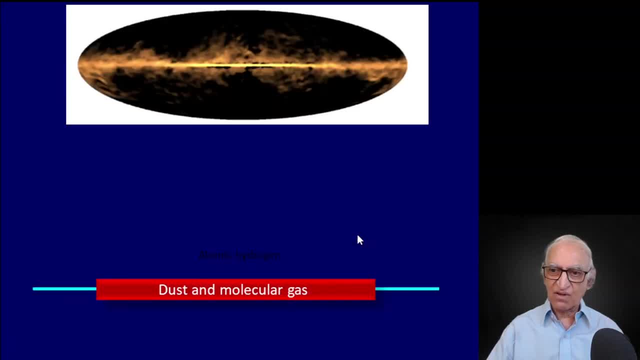 over here. Now it is the same thing that is shown over there. We shall soon discuss the mechanism, the radiation mechanism, that is responsible for gamma-ray emission from the interstellar medium. As we shall see, it has to do with the interaction of cosets. 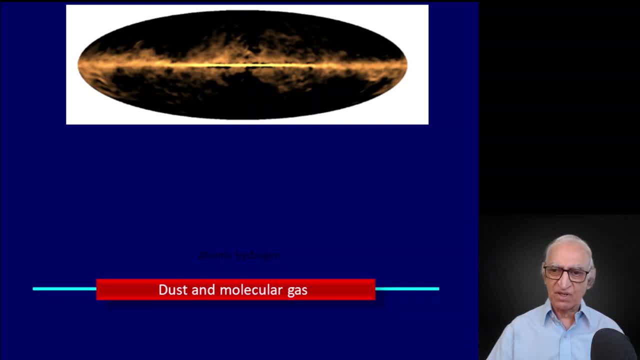 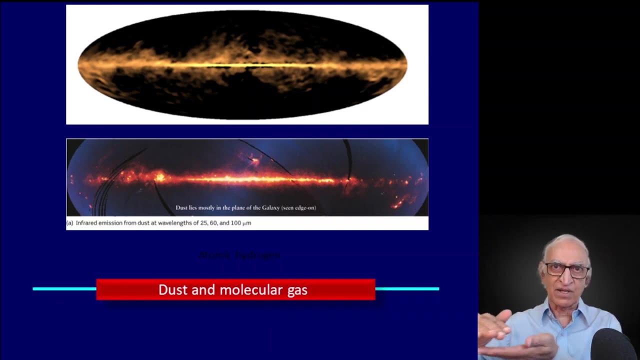 The interaction of cosmic ray particles, protons in particular, with molecular gas in the interstellar medium. If you remember, the molecular gas is a rather thin layer about the plane of the galaxy, only about 60 parsecs. Of course the neutral hydrogen layer is very thick, but the molecular gas and associated 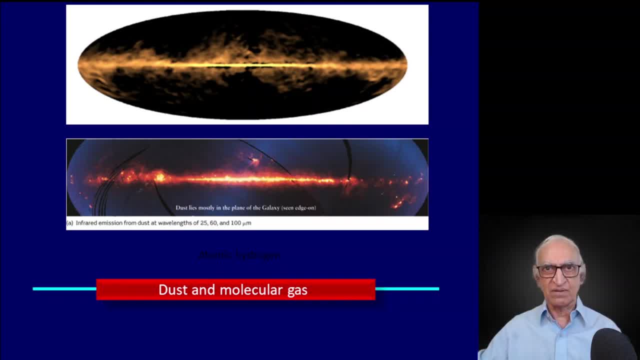 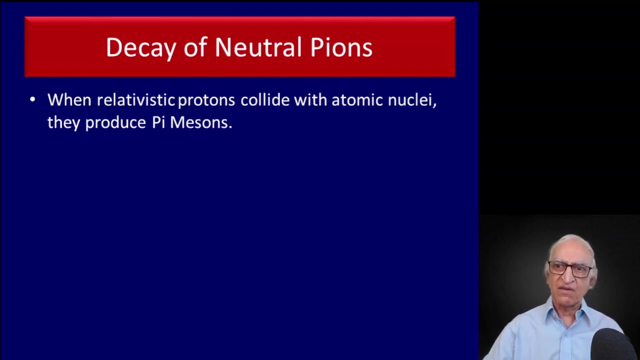 dust is a fairly thin layer And that can be seen very prominently through the infrared emission emanating from the dust, as well as diatomic molecules. Now let us discuss the emission mechanism from the interstellar medium. Well, relativistic protons. These relativistic protons probably come from extragalactic particles. 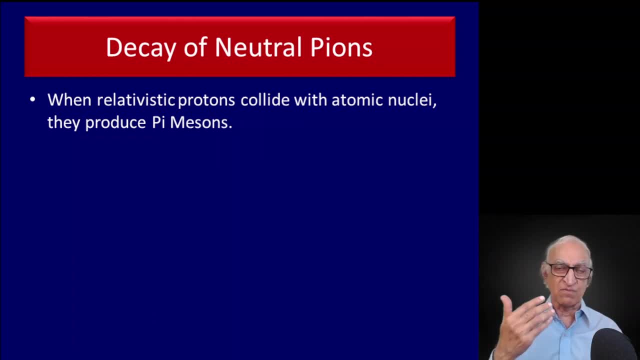 They come from extragalactic energetic sources, from nearby pulsars or what have you. They collide with atomic nuclei in the interstellar medium, in the molecular clouds, And they produce pi mesons. Now pi mesons come in three varieties. 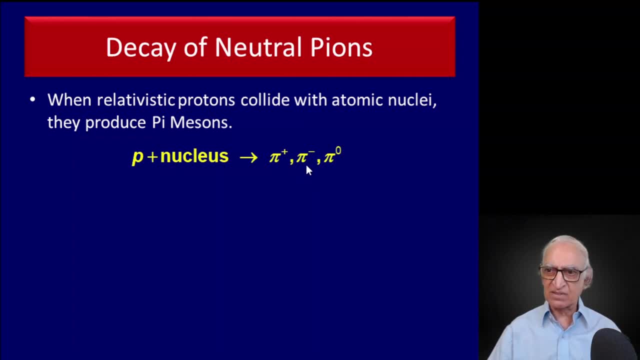 They are either pi plus, pi minus or neutral pi mesons, which is the pi zero mesons. Now charged pi mesons- pi plus or pi minus, decay to mu mesons, which are lighter than the pi mesons and neutrinos, and the mu mesons in turn decay to electrons or positrons. 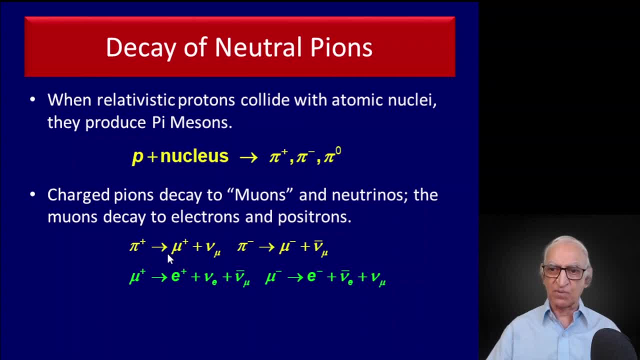 And that is shown over there. Pi plus, for example, decays to mu plus and a muon neutrino. pi minus decays to mu minus and a muon antineutron, And then the muon decays to a positron plus an electron neutrino. 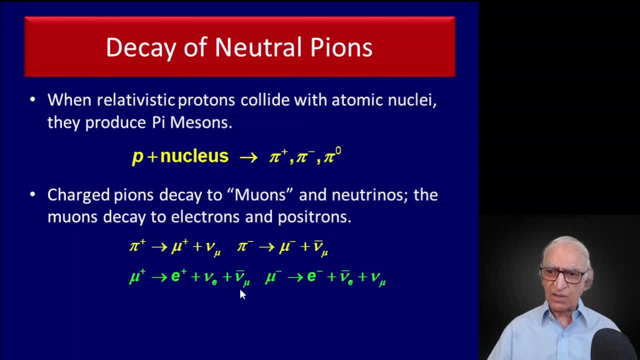 And of course you have a muon antineutrino. We are not discussing neutrinos at all in this lecture. I just want to say that the mu mesons produced in the decay of pi mesons, charged pi mesons, eventually decay to positrons and electrons. 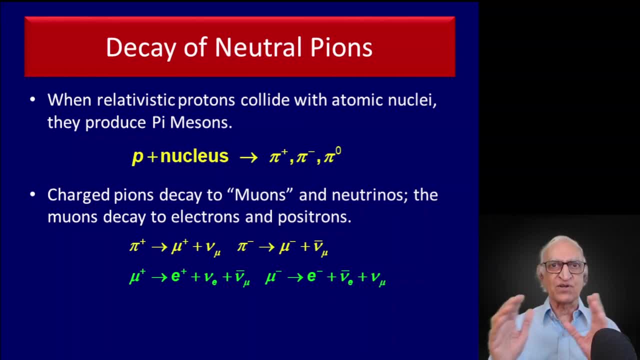 And they may produce some muons, some radiation which we are not tracking in this particular lecture. Now let's concentrate on the pi zero meson, the neutral pi zero meson. Now, it is well known that a neutral pi zero meson decays to two gamma rays. 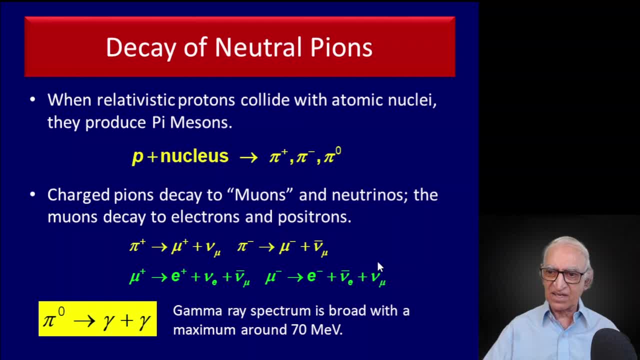 and the energy spectrum of the gamma rays produced in this reaction is rather broad and peaks around 70 million electron volts. So when you look at the interstellar medium and it is glowing in gamma rays, it is really glowing at an energy of around 70. 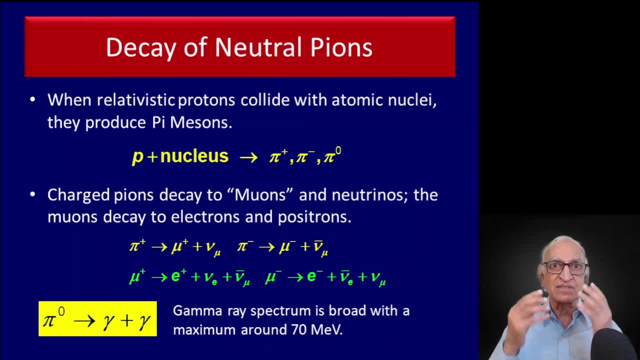 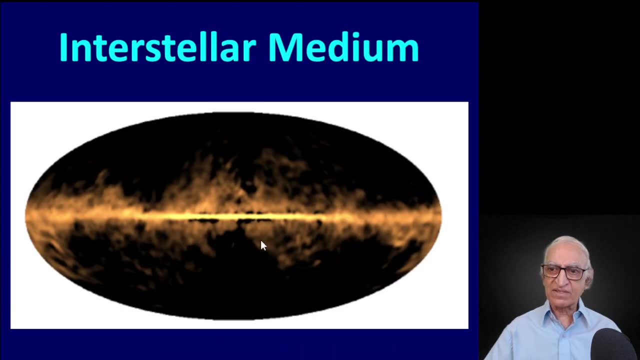 MeV, and what is really happening is that the pi zero mesons, which are produced by the collision of relativistic protons with the nuclei in molecular clouds, decay to two gamma rays. Now that's the interstellar medium over there and that's the diffuse emission due to pi zero decay. 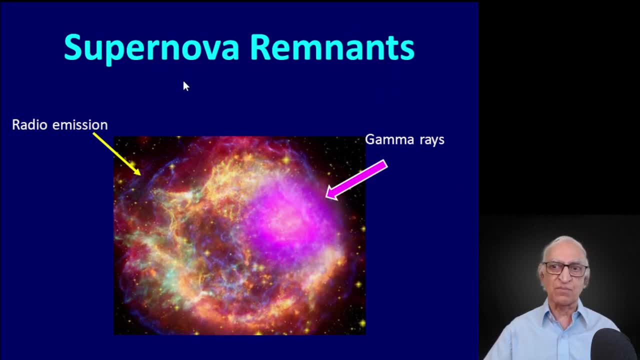 But supernova remnants which we discussed in the previous lecture, which of course are well known through the synchrotron radio emission which you see over there. This is Cassiopeia A, which we discussed in several contexts. but these supernova remnants also emit gamma rays. 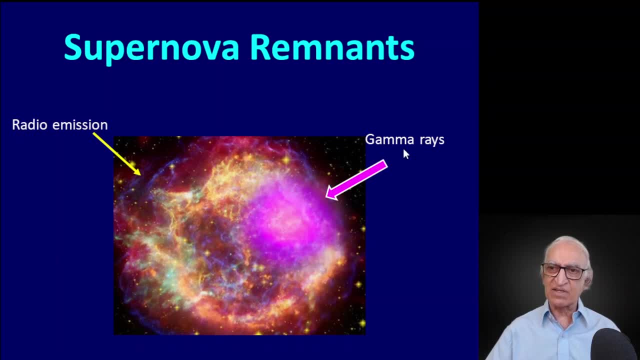 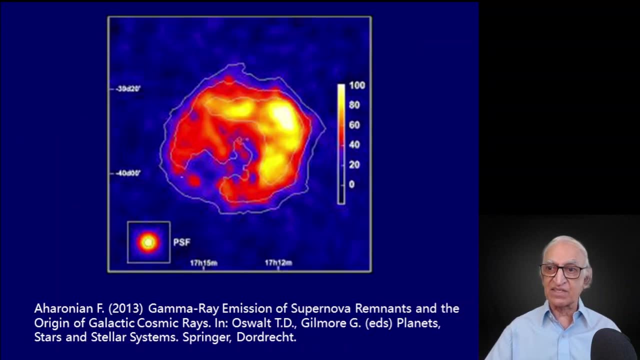 And that magenta color over there is gamma rays from Cassiopeia A detected by the Fermi Large Area Telescope. Here is another supernova remnant. This is the false color image. The lighter colors are more intense regions. It's a gamma ray emission of some supernova remnant and the gamma 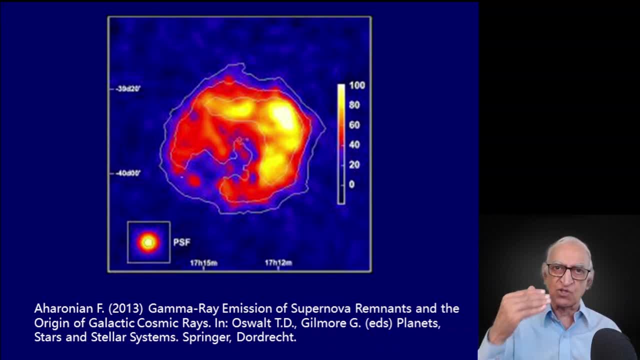 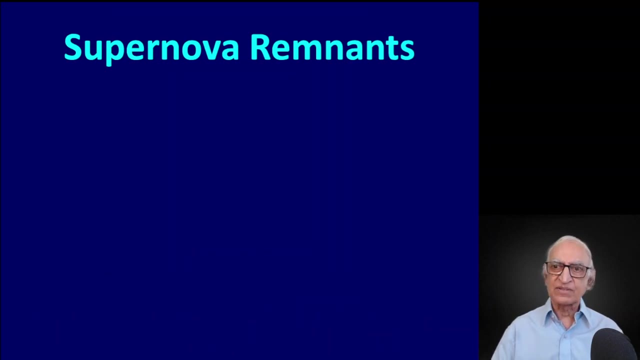 emission is again due to the interaction of cosmic rays with the molecular gas with which the supernova remnant is interacting and ramming into, possibly, a molecular cloud. Now let us discuss supernova remnant. As I said, the Fermi telescope has detected gamma rays from more than 30 supernova remnants. 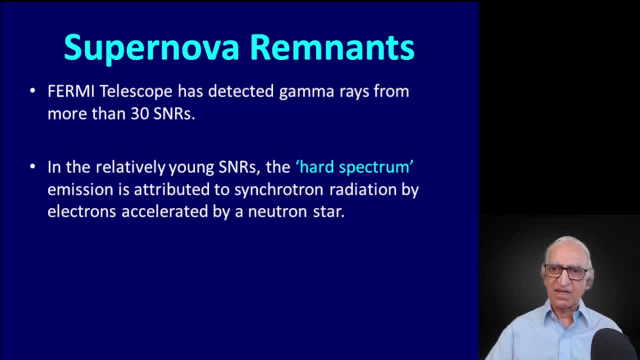 in our galaxy, In the relatively young supernova remnants like the Crab Nebula, for example, the spectrum is very hard. In other words, you have gamma rays up to high energy. This can be attributed to synchrotron radiation by electrons accelerated by a neutron star. 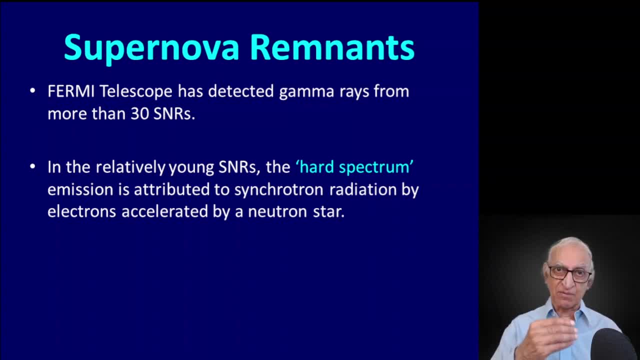 We know that the Crab Nebula emits gamma rays From near the light cylinder. let us note what I am talking about now. These charged particles are finally deposited into the Crab Nebula and there they radiate by gyrating in the magnetic field of the Crab Nebula through synchrotron radiation. 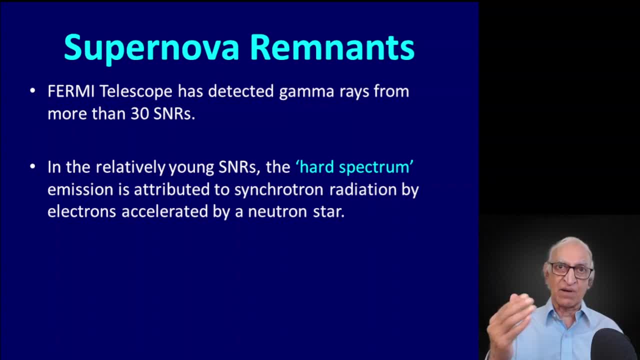 Of course you need very high energy particles and very strong magnetic fields before the synchrotron radiation can be observed. Now let us look at the Crab Nebula. The Crab Nebula emits gamma rays at as high an energy as gamma rays. That is only possible in very young supernova remnants like the Crab Nebula. 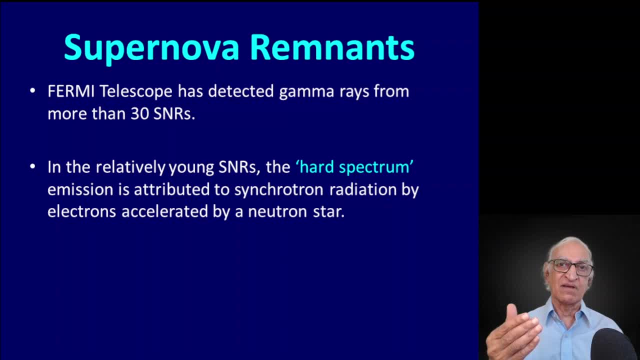 In older supernova remnants the electrons do not have that high an energy and the magnetic field strength is also decayed due to adiabatic losses as the supernova remnant expands. Therefore you do not get any synchrotron gamma ray emission from older supernova remnants. 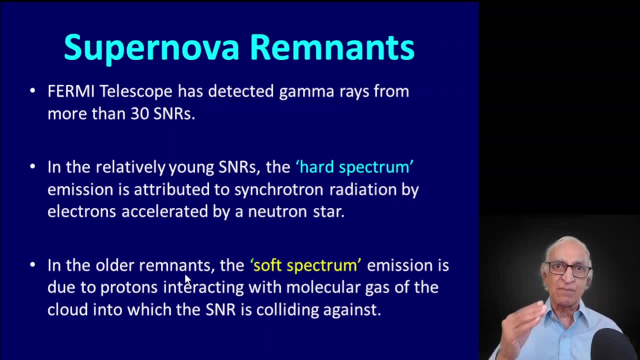 You do get gamma ray emission from older supernova remnants, but they are softer in the spectrum, In other words, the energy of the gamma rays is much lower. Careful examination tells us that this emission is due to cosmic ray protons interacting with 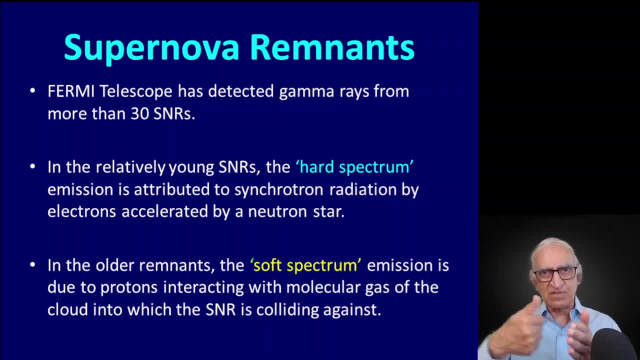 the molecular gas into which the supernova remnant is ramming into in the interstellar medium. So it is really not gamma ray emission. It is not. It is not a gamma ray emission from the supernova remnant itself, but it is a gamma ray emission. 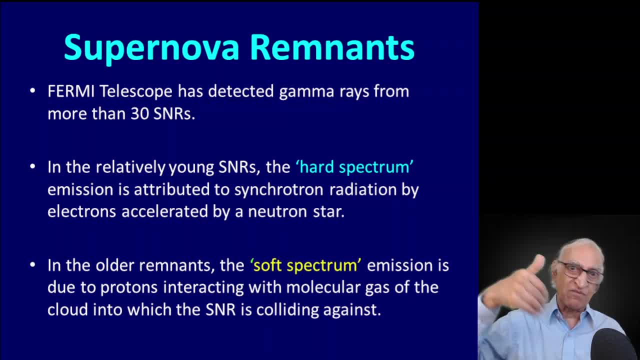 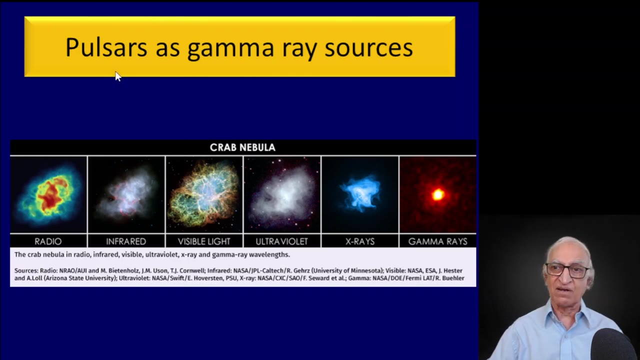 from the periphery of the supernova remnant, where you have a compression of the magnetic field of the molecular cloud because it is being rammed by a supernova blast wave and then the protons are gyrating in that magnetic field. Of course young pulsars like the Crab Pulsar. 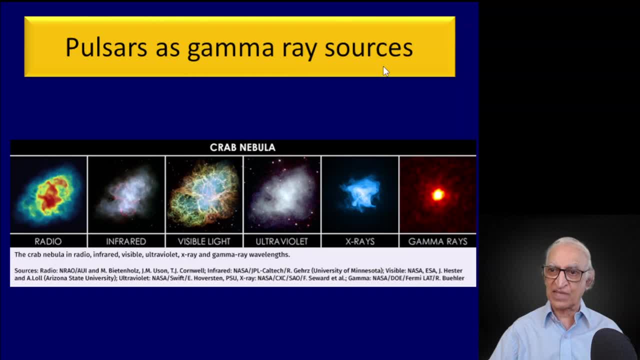 They are powerful sources of gamma rays. Here is, of course, the Crab Nebula, seen in the entire electromagnetic spectrum at radio wavelength, infrared, visible wavelength, ultraviolet X-rays, soft X-rays and hard X-rays and, of course, low energy and ultra high energy gamma rays. 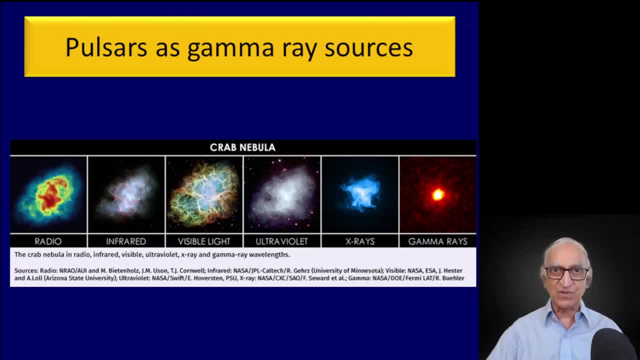 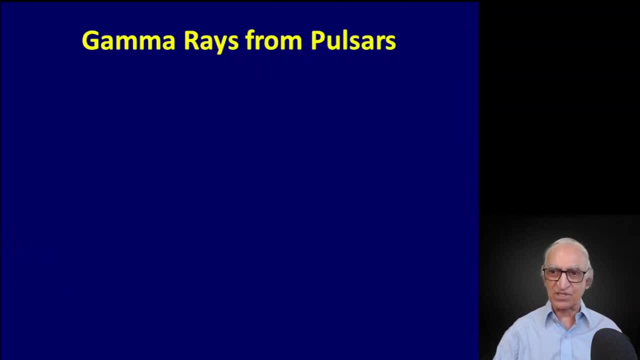 This is the Crab Nebula, But the Crab Pulsar is also a gamma ray emission. This is the Crab Nebula. This is the source of pulsed gamma ray emission. Now, the emission from pulsars is clearly synchrotron radiation, and this radiation emanates. 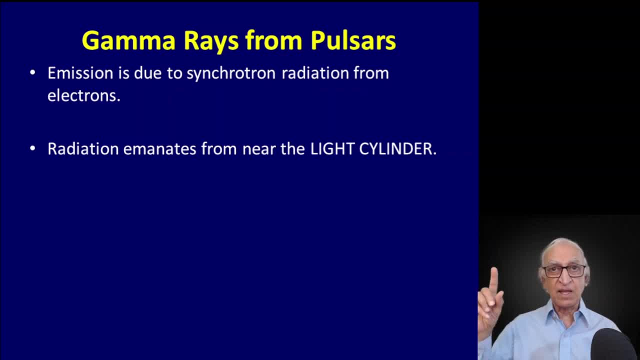 not from near the surface of the neutron star, but far away, near the light cylinder. Let me remind you in a minute about the light cylinder in case you have forgotten. Now gamma rays are produced. They are produced near the surface of the neutron star by relativistic electrons. that 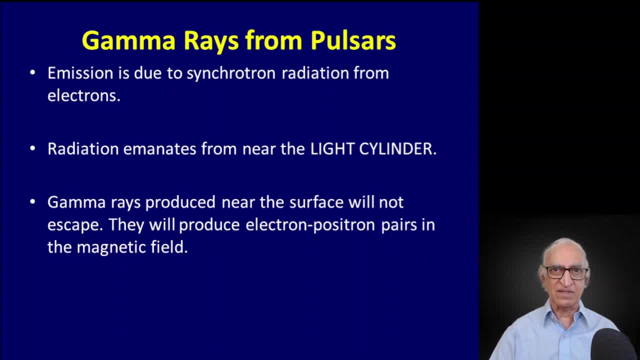 are accelerating along curved magnetic field lines. But these gamma rays are absorbed by the magnetic field themselves and they produce electron positron pairs which finally radiate at radio wavelengths. So the gamma rays produced very near the surface of the neutron star do not really get out. 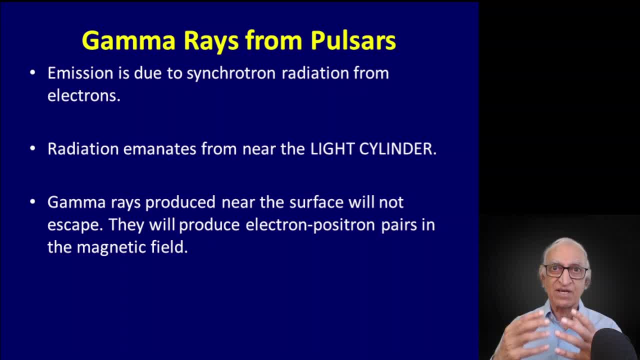 because the magnetic field has a very large optical depth For the photons. only large area telescope has detected gamma rays not only from the Crab Pulsar, which is an old story, but from several young pulsars, nearly a dozen or so. 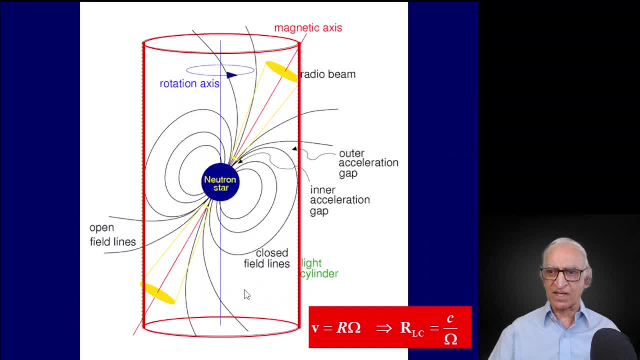 young pulsars. Now let me remind you once again about the light cylinder. Here are the magnetic field lines of an inclined neutron star. This is the rotation axis of the neutron star. The light cylinder is what is shown in red, and the radius of the light cylinder is such: 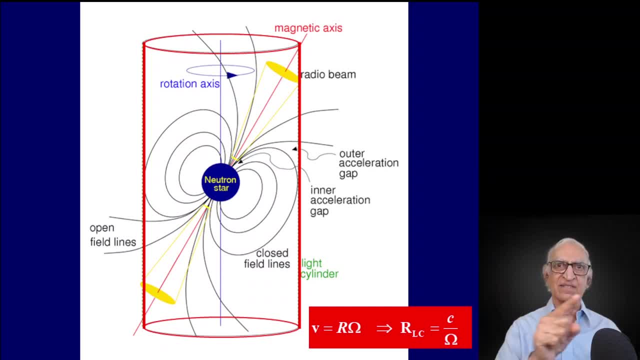 that if a particle were co-rotating with the central neutron star at that radius, it would be going at the speed of light, In other words, the circular or tangential velocity v, which is equal to the velocity which is equal to r, omega. that v will be equal to c, the speed of light. 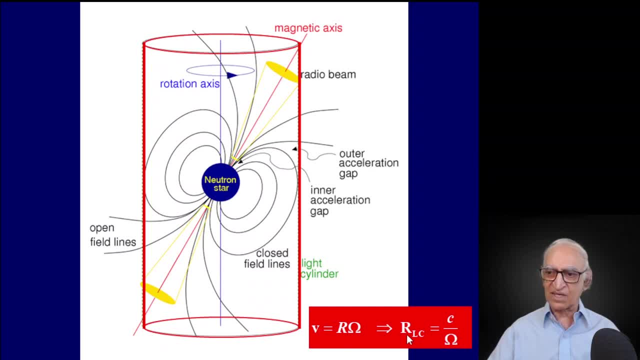 Therefore, if I solve this equation, I will get the radius at which the velocity becomes equal to c. Therefore, the radius of the light cylinder is c over omega. The faster the pulsar spins, the larger is omega, the closer is the light cylinder. 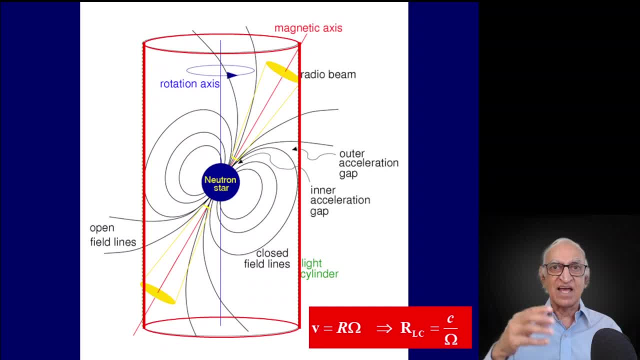 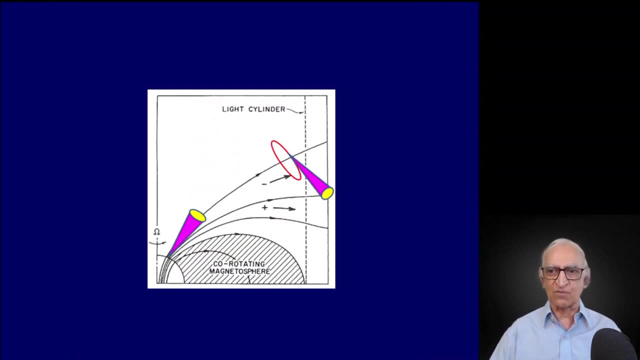 As the neutron star slows down and its period lengthens and omega increases, the light cylinder radius will increase proportionately. Now why am I bringing in this light cylinder now? This is just to remind you of what we discussed in our lecture on pulsars. 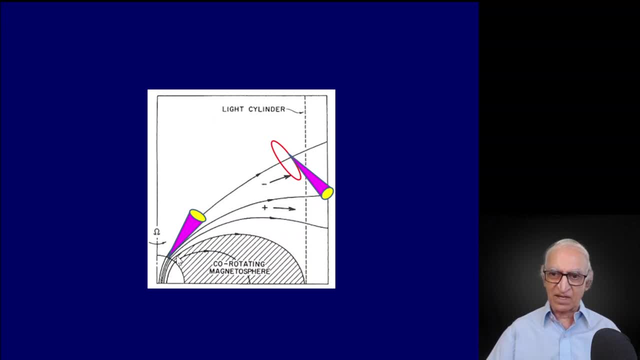 Here is the central neutron star. There are gamma rays produced very close to the neutron star surface. Near the star the magnetic field is very strong. The charges are not allowed to cross the field lines because the Lorentz force is very, very. 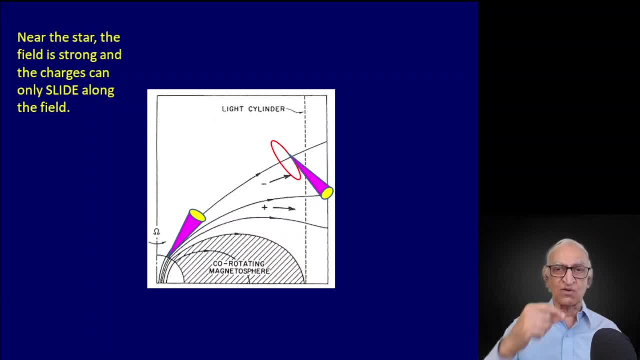 strong. They can only slide along the curved field lines. And since the field lines are curving, these electrons will radiate. They will radiate into a narrow cone and the width of the cone will be the angle. opening angle of the cone will be 1 over gamma, where gamma is the Lorentz factor: 1 over square. 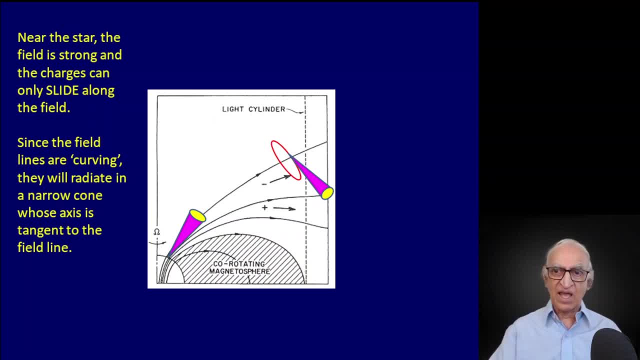 root of 1 minus v squared by c squared, and therefore the radiation is essentially emitted in a tangential direction to the magnetic field. Now, this is how the radio radiation from the pulsars are produced. These gamma rays decay into electron-positron pairs and they in turn produce much lower. 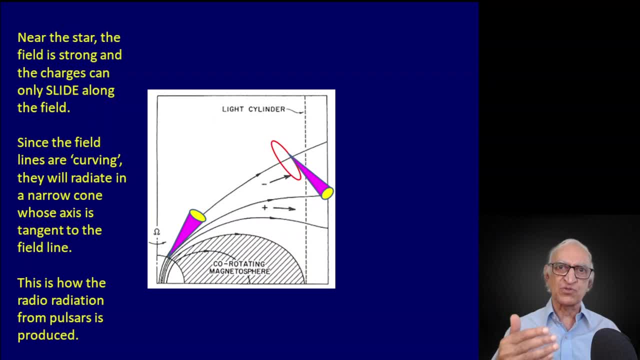 energy. Therefore, the synchrotron photons produced by the electron-positron pairs is not in the gamma ray region of the spectrum, but they are the radio wavelength. But now let us look at what happens to these charges, Electrons as they go near the light cylinder, whose radius is c over omega. 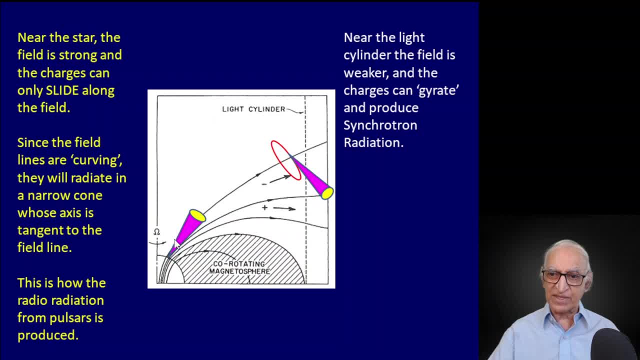 Near the light cylinder the magnetic field is much weaker than near the surface of the star. The magnetic field of the neutron star is roughly a dipole magnetic field and the strength of the dipole magnetic field decreases as 1 over r cubed, where r is the distance from. the center of the star. Therefore, by the time you go to the light cylinder, The magnetic field is not 10 to the power 12 Gauss. It is significantly weaker and therefore electrons can now defy the magnetic field, gyrate around the magnetic field and produce synchrotron radiation from near the light cylinder. 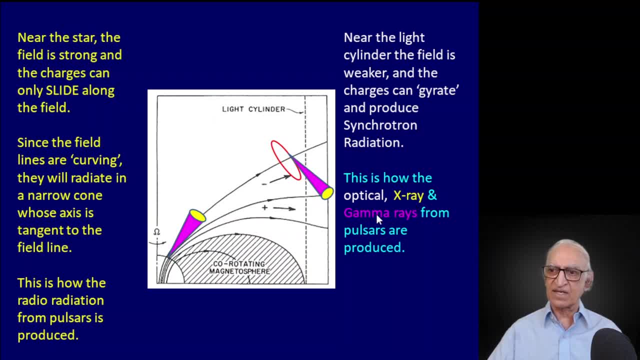 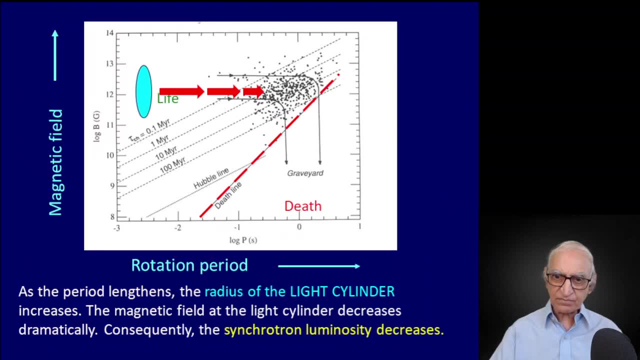 This is how the optical radiation, the X-ray radiation and the gamma rays are produced from pulsars like the Crabbe pulsar or the Wheeler pulsar. But please remember this: As the pulsar ages, its period will lengthen. 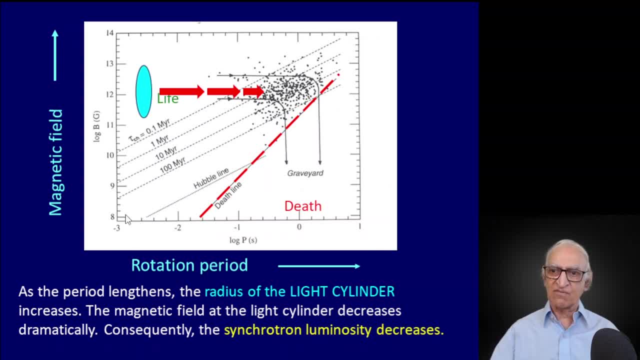 This is the plot of the magnetic field versus the period of rotation. So pulsars are born spinning fast, like the Crabbe pulsar or the Wheeler pulsar, But as they get older their periods lengthen. their omega decreases, their period lengthens. 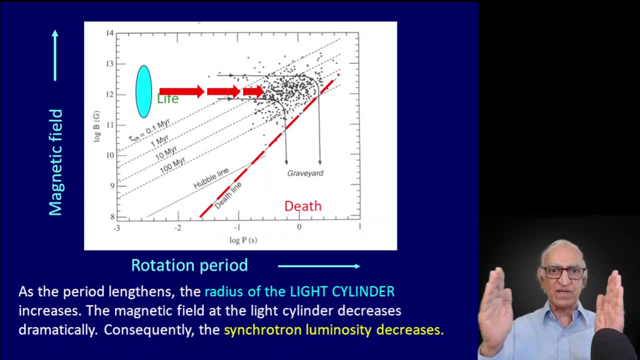 and therefore the radius of the light cylinder, which is c over omega, decreases. Therefore the magnetic field, which decreases as 1 over r cubed, decreases. Therefore in older pulsars the magnetic field near the light cylinder is too weak. 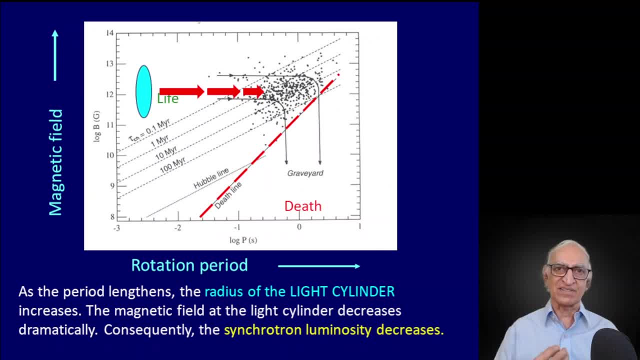 for any significant synchrotron radiation. If you remember, the energy radiated per unit time by a relativistic electron in synchrotron radiation is proportional to b squared gamma squared, where b is the strength of the magnetic field and gamma is the Lorentz factor. 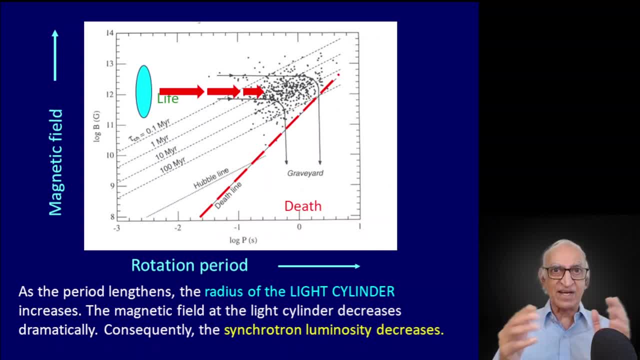 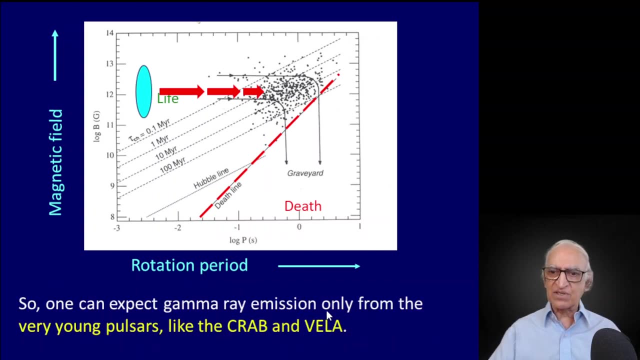 Therefore, as the pulsar ages and the dynamo becomes weaker, gamma ray emission will cease and you will just get radio emission, which is, of course, coming from very close to the surface of the star. Therefore, we can expect gamma ray emission only from very young pulsars, like the Crabbe pulsar. 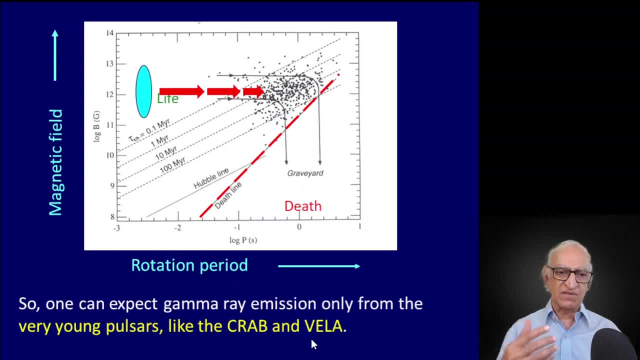 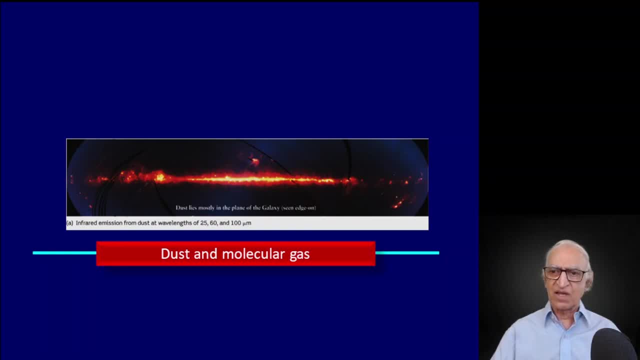 which is 1,000 years old, or the Wheeler pulsar, which is just 10,000 years old. Now let us remind ourselves about the dust and molecular gas around the plane of the galaxy, seen so clearly through their infrared emission. 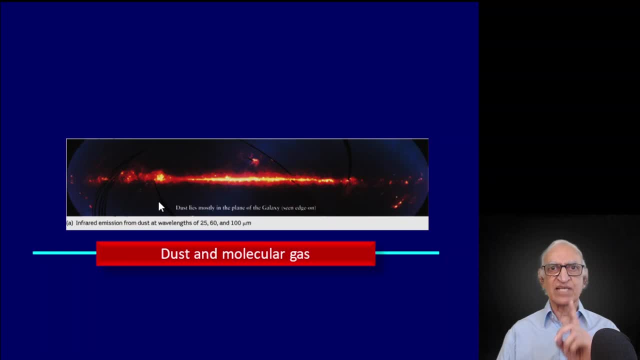 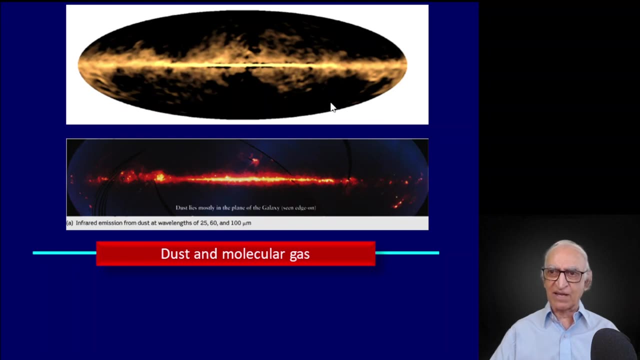 Now let us look at the gamma ray- diffused gamma ray emission from the interstellar medium. This is the picture we saw before And I am showing it again for a particular reason. You notice that if gamma rays are produced by protons interacting with the nuclei of dense gas, 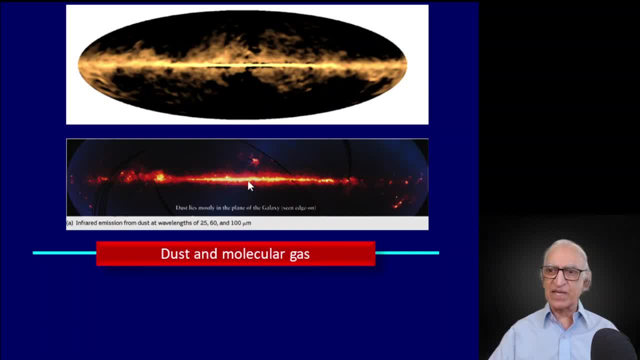 then you would expect the gamma ray emission to mimic the infrared emission. But the gamma ray emission from our galaxy is rather wide in its latitudinal distribution. You see gamma rays from very high north galactic latitudes. You see gamma rays from very high south galactic latitudes. 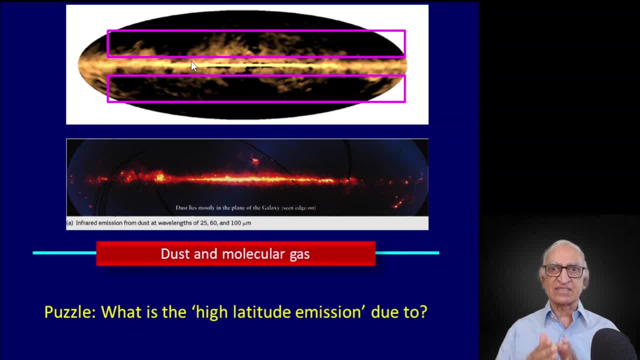 So there is a puzzle. What is this high latitude gamma ray emission which seems to be very diffused in the top magenta box or the bottom magenta box? What is this diffused high latitude galactic gamma ray emission due to? 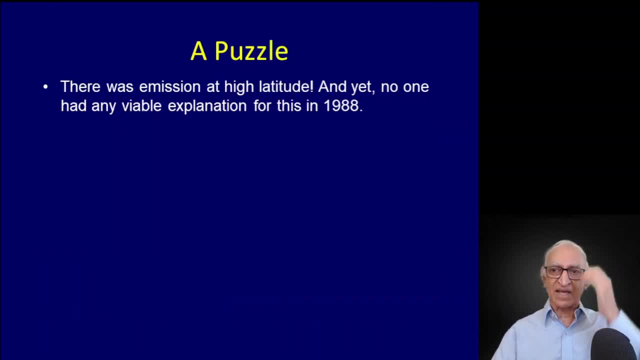 In 1928, when these gamma ray observations were first beginning to come, every gamma ray satellite there was emission already detected at high latitude, And yet no one had any viable explanation, as I just told you, way back in 1988. Besides the interstellar medium, you need dense interstellar medium for protons to interact. That medium isn't there at high latitude because the molecular gas is only 60 parsecs in thickness- half thickness. The only other source of gamma rays are pulsars. 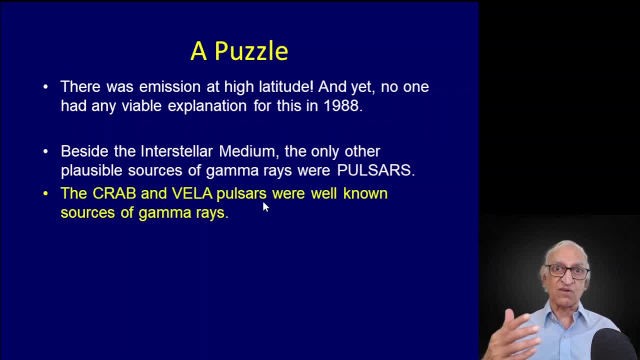 But the urban velar pulsars, of course, are well-known gamma ray sources. So could the high latitude gamma ray emission be really due to young pulsars, which we are not resolving? The answer is no, Because one expects gamma ray emission, as I said, only from young pulsars. because you need the light cylinder to be close to the neutron star so that the magnetic field strength hasn't decreased very dramatically at the light cylinder. But young pulsars will be found near the neutron star, near their birthplaces. Pulsars are born due to the collapse of massive stars. Where are the massive stars to be found? In the plane of the galaxy, where the molecular gas is? Therefore young pulsars like the Kraven velar. you would expect them to be very close to the plane of the galaxy. Therefore, the high latitude galactic emission. 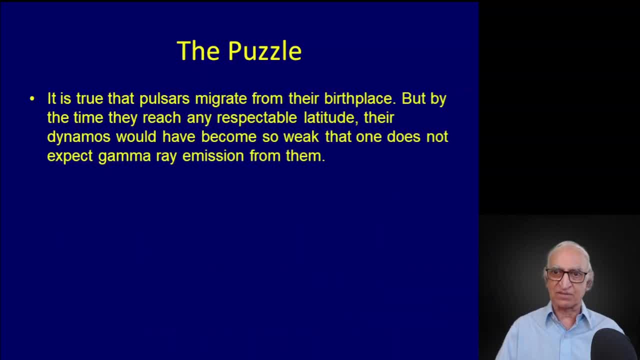 cannot be due to young pulsars like the Kraven velar pulsar. You will say: but look, you told me in the previous lecture that pulsars have very large space velocities, So pulsars may be born near the plane of the galaxy. But they could migrate to very large distances And therefore they could emit gamma rays even though they are at very high latitude. But that won't work Because, yes, it's true that pulsars can migrate, But as they migrate they age. 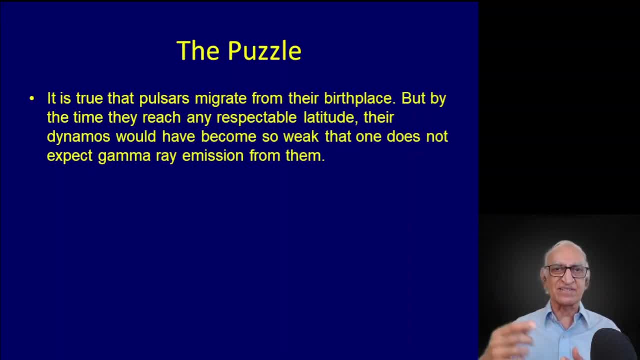 And as they age, their periods lengthen, The dynamo weakens And therefore you would not expect any synchrotron radiation from older pulsars. Therefore, neither the interstellar molecular gas interacting with cosmic ray protons nor young pulsars could be invoked. 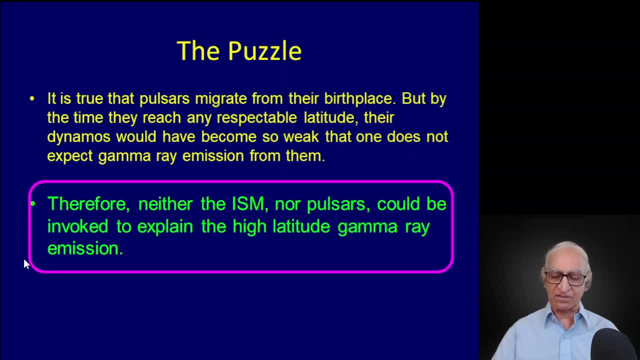 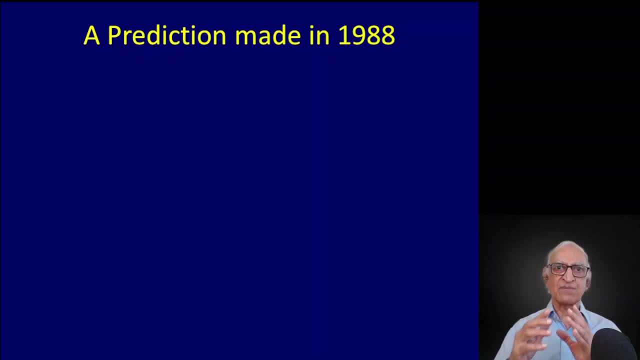 to explain the high latitude gamma ray emission. So this was the puzzle in 1988. When the first NASA gamma ray telescopes were launched, and the galactic emission was first detected In 1988, a long time ago now. 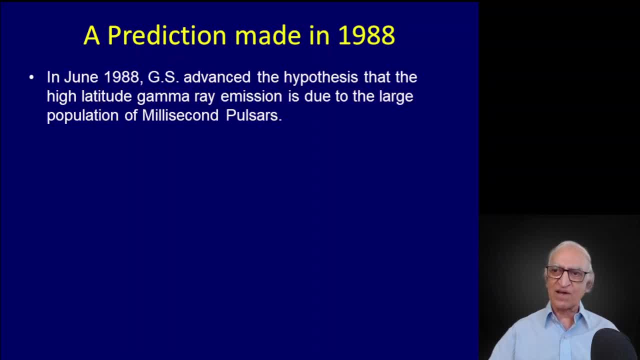 I made a prediction. I advanced the hypothesis that the high latitude gamma ray emission must be due to a large population of millisecond pulsars. Now, millisecond pulsar was first discovered in 1982.. By 1988, only three millisecond pulsars were known. 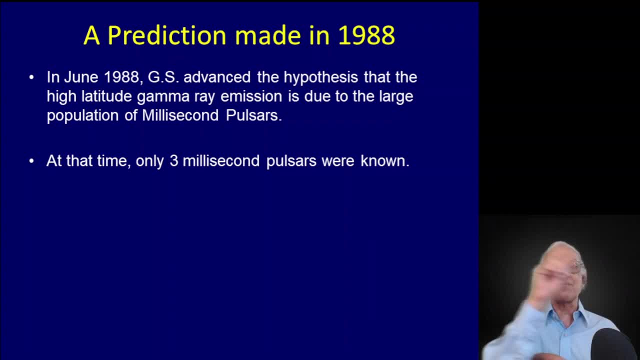 But I was invoking a very large. with three millisecond pulsars you get only three point source emission. So if you want to explain diffuse high latitude emission you need thousands and thousands of millisecond pulsars. Only three millisecond pulsars known. 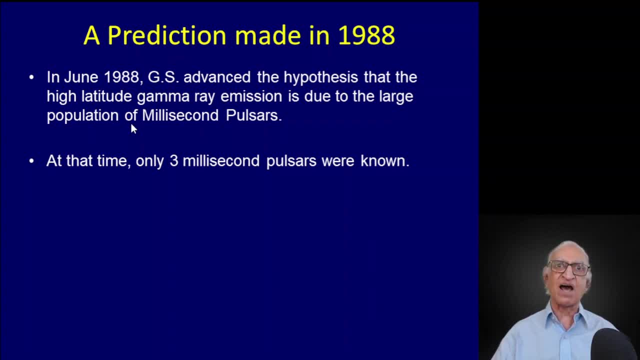 But then I stuck my neck out and said: look, there must be a very large population of millisecond pulsars as yet detected. So I stuck my neck out and the title of my talk was: Millisecond pulsars- a new population of gamma ray sources. 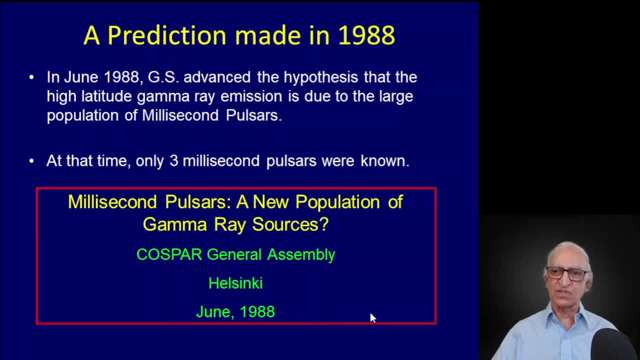 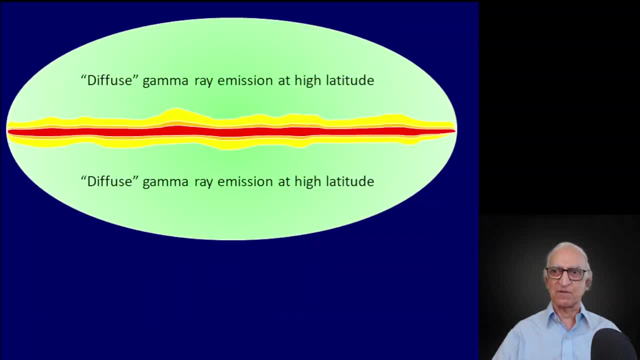 This was at a conference in Finland in June 1988.. What made me make such an atrocious and audacious statement? The idea was simply the following: Yes, you're seeing diffuse gamma ray emission at high latitudes, but this is appearing to you to be diffuse. 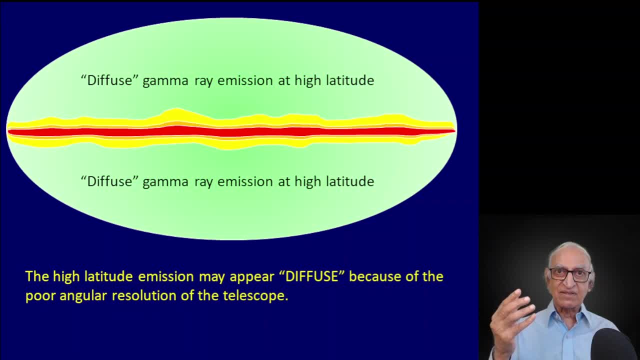 simply because the gamma ray telescopes of that time did not have sufficient angular resolution to detect individual point sources. So if your glasses get fogged because you're wearing a COVID mask, then everything looks very diffuse. But then if you clean the glasses, 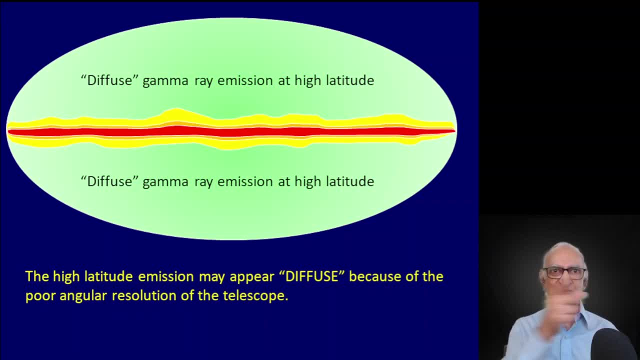 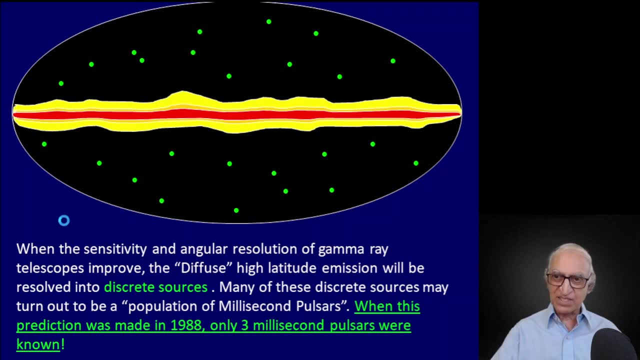 with a piece of cloth and wear it and remove your mask, you'll see individual sources. So that was my crazy idea. So the idea was that this diffuse emission seen by the NASA telescope will someday be resolved into individual point sources and you will then discover. 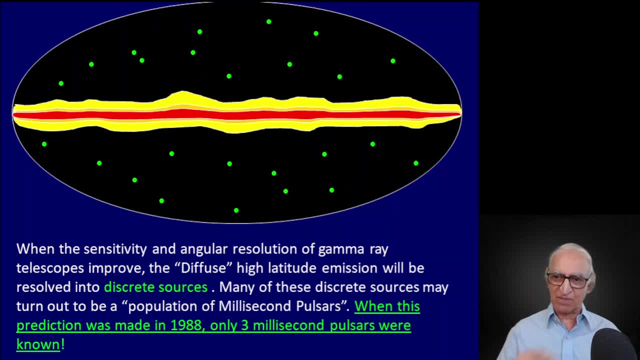 these are, in fact, thousands and thousands of millisecond pulsars. Now, when I said this, of course there was a great deal of skepticism in the audience, because at the time, only three millisecond pulsars were known and I was invoking tens of thousands of millisecond pulsars. Now, why was I doing that? That's because two years earlier, in 1986,, Nipankar Bhattacharya and I wrote a paper in which we predicted that there will be a very large population of millisecond pulsars with a period, with a rotation period. 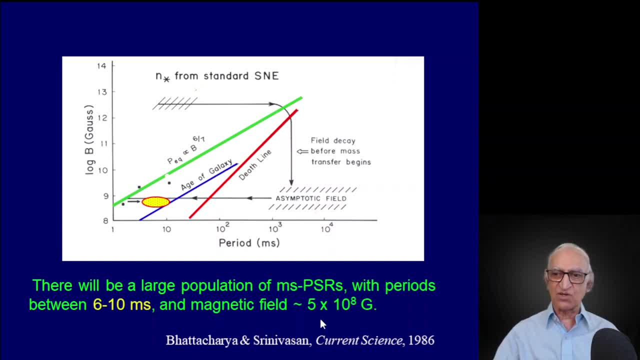 between six and ten millisecond, an extremely low magnetic field of the order of five times ten to the power eight Gauss. Now this is the plot that you might be familiar with. logarithm of the magnetic field of pulsars in the y-axis. 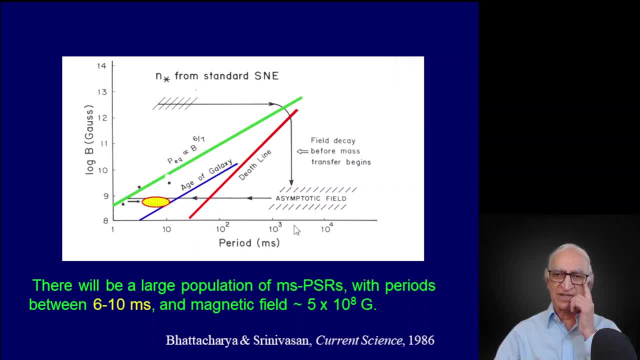 and the logarithm of the period of rotation in the x-axis. Most of the thousand or two thousand pulsars are in this part of the diagram. They have magnetic fields between ten to the power twelve and ten to the power thirteen Gauss. They are in this region. 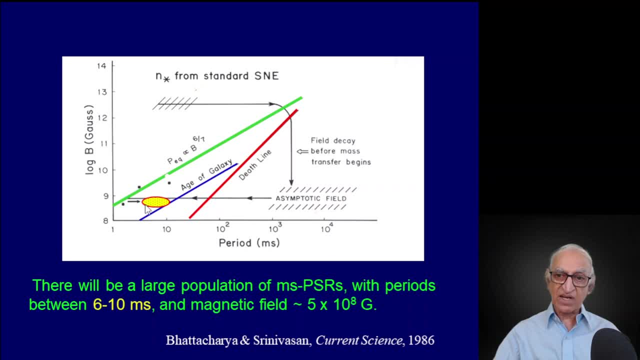 So what we predicted is a very large population of millisecond pulsars in this oval, red oval, and those dot dot dots are the predicted millisecond pulsars which will be detected some day. Now, why won't millisecond pulsars age? 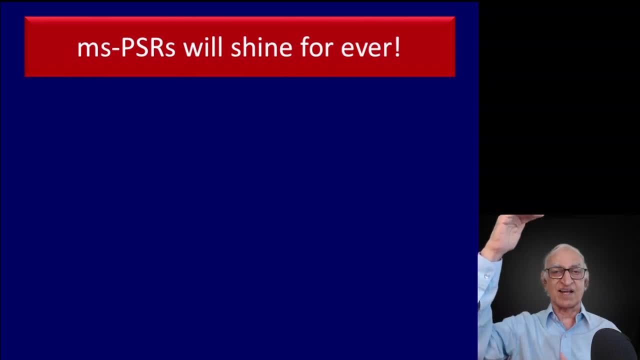 Why will millisecond pulsars be at very large galactic latitude Now? if you remember our discussion of millisecond pulsars several lectures ago, let me repeat it This: millisecond pulsars come from low mass x-ray binaries, The progenitors of millisecond pulsars. 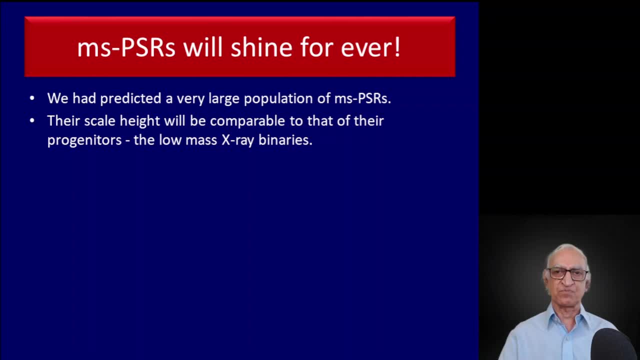 are low mass x-ray binaries and they are spun up. Low mass x-ray binaries have very large scale height. Therefore, you would expect millisecond pulsars to have very large scale height Now, because the millisecond pulsars have extremely low magnetic fields. 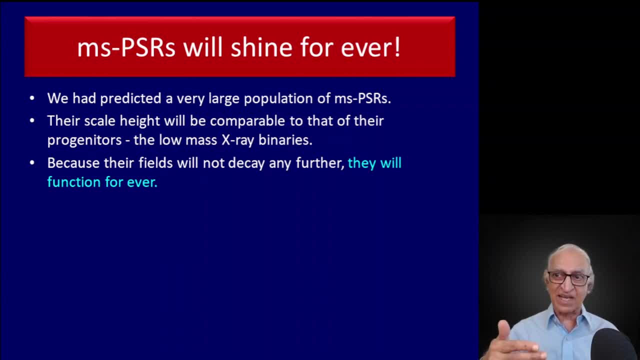 and these magnetic fields do not decay. they will function forever. Why do pulsars die? Pulsars die because their periods lengthen and the dynamo becomes weaker. The period lengthening p dot is inversely proportional to 1 over b squared. 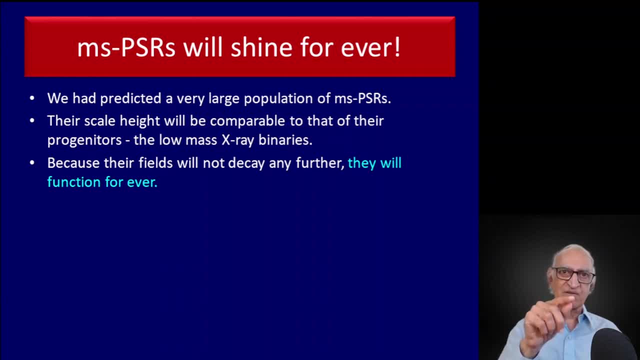 Sorry, p p dot is b squared. The period derivative is proportional to b squared divided by the period. Therefore, larger the period, smaller is p dot And smaller the period, larger is p dot. This is true for normal pulsars. 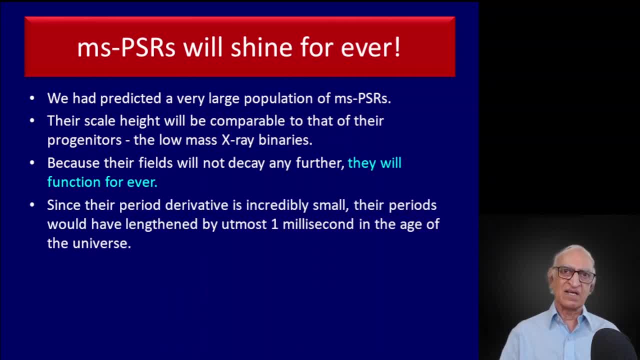 But in the case of millisecond pulsars the magnetic field is not 10 to the power 13 gauss, it is 10 to the power 8 gauss, Five orders of magnitude smaller. Their period derivatives, p dot is not 10 to the power minus 14 seconds per second. 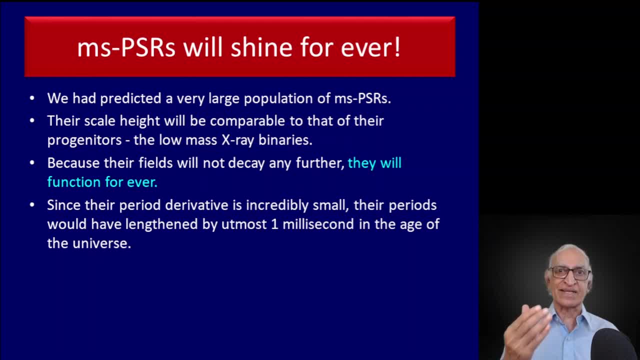 it is 10 to the power minus 21 seconds per second. In other words, a millisecond pulsar in the entire history of the universe. its period will only lengthen by 1 millisecond. Therefore, millisecond pulsars will never age. 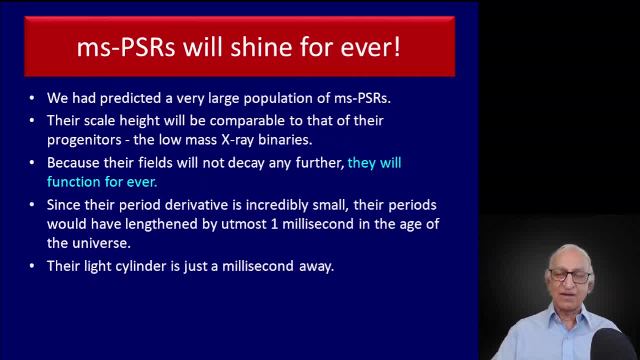 They are youthful forever. Secondly, millisecond pulsars: because they are spinning very fast, the light cylinder will be close by Because, remember, the radius of the light cylinder is c over omega. Therefore the radius of the light cylinder is very large for millisecond pulsars. 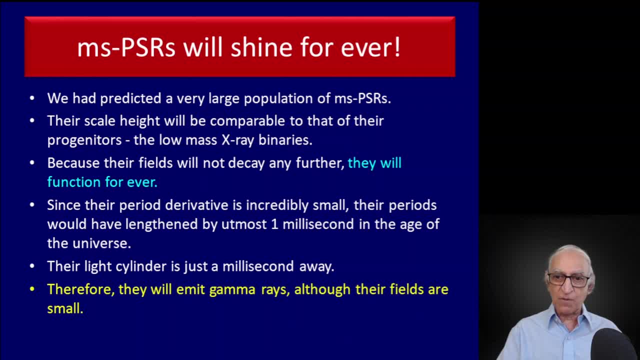 because the period is very short. Therefore light cylinder will be closer. Therefore they will emit gamma rays, although their magnetic field is only 10 to the power, 8 gauss, 1 over r, cube hasn't decayed the magnetic field very much. 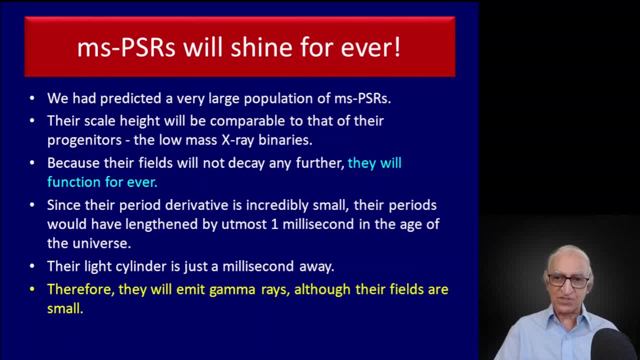 because the light cylinder is very, very close to the pulsar. Therefore, in our paper of 1986, Dipankar Bhattacharya and I had ascertained that millisecond pulsars will live forever. Their lifetime will be the lifetime of the universe itself. 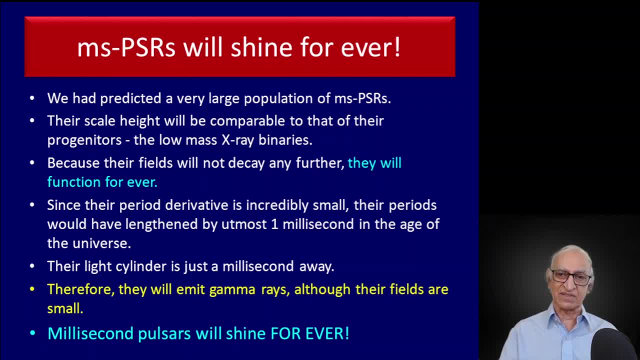 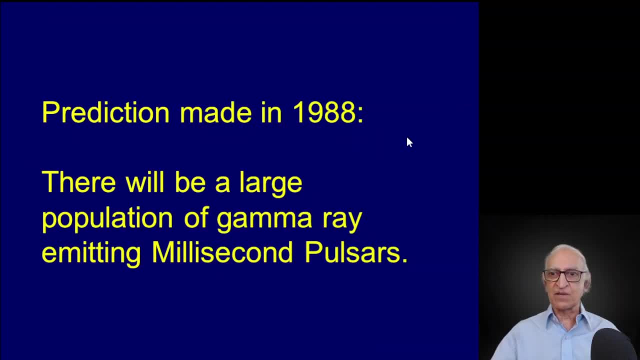 Because their period derivatives are almost vanishingly small And they will have very large scale heights. So that was the basis of my prediction made in 1988.. And the prediction was that the diffuse gamma ray emission at high latitude which couldn't be explained, 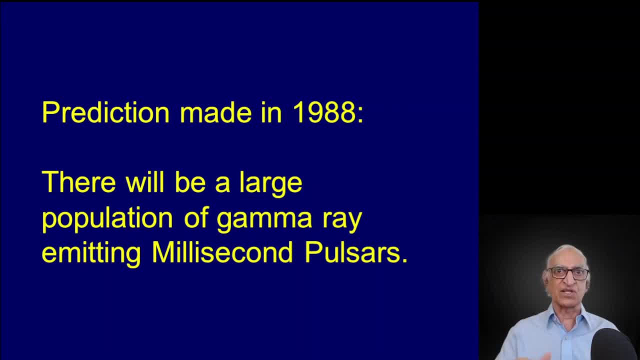 either in terms of young pulsars or in terms of molecular gas interacting with cosmic ray protons, must be due to a very large population of millisecond pulsars which are emitting gamma rays. There were only 3 millisecond pulsars known at that time. 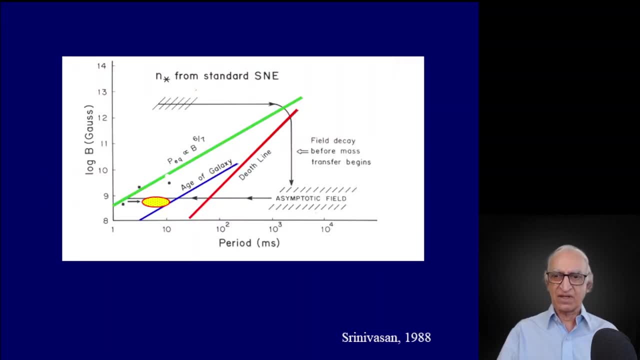 That was the prediction made way back in 1988.. So the prediction was: there must be a large population of millisecond pulsars numbering tens of thousands, if not hundreds of thousands, and they will emit gamma rays and they will be located in this part of the log b, log p period. 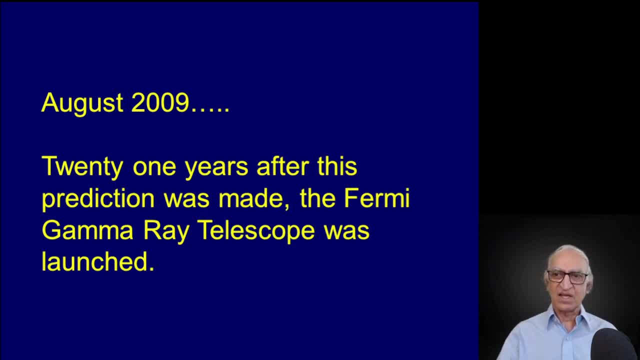 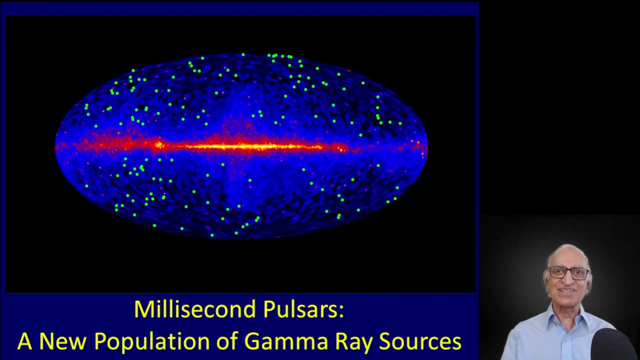 Many years later, in 2009,, 21 years after this prediction was made, Fermi gamma ray telescope was launched, And the first thing that the Fermi Large Area Telescope detected was gamma rays from millisecond pulsars And the discovery paper. 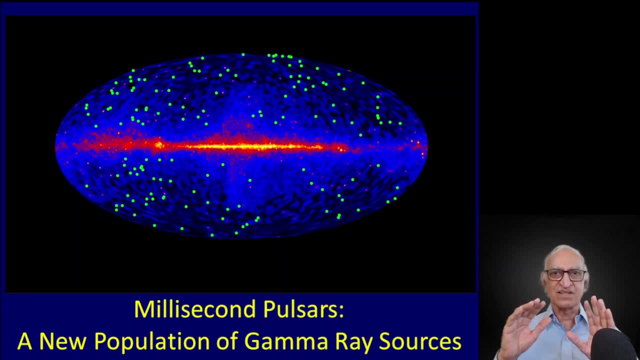 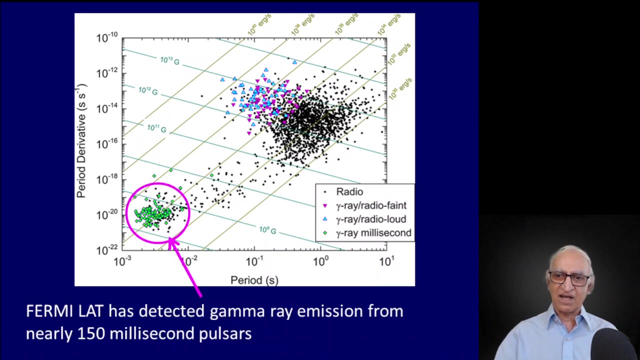 that appeared in the cover of prestigious journal Science. the title of the paper was precisely the title of my paper way back in 1988.. Millisecond pulsars, a new population of gamma ray sources, And what Fermi Large Area Telescope has detected is 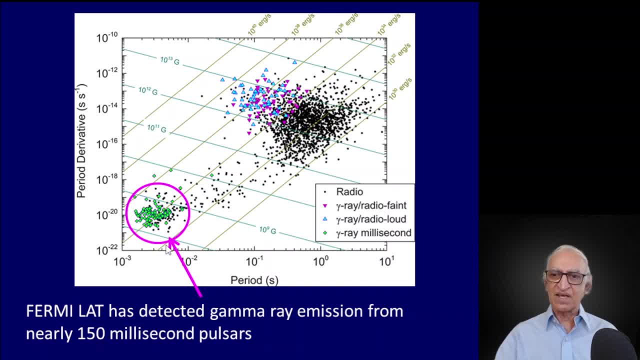 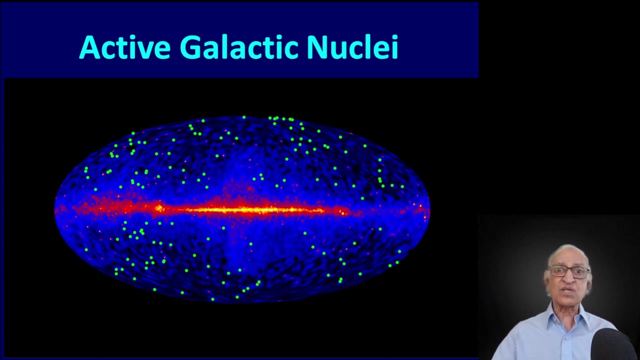 nearly 150 millisecond pulsars in precisely the location that we had predicted way back in 1986.. So the millisecond pulsars are indeed account for the galactic part of the diffuse high latitude gamma ray emission. Now, those aren't the only. 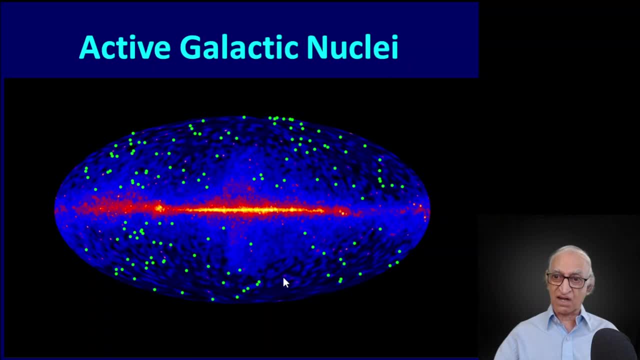 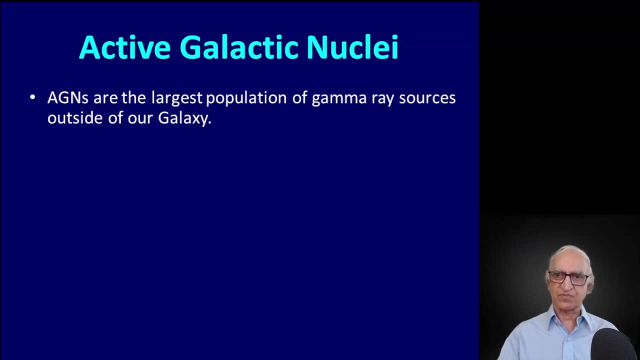 high latitude sources. There are other sources which are not millisecond pulsars. In fact they are the majority. They are the active galactic nuclei. Active galactic nuclei of any description: Seaford galaxies, blazars, quasars. 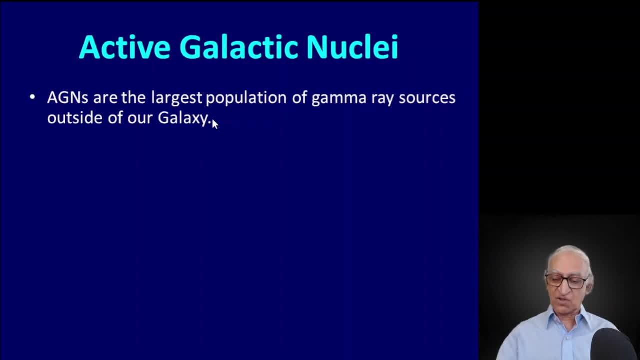 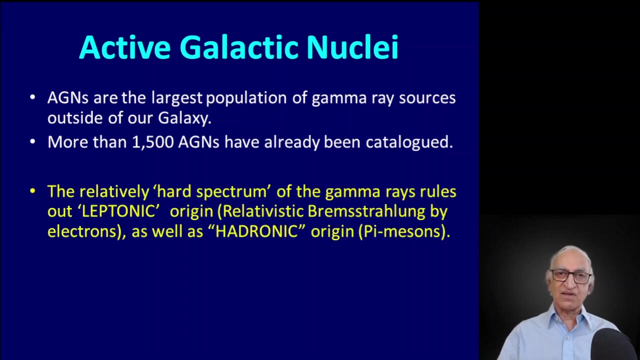 or what have you constitute the largest population of gamma ray sources. More than 1,500 AGNs have already been catalogued based on observations by the Fermi Large Area Telescope. Now the spectrum is very hard. Remember the Fermi Large Area Telescope. 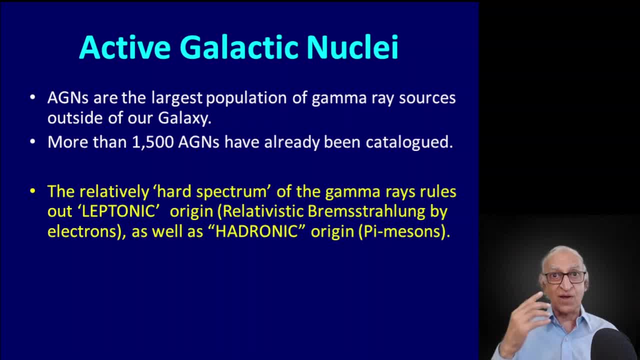 can observe up to 2 TeV, 2 times 10 to the power 12 electron volts. Now this gamma ray emission cannot be leptonic in origin. Leptons are light particles like electrons, So it cannot be thermal brimstone. 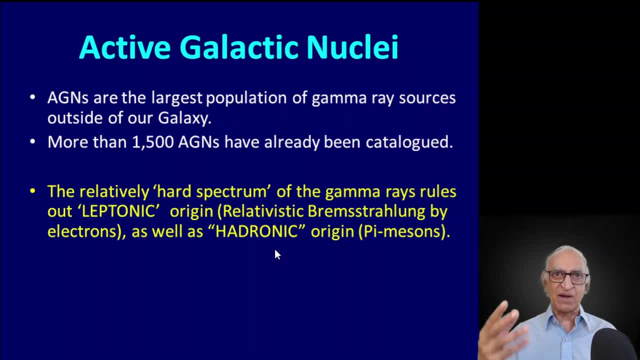 It cannot be hadronic either. heavy particles- Hadrons are heavy particles like the pie mesons. Remember. decay is to 2 gamma rays, But their energy peaks at 70 MeV. Here we are talking of hundreds of GeV. 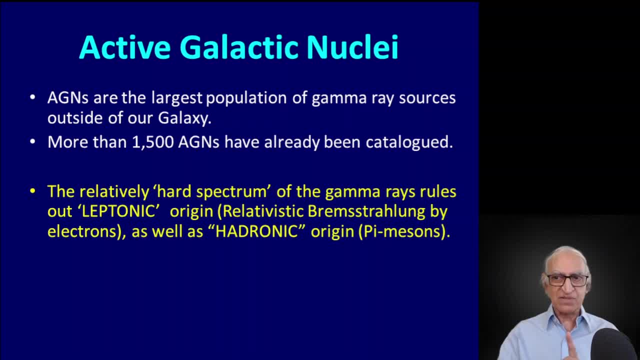 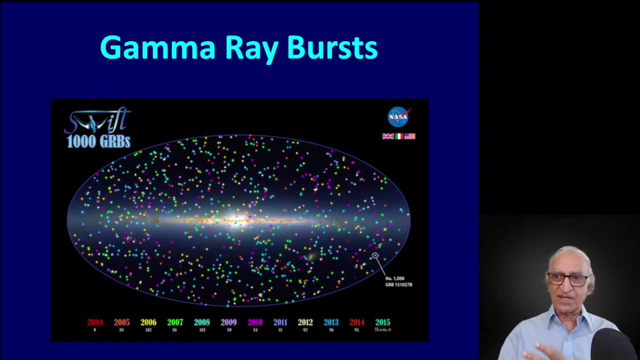 if not 1000 GeV. So it cannot be either leptonic in origin or hadronic in origin. The only other mechanism that is left is inverse quantum scattering. So let us now discuss inverse quantum scattering. Of course, there are also gamma ray bursts. 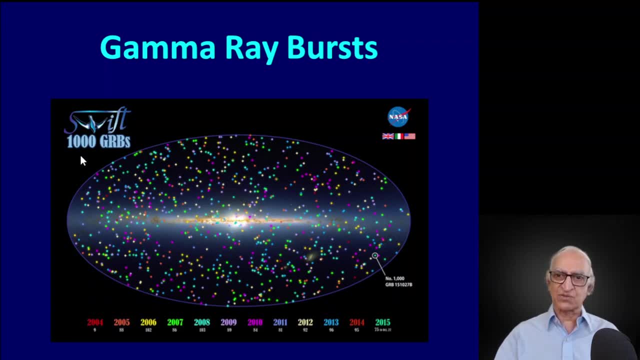 and there are more than 1000 gamma ray bursts that have been detected so far. Their origin is not entirely clear. We know that some of them could be coalescence of 2 neutron stars. because we have detected them, Some of them could be. 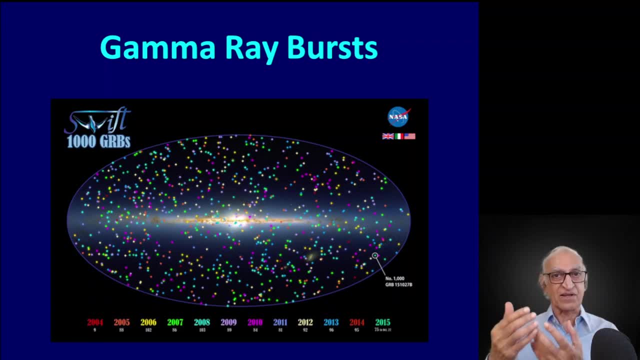 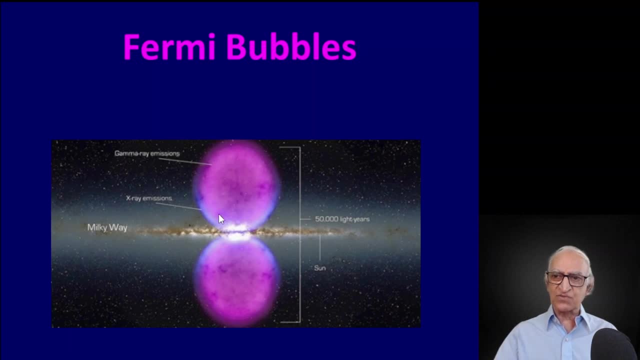 supernovae of a very special type, because we have identified some gamma ray, But there may be other sources of gamma ray bursts also. Then there is this source we saw right at the galactic centre In this picture we are looking straight. 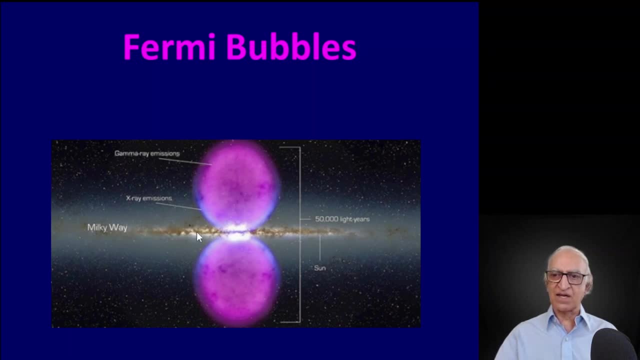 towards the centre of the galaxy And that dark band over there is the dust in our galaxy. That is the plane of the galaxy. Then you see this dipole structure. It is like the radiation pattern of electron, non-relativistic electron. 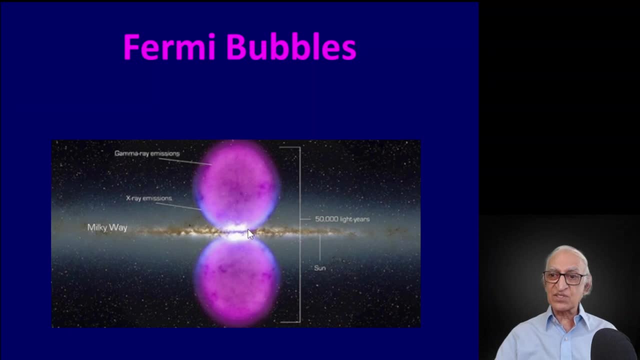 in the dipole approximation, Except this, is enormously large in size. This is 50,000 light years from there to there. 50,000 light years from there to there, Just to remind you the distance from the Sun to the centre of the galaxy. 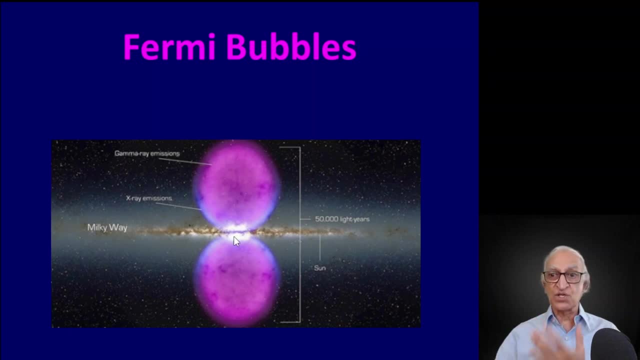 is only 30,000 light years. So these are two enormous structures And what you are seeing? there is gamma ray emission from near the centre of the galaxy. These are now termed as the Fermi bubbles- Fermi because they were detected. 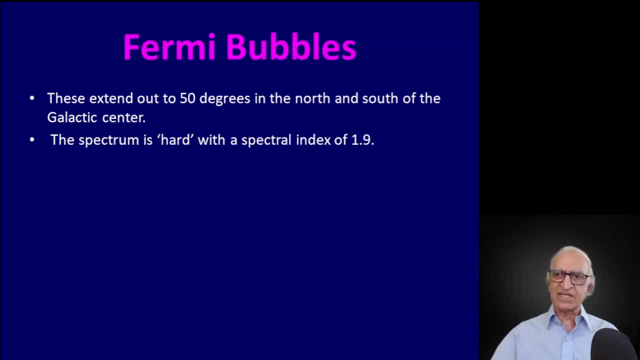 by the Fermi Large Area Telescope. They extend to 50 degrees above and below the plane of the galaxy. The spectrum is very hard. The spectrum index is 1.9.. Intensity versus frequency: the slope is 1.9.. 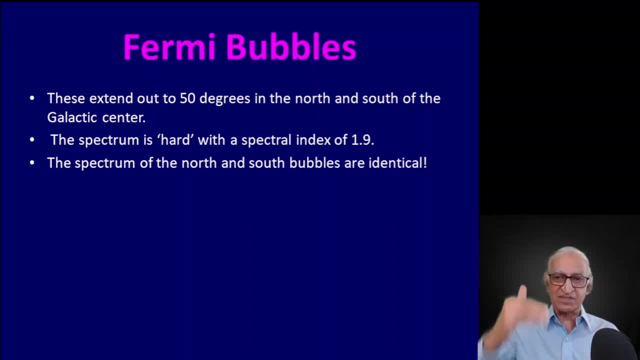 The spectrum of the northern part of the bubble and the southern part of the bubble are identical, So whatever is the mechanism producing these bubbles, they are identical. It is located at a distance of 10,000 parsecs, or 30,000 light years. 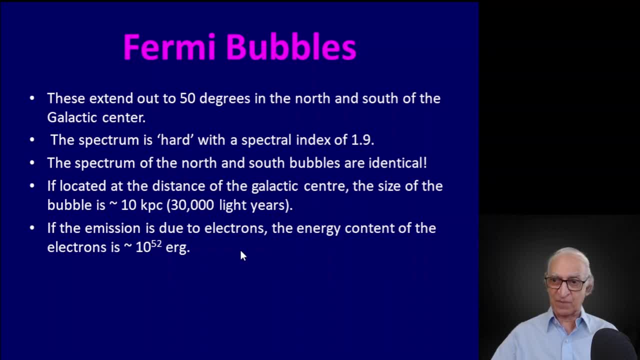 And if the emission is due to electrons, which is suspect, then the energy content of the electrons must be as large as 10 to the power 52x, which is enormous: 10 to the power 52x, The most likely mechanism. 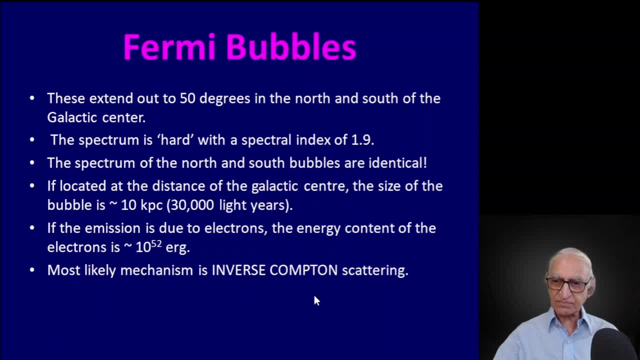 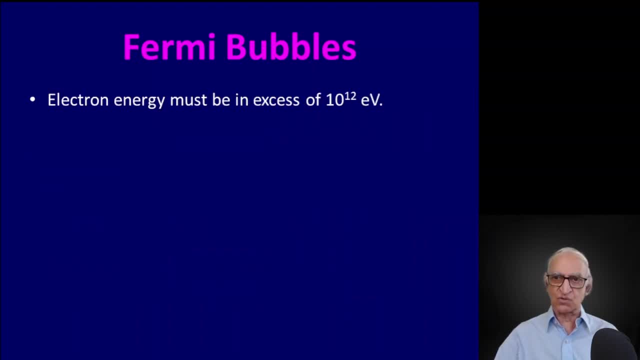 is inverse content. scattering Electrons must have an energy in excess of 10 to the power, 12 electron volts. But these electrons, by the time they travel 50,000 light years above and below, will cool because the energy is lost in radiation. 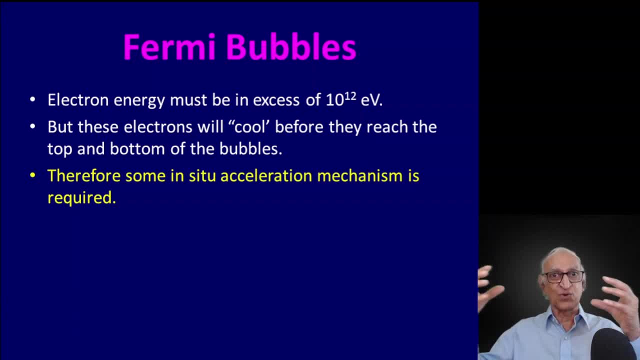 Therefore, just like in radio galaxies, we had the two lobes at a distance of billions of parsecs, millions of light years, The electrons would have lost energy, so they had to be in-situ acceleration, Similarly here, to irradiate this bubble. 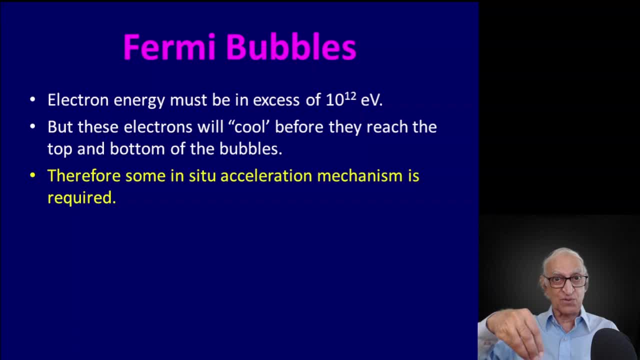 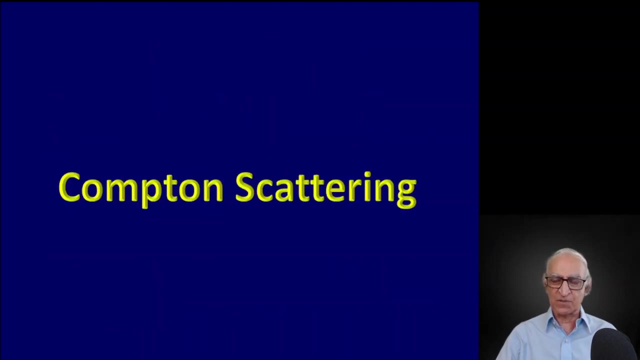 the electrons must not only be produced by the central source, presumably the central black hole. Black hole is the center of a galaxy, but these electrons must be accelerated continually. We don't know what this mechanism is, So let's leave the speculations for a moment. 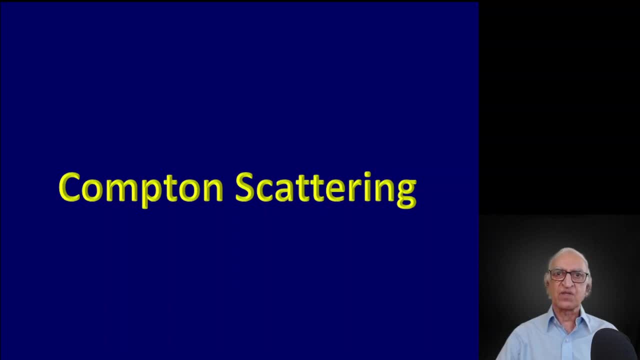 And so, in the remaining time, let us discuss Compton scattering. Now, if you remember, in 1928, Compton discovered an important effect for which, in 1928, he was awarded the Nobel Prize for Physics. Let us first remind ourselves of Thomson scattering. 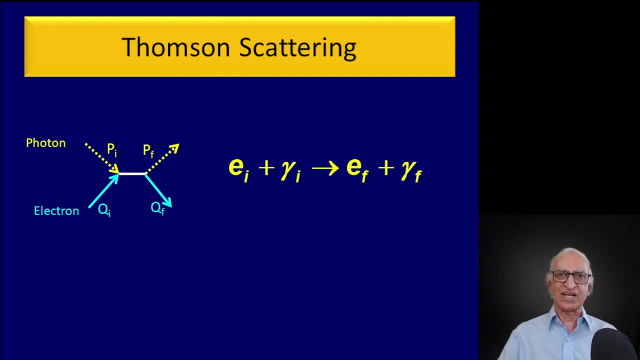 first discussed by the great JJ Thomson, who discovered the electron in the Cavendish laboratory. We discuss Thomson scattering when we discuss the sun and the stars. An electron scatters off a photon. Electron collides with a photon and what you have coming out. 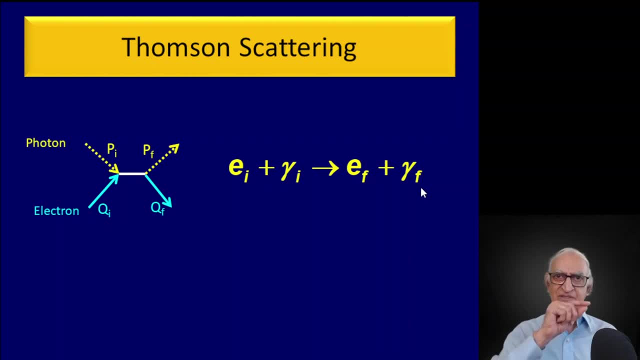 is an electron and a photon. What really happens is that if you have an electron which is more or less stationary, the oscillating electric field of the incoming radiation will make the electron oscillate at the same frequency and oscillating electron will radiate at the same frequency. 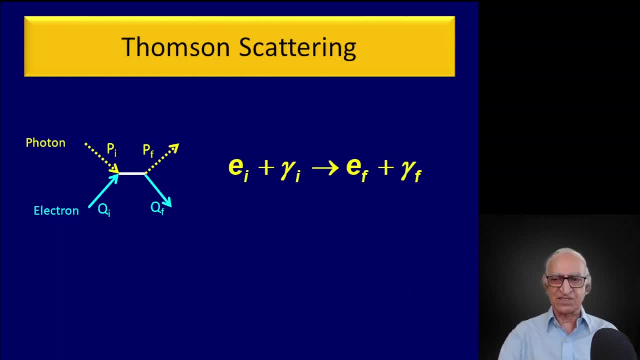 and that's what Thomson scattering is. We discuss this at great length Now. in Thomson scattering we assume that the energy of the photon remains unchanged, namely the incident energy of the photon gamma i is the same as the photon scattering of the final energy. 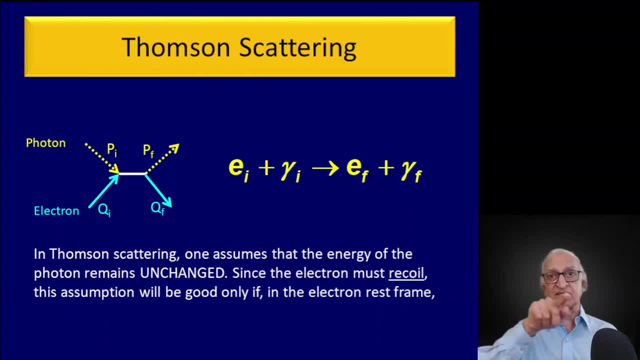 gamma f. Now, when a photon scatters off an electron, the electron is bound to recoil, and that recoil energy must surely come at the expense of the energy of the photon. Therefore, the photon scattering can be rigorously elastic, or the photon will not lose. 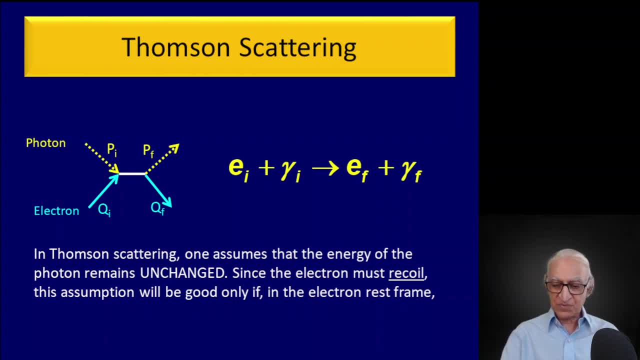 any energy at all in the scattering, only if in the rest frame of the electron the photon has a very low energy. But as I have said many, many times, low or high energy in physics has no meaning. you have to compare it with something. 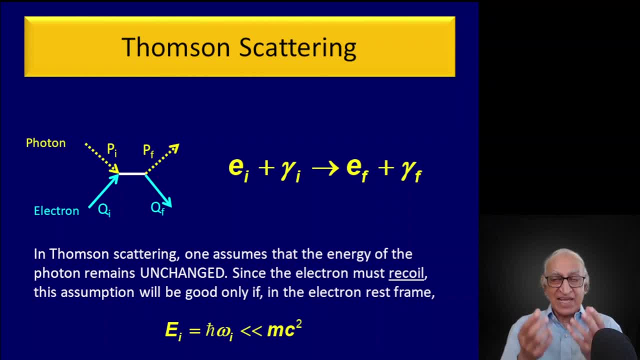 How much energy does a stationary electron have, m, c squared, where m is the rest mass of the electron. So as long as the energy of the photon, h bar omega, is much less than the rest mass energy of the electron, the electron will not recoil much. 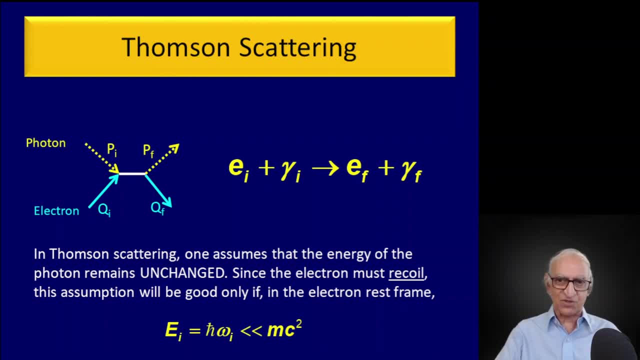 when the photon bounces off the electron. So that is the regime of Thomson, scattering The incident. photon must have an energy which is very small compared to the rest mass energy of the electron. In this case we are talking about stationary electron, more or less stationary electron. 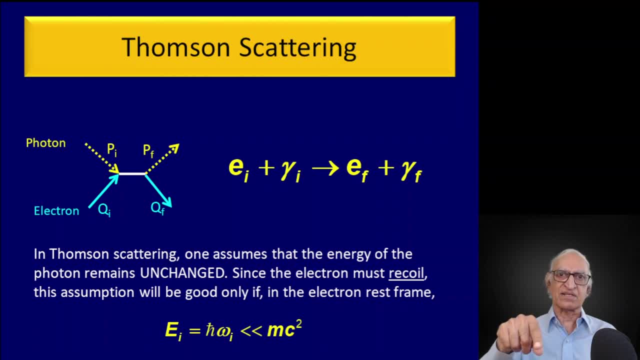 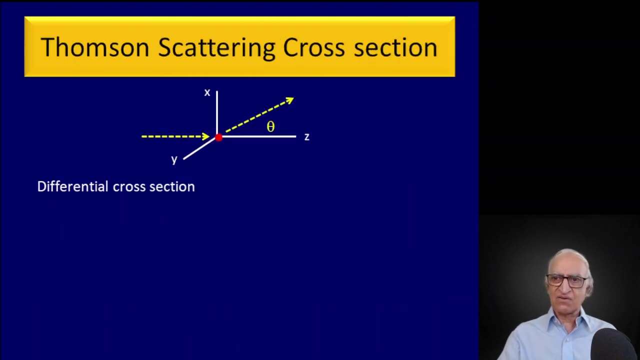 because what Compton did was to scatter x-rays of electrons and metals. Electrons and metals are moving at relatively low velocities. They are not relativistic electrons. Now the differential cross section for Thomson scattering. let us skip all the mathematics. we have discussed this several times before. 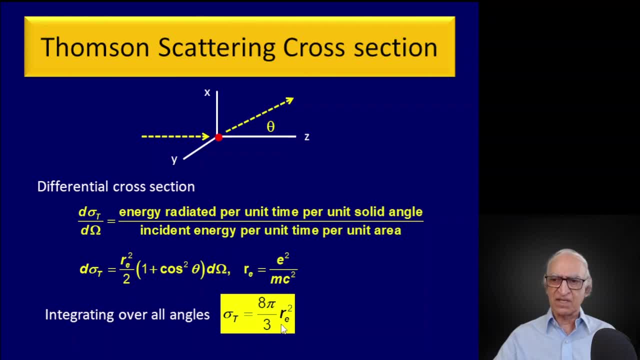 The Thomson scattering cross section is 8 pi by 3, square of the classical electron radius. The classical electron radius is e squared over mc squared. The value of the Thomson scattering cross section is 6.65 into 10 to the power, minus 29 meters squared. 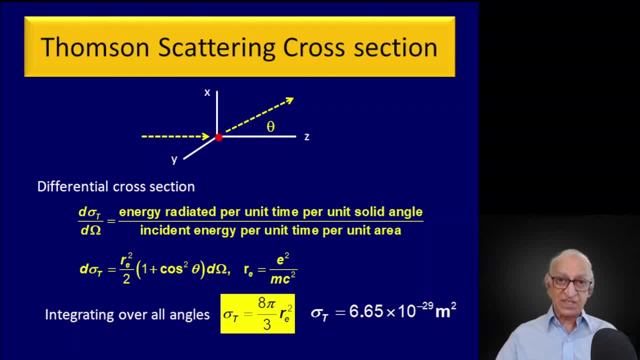 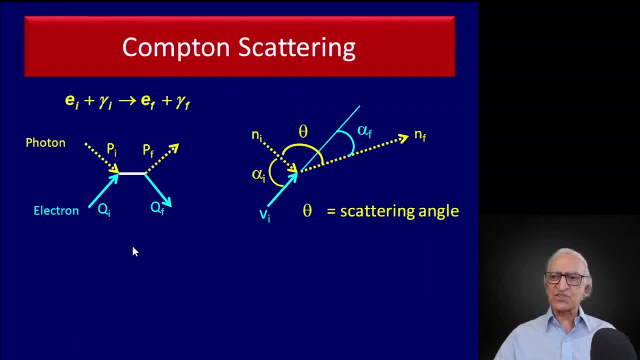 Cross section is the dimension of an area. This leads to a mean free path in the sun of half a centimeter. This is the mean free path in the sun of half a centimeter. Now let us discuss Compton scattering. It is the same scattering. 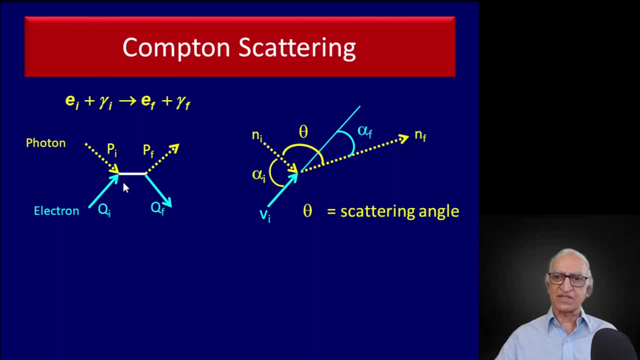 There is an incident electron and an incident photon and there is a final photon trajectory and a final electron trajectory. Pi is the initial momentum of the photon. Qf is the final momentum of the photon. Qi is the initial momentum of the electron. Qf is the final momentum. 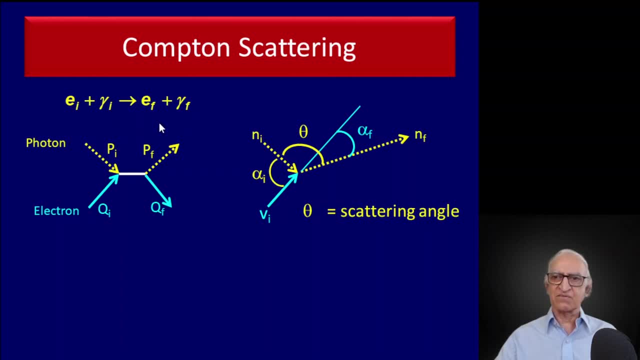 of the photon And this is the scattering we are discussing Now. the geometric representation of the scattering is shown on the right. This is the incident electron, This is the incident photon, And the angle between the incident photon and the incident electron is alpha i. 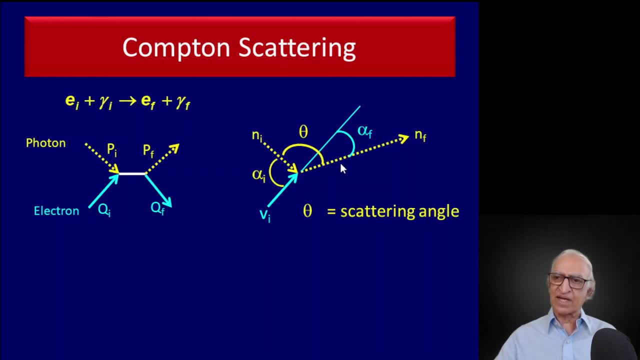 The photon is scattered and goes in that direction. The angle of scattering between the initial direction of the photon and the final direction is theta, And the electron goes in that direction. This angle is alpha f, So theta is the angle by which the incident photon. 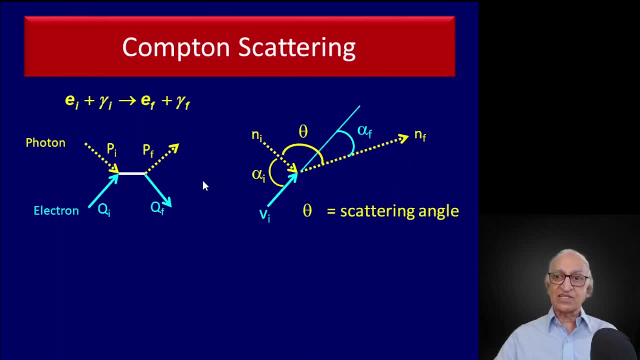 is scattered. Now the difference between Thomson scattering and Compton scattering is: we will now be discussing the case where the electron is relativistic. Now, Ei is the initial energy of the electron, Ef is the final energy of the photon. Gamma i is the initial energy. 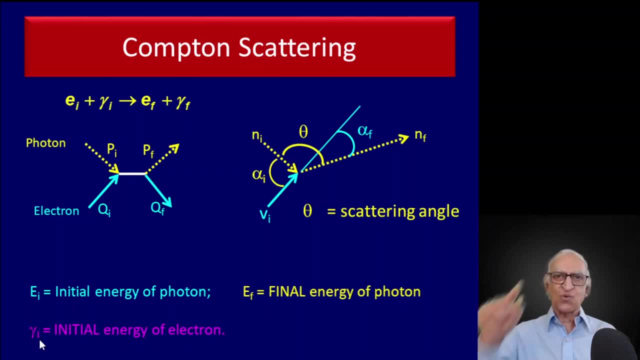 of the photon Gamma i is 1 over square root of 1 minus Vi squared divided by c. squared Vi is the incident velocity. So it is a very simple problem You have on the left hand side of the reaction. you have a momentum. 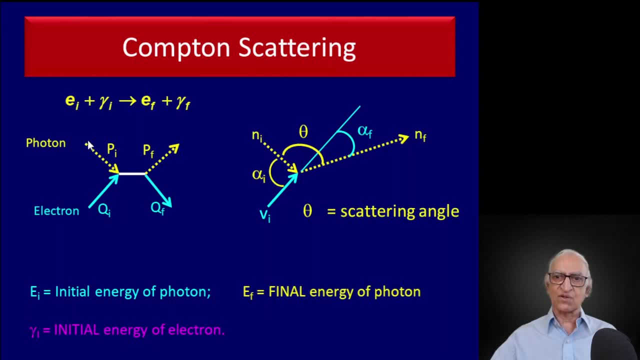 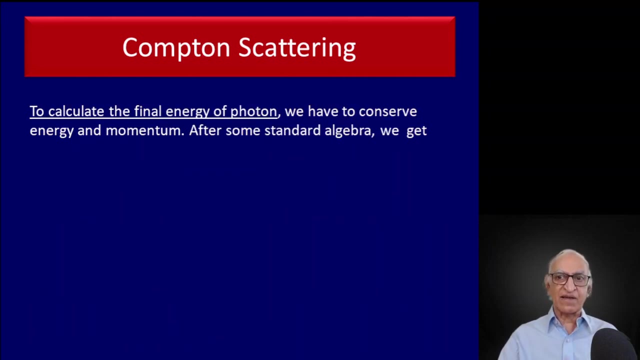 of the electron momentum, of the photon energy, of the electron energy of the photon. On the right hand side you have the photon and the electron. Both energy and momentum have to be satisfied simultaneously. Therefore, to calculate the energy Ei, the sum of the energy, 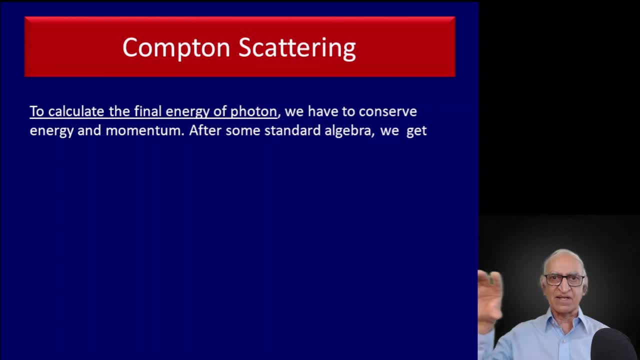 of the photon and the electron must be equal to the final energy of the electron and the photon, and similarly for the momentum. Now this is a very simple, straightforward high school calculation. You should be able to do it in about 5 minutes time. I shall not take the time. 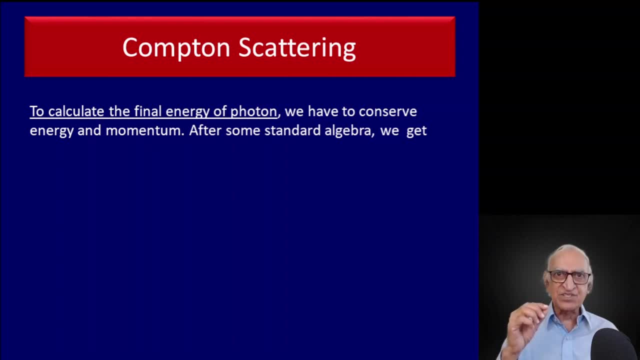 to do this algebra for you. I suggest you do it yourself. This is a very elementary calculation: Adding up the momentum on the left hand side, right hand side, adding up the energy on the left hand side and right hand side and equating the two. 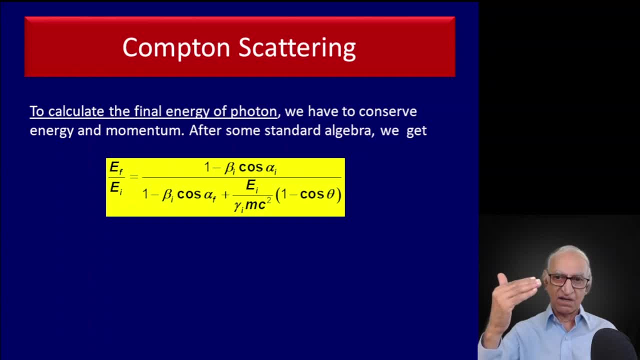 When you do that, please take it from me. This is what you get: Ef divided by Ei, where Ef is the final energy of the electron. I showed you what these various angles are in the previous diagram, So we will not bother about that. 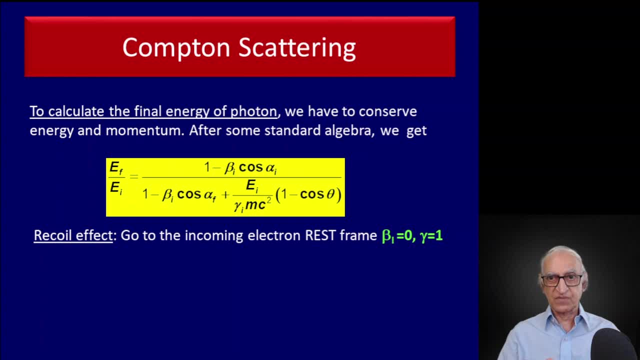 Now we are talking about a relativistic electron. How to make this calculation simple, A trick that we have done before. Let us jump on to the relativistic electron. In that frame, the electron is at rest. Beta, which is V over C, is 0.. 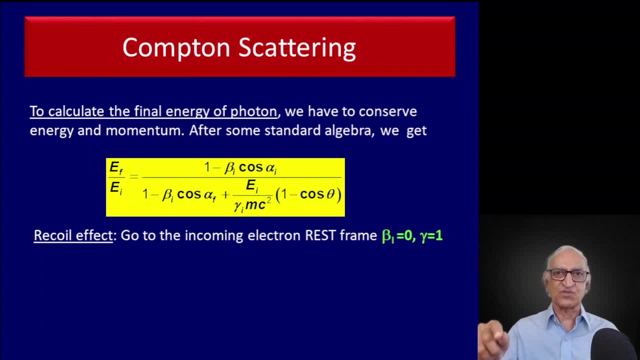 Gamma, which is 1 over square root of 1 minus V square by C square, is 1.. Because the electron is stationary. So in that case, in this formula, in that frame of reference, I put Beta equal to 0 and Gamma is equal to 1.. 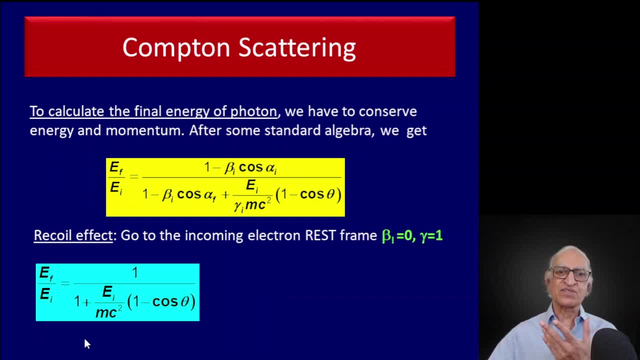 The formula reduces to a very simple formula which you would have studied in your BSC physics: In the rest frame of the electron. So the final energy of the photon, divided by the initial energy of the photon, is given by this expression over there. 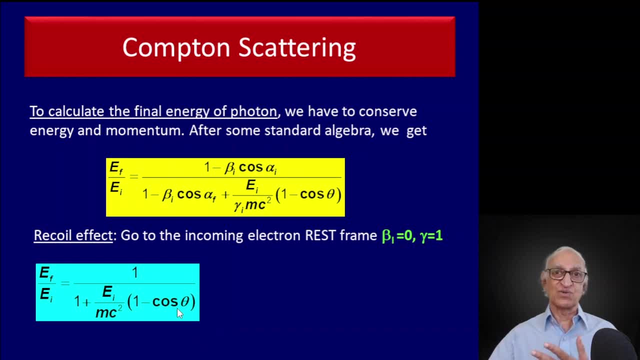 Now, cos theta is a value always equal to or less than 1.. And this is a positive number. Therefore, it is always 1 plus some positive number. Therefore, denominator is greater than the numerator. What this tells you is that the numerator on the left hand side 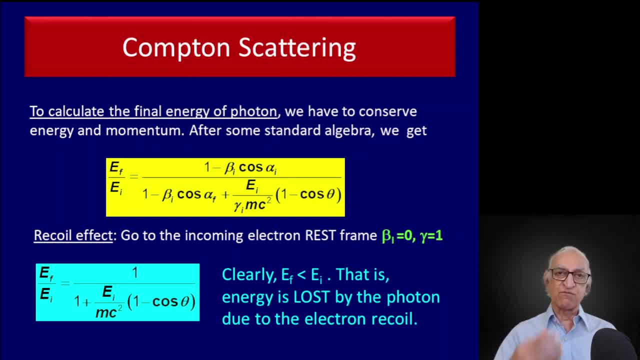 is clearly less than the denominator on the left hand side. In other words, the photon has lost some energy. Where did that energy go? In the recoil of the electron. When the electron gets a kick, it has a certain kinetic energy- half mv square- and that has come at the expense. 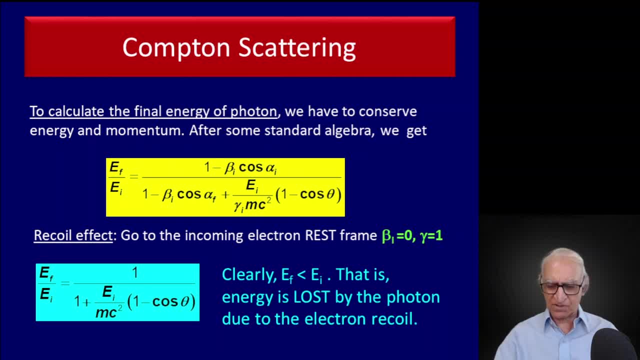 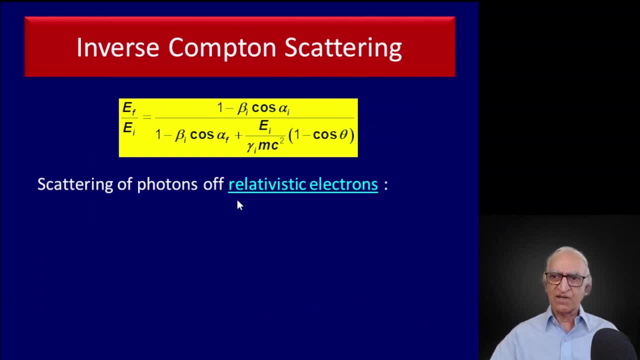 of the photon energy. This is content scattering. Now let us look at the formula again. Now we want to discuss the case of relativistic electrons. When we are talking of relativistic electrons, beta, which is v over c, is approaching 1.. Gamma, which is 1 over square root of. 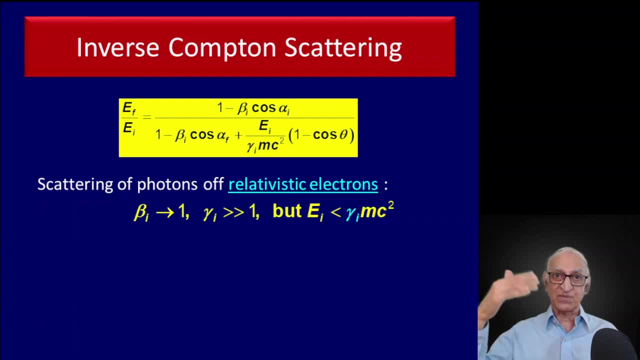 1 minus v square by c square is a very large number. It can be 100, 1000 or even a million, But let us assume that an incident photon, whatever it might be, has an energy less than the rest mass energy of the electron. 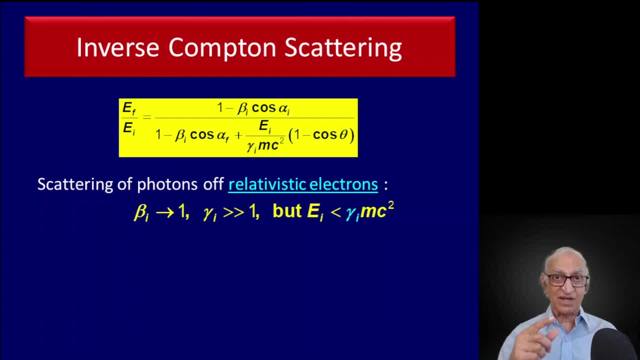 What is the rest mass energy of the electron mc square? Where m is not the rest mass energy, It is m0 divided by square root of 1 minus v square by c square. Einstein taught us that in 1905.. In other words, 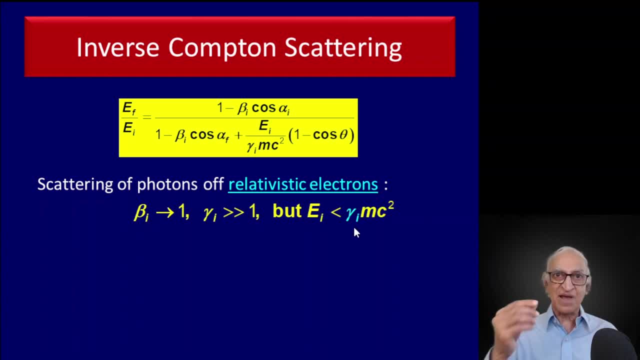 the energy of the rest mass energy of a relativistic electron is gamma mc square, where m is now the rest mass. it is mc square, but m is now not the rest mass energy that you find in, but it is really gamma m. Gamma is 1 over square root of. 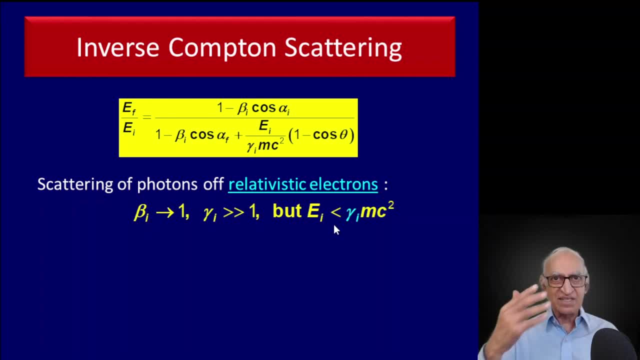 1 minus v square by c square. So we are going to assume that this condition is satisfied. Now, in this case, we will see that this formula will predict that the photon can gain an enormous amount of energy, In other words, the final energy of the photon. 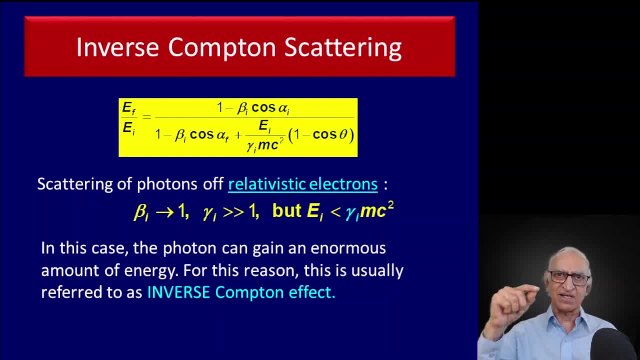 can be thousands or million times more than the initial energy of the photon. It comes from the same formula from which we derived the Compton's formula by jumping onto an electron going to its stationary frame. But this is the formula in the laboratory frame, not in the electron rest frame. 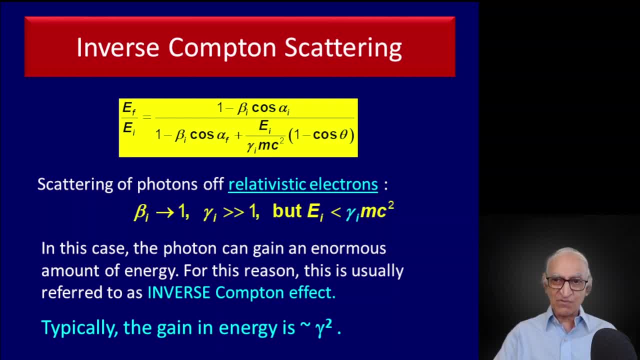 Now what we will find- and I will make this argument possible in the next couple of minutes- is that typically, when a relativistic electron collides with a photon, the photon will gain energy by a factor of the order of gamma square, Where gamma is 1 over square root of. 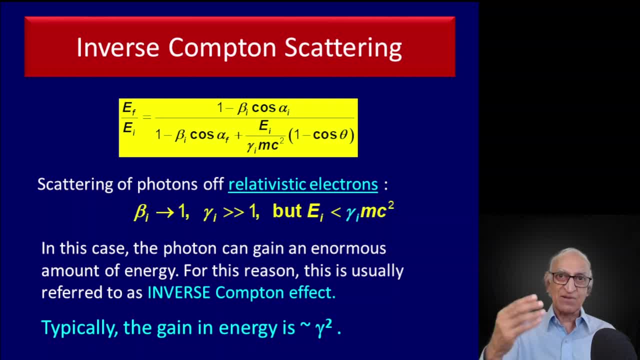 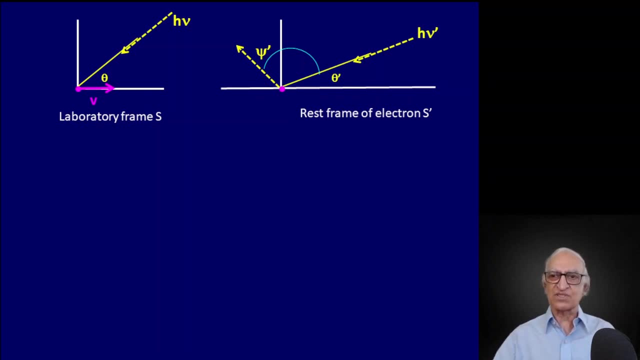 1 minus v square by c square. Therefore, gamma square is 1 over 1 minus v square by c square, which can be an enormous number. It can be a million or a billion. So let us convince ourselves that you will in fact gain an enormous amount of energy. 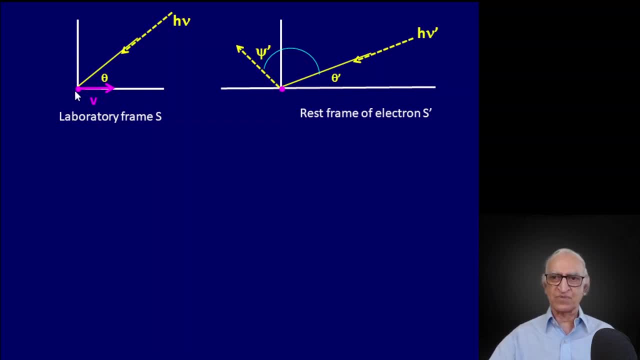 The scattering we are talking about is the following: An electron is moving, let us say, along the x axis with a relativistic speed and a photon is approaching it at an angle theta. This is the diagram of the collision in the laboratory frame which I have named as S. 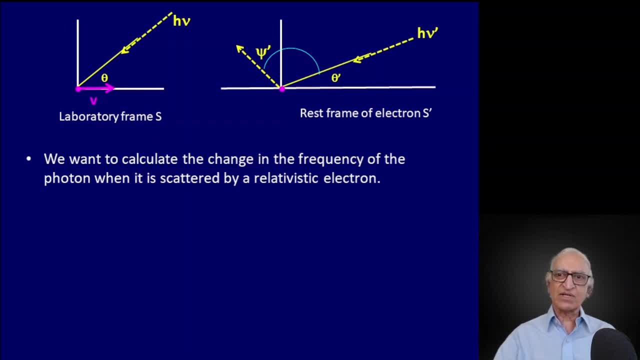 Now let us do a simple trick. We want to calculate the change in the energy of this photon when it scatters off this relativistic electron. Now this calculation can be done. We have the full formula, Which I have shown you three times already. 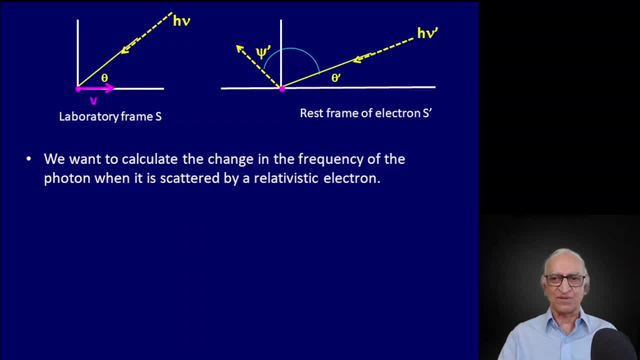 But I am trying to do a poor man's estimate of how much energy will be gained Now. in order to make a poor man's estimate, let us do a trick. Let us jump onto this relativistic electron And go to this frame S prime. 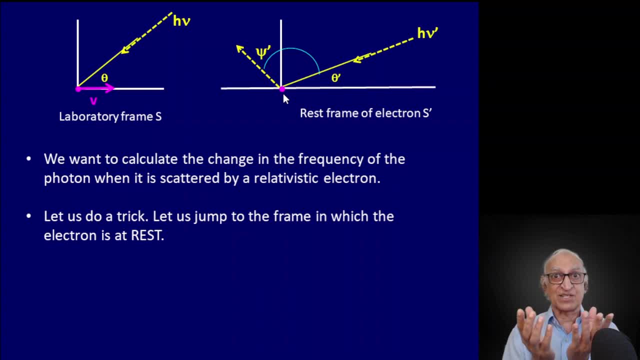 So in that frame I have jumped onto the electron. Therefore the electron is at rest with respect to me, because I am co-riding with the electron. Now, in that frame S prime the photon is coming not at this angle theta, but at angle theta prime. 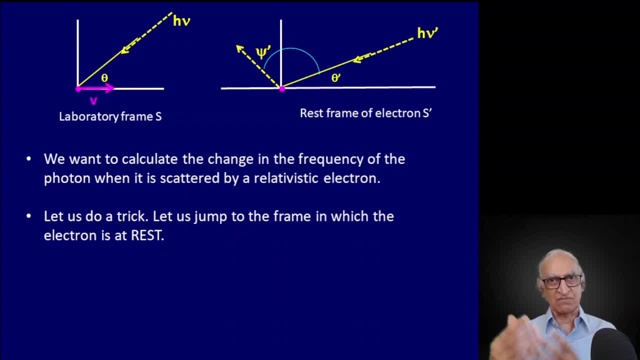 The angle may be the same or may not be the same. You have to see for Lorentz transformation. Now, the important thing to appreciate is that you notice that this incoming photon- I have not labelled it the frequency nu, I have called it as nu prime. Why? 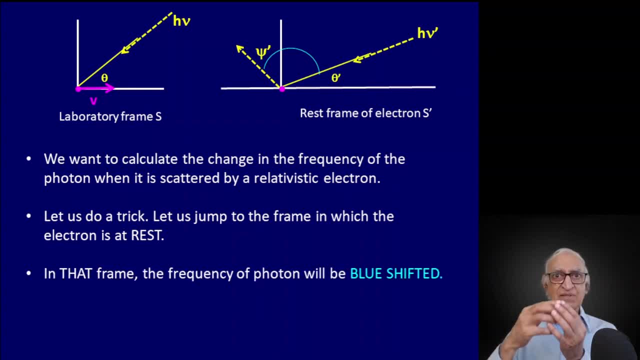 That is because if I am in the rest frame of the electron, the photon is approaching me, I will see the frequency of the photon Doppler shifted towards the bluer part of the spectrum. In other words, the photon frequency will be blue shifted. Remember, if the photon is moving away, 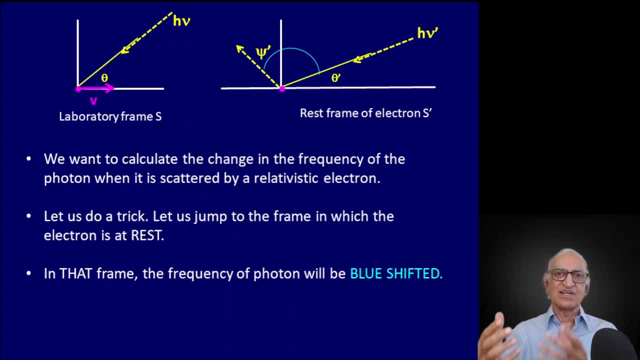 it will be red shifted. If the photon is moving towards you, its frequency will appear to be blue shifted or the frequency will increase, And that is, of course, given by a formula which I derived for you in our lecture on special relativity. When I am sitting, 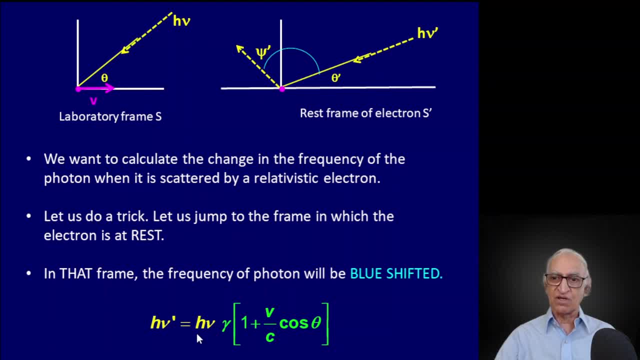 on the electron. the frequency of this photon, which is nu in the laboratory frame, will appear to me to be nu prime, and the two are related by Doppler's formula: gamma times 1 plus v, cos, theta. Now, if the electron is moving very slowly- velocity, 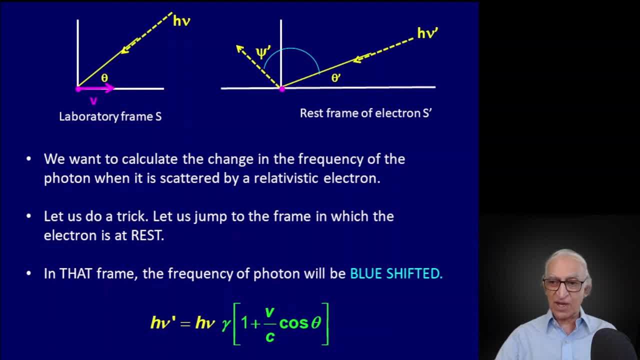 is very small compared to the speed of light. gamma is 1 and I have only 1 plus v cos theta, which is our good old Doppler shift formula. This is also the Doppler shift formula, but it is that special relativistic Doppler shift formula which I 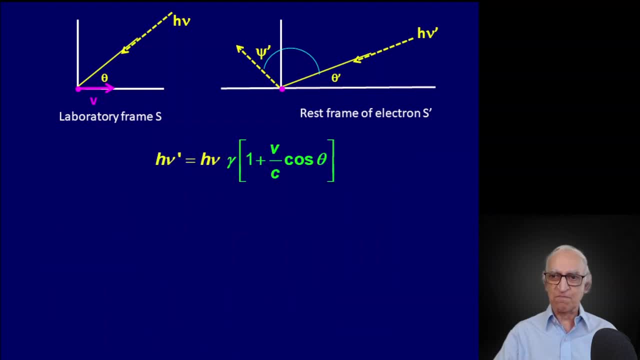 derived for you and used also. So in the frame in which the electron is at rest, the relativistic electron is at rest. that is the frequency of the approaching photon. Now the approaching photon will be scattered. It will be scattered to a new direction, scattered by an angle. 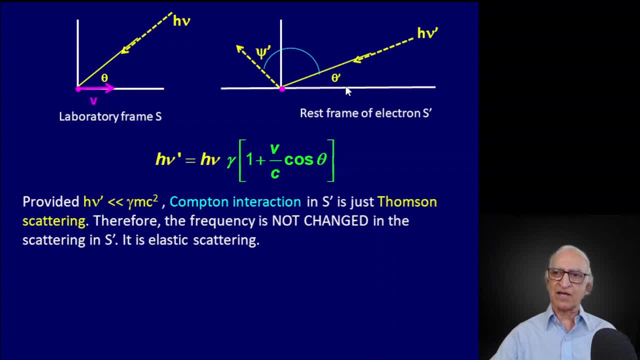 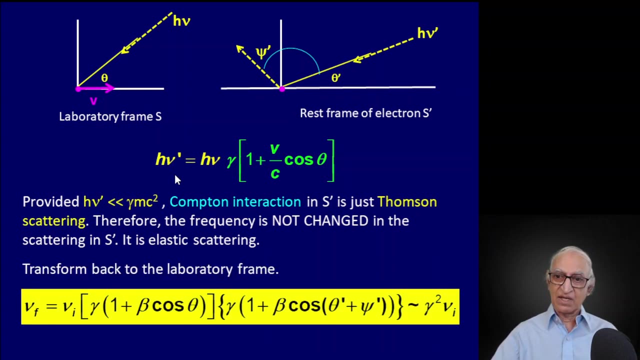 psi prime in the frame s prime, so photon is scattered by that angle. Will its frequency change? Well, its frequency will not change if as long as, sorry, as long as this frequency h nu prime given by this formula, as long as it is still less than. 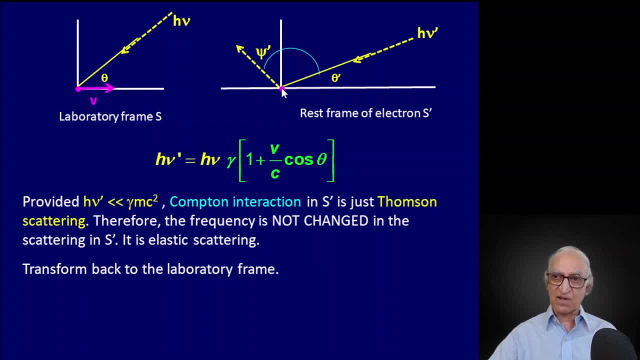 gamma m c square, where gamma is the Lorentz factor of the electron in the laboratory frame. As long as h nu prime is much less than gamma m c square, I can regard this scattering in the frame s prime as Thompson scattering, in which the frequency of the photon is not changed. 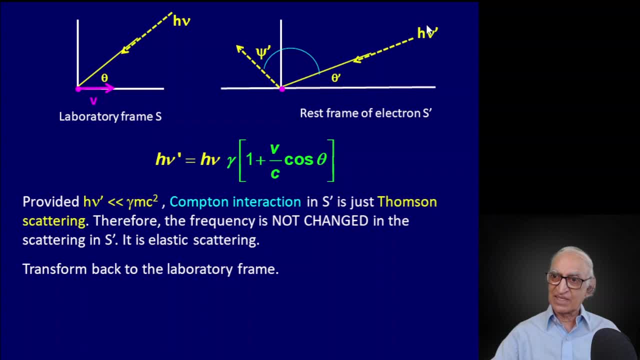 at all. So this photon in this frame has a frequency nu prime, and this photon in this frame has again frequency nu prime. So what I am interested is the frequency in this frame, laboratory frame s prime. So I jump off the electron onto the laboratory. 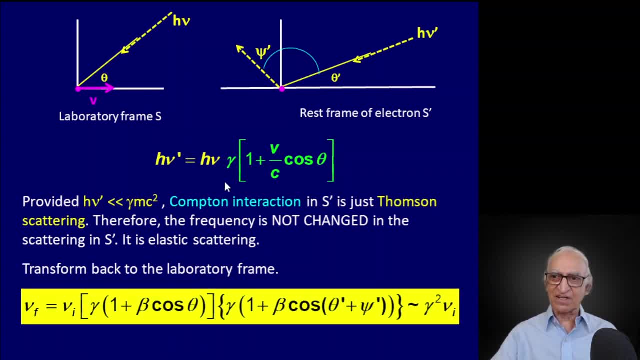 and what I will get is another factor of Doppler shift, namely I had h nu prime- h cancels out nu prime, which is nu i- into gamma, 1 plus beta, cos theta, which is just this formula there, and then again I will have a gamma into 1 plus beta. 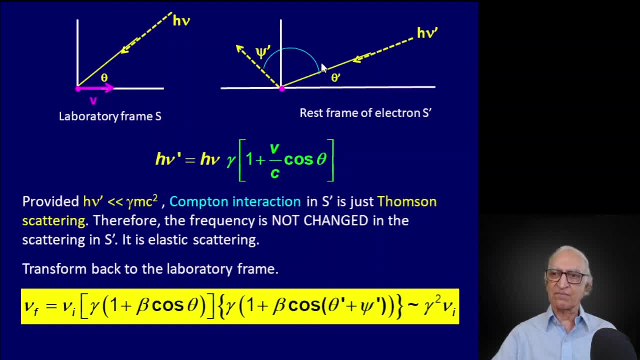 cos of this angle, which is theta prime plus psi prime, so it is elastic scattering. so all I have done is now, calculated by some simple trick, a poor man's derivation of the frequency of the scattered photon in the laboratory frame. we didn't want to do this. if you are. 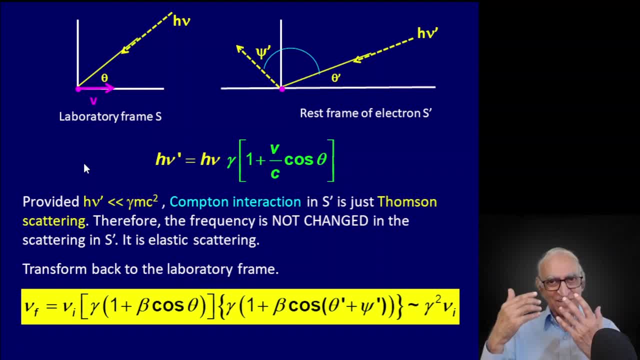 uncomfortable doing this, go to the original formula and convince yourself. the result is there. I am just trying to make it possible for you. so now you will see that the frequency, final frequency of the photon will be approximately gamma square times the initial frequency, provided these angles are all suitable. 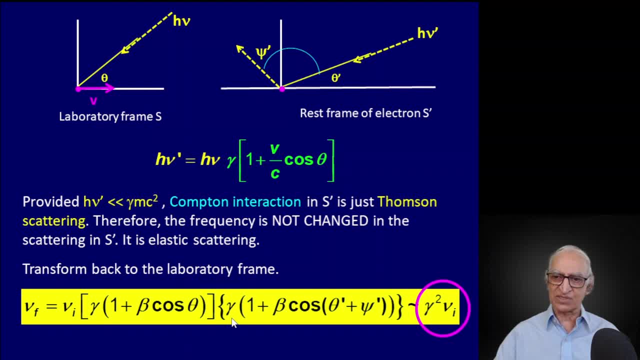 so there is a gamma here and there is a gamma over there. so please convince yourself that in the most favorable situation, which is head on collision between the electron and the photon, the frequency of the photon will be increased by a factor. gamma square so in the laboratory frame. 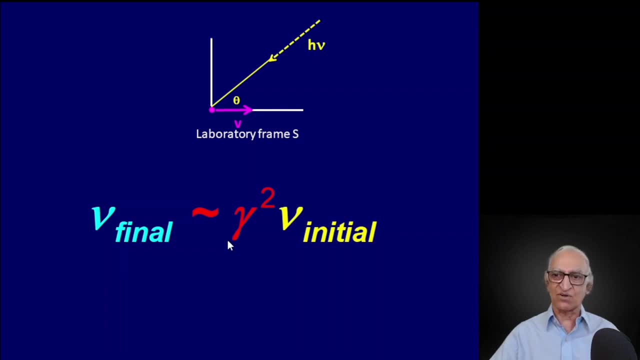 where a photon scatters off a relativistic electron whose energy is gamma mc squared the frequency of the final photon. the scattered photon will be gamma square times the frequency of the initial photon. this is the energy gain in Compton scattering. now this inverse Compton scattering. 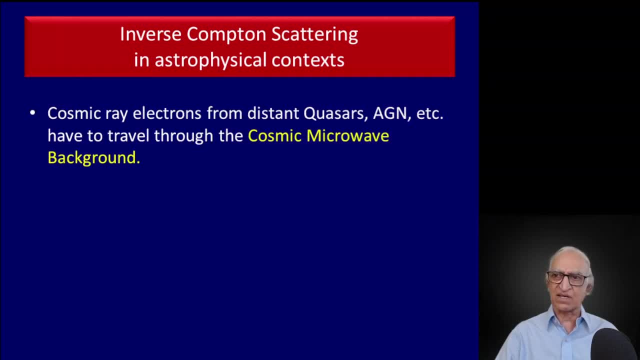 is extremely important in many astrophysical consequences. for example, cosmic rays, which I talked about many times, are produced by quasars and active galactic nuclei, which are billions and billions of light years away. so are the cosmic rays that we observe on earth coming from? 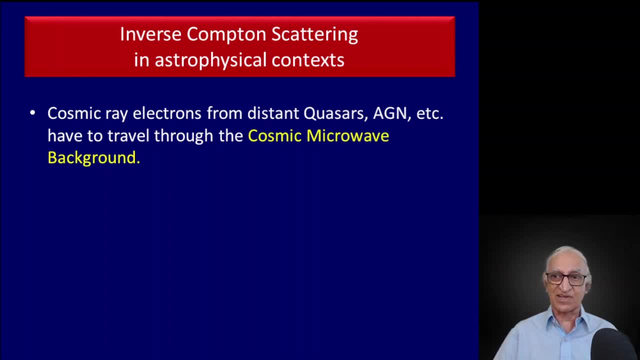 a quasar or active galactic nuclei which is a billion light years away? I don't think so. why? because in between it's not vacuum. the space between the quasar and the sun is filled with cosmic microwave background radiation. it is filled with photons whose energy peaks in the microwave 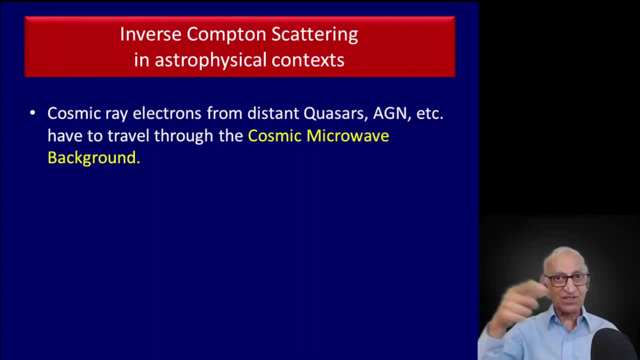 region. these relativistic electrons scatter off the photons, so they will lose energy to the photons. active galactic nuclei have lots of relativistic electrons as well as lots of photons generated by synchrotron radiation. so I am trying to tell you about situations where we have the coexistence of 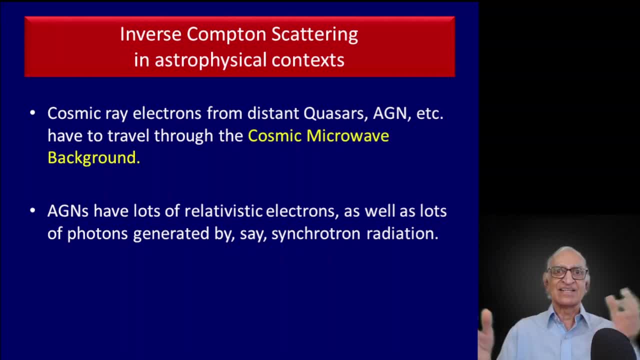 relativistic electrons and a radiation field. therefore, the relativistic electron can interact with the radiation field and the frequency of the photon will be increased by a factor: gamma square. now the question is: how will the spectrum of radiation be modified by compton interaction between the electrons? 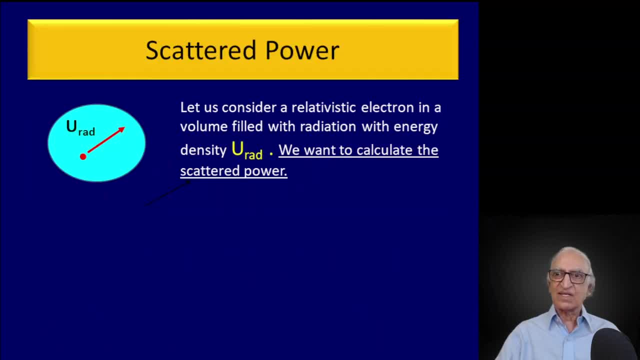 and the photon. let us discuss this. so let us say that there is some region. it could be intergalactic region, it could be in the vicinity of an active galactic nuclei or quasar. there is radiation field. there is radiation- synchrotron radiation- produced by relativistic electrons. 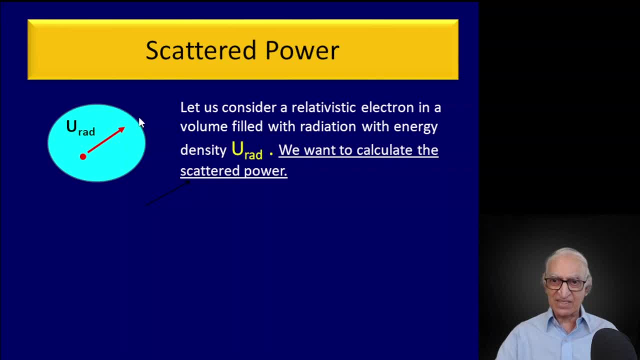 or cosmic microwave background radiation. so there is an energy density- u radiation- and there is a single relativistic electron. now let us consider a relativistic electron interacting with the radiation field. so far we have discussed the interaction of a relativistic electron. now, if i am sitting on top of the 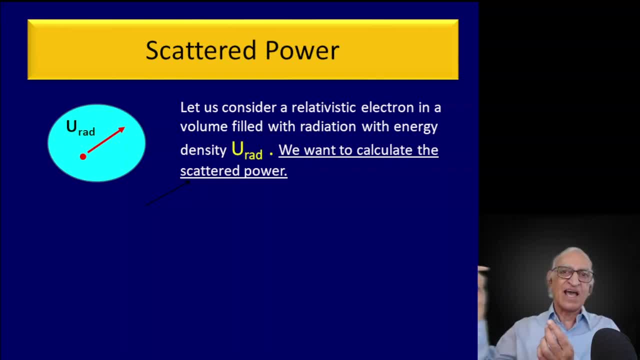 electron. i will find not just a single photon hitting me. i will find photons hitting me from all directions with all possible initial energy of the photon. so all i have to do is, for each scattering i calculate what is the scattered frequency and what is the scattered intensity, and then i integrate over. 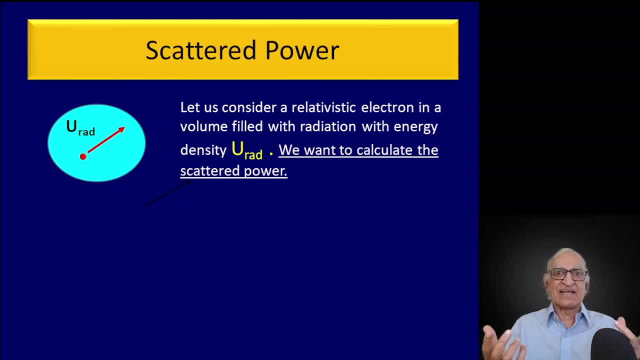 all solid angle over the radiation field, then i get the answer that i want. i hope it is clear to you what i am talking about, so let me repeat it. so far we talked about sitting on top of an electron and asking what will be the consequence of a photon scattering. 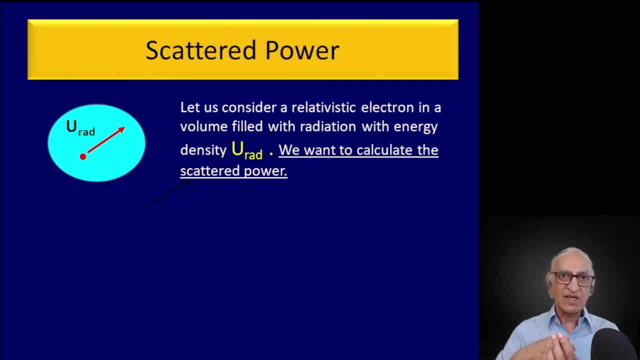 off the electron or in the laboratory frame. now this electron in this picture is being bombarded by photons from all directions, photons with all sorts of energies. so we have to do this calculation properly and calculate the total scattered power. it is very easy to do this calculation. i will not. 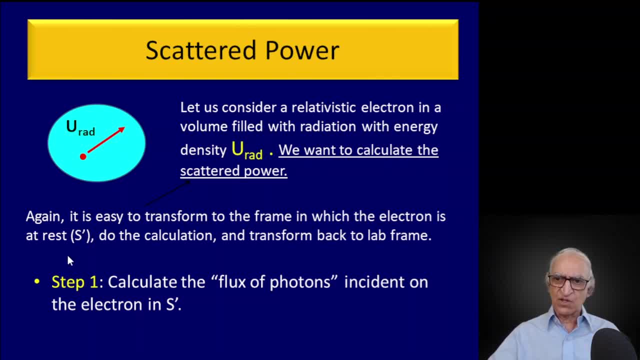 do it for you. there are two steps to this calculation: go to the frame in which the electron is at rest and calculate the flux of photons- flux means the number of photons crossing a unit area per unit time coming and hitting the electron. and step two, calculate the scattered power. 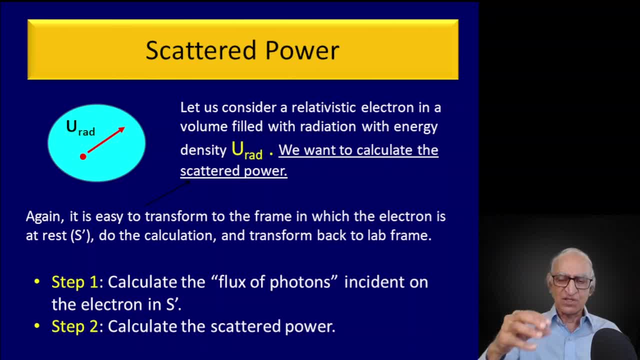 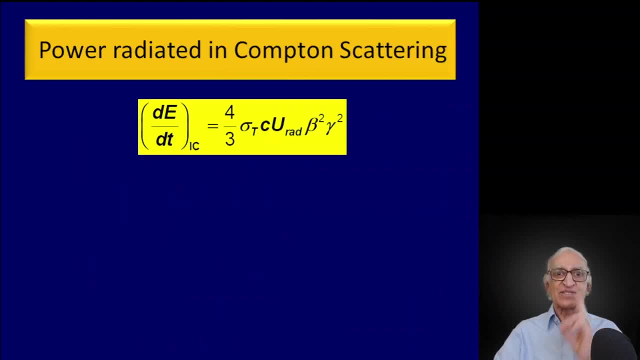 and then jump from the electron rest frame to the, to the frame of the radiation field or the laboratory frame. if you do this calculation, which you will find in all standard books, this is what you will get: the energy radiated per unit time due to compton. 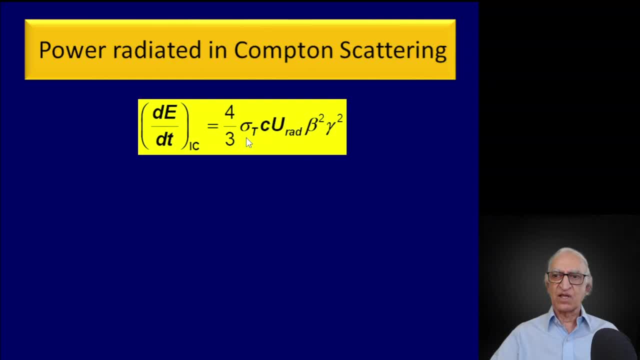 scattering is four by three. thompson scattering cross section sigma t: the speed of light into energy density of the radiation field multiplied by beta squared gamma squared, where beta is v by c and gamma is of course the usual lawrence factor. this is what you get now, some of you. 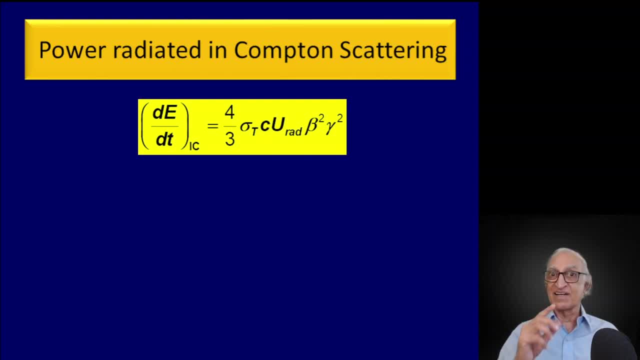 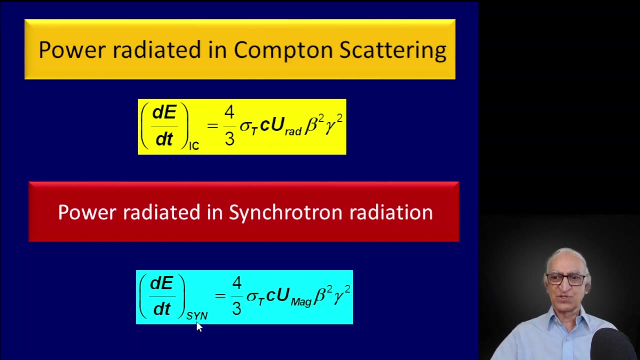 who have carefully studied my lecture on radiation from synchrotron radiation from relativistic electron gyrating in a magnetic field will remember this formula: the energy radiated per unit time due to synchrotron radiation is given by four, by three sigma t, c. 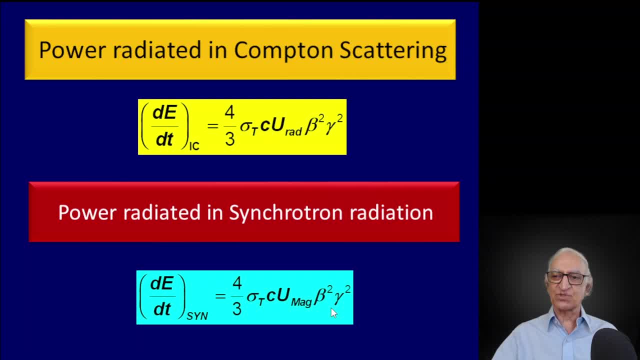 multiplied by b squared, beta squared, gamma squared, where b squared is the square of the strength of the magnetic field. remember b squared, beta squared, gamma squared, since we were talking of relativistic electron, beta is one, so i would have essentially written: capital b squared multiplied by gamma squared. 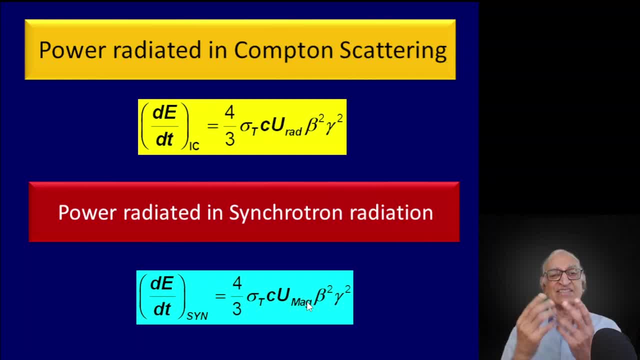 now capital b squared, divided by eight, pi is just the energy density in the magnetic field. so what i have done is to cleverly write the formula for power radiated in content scattering and the power radiated in synchrotron radiation. to look the same, the only 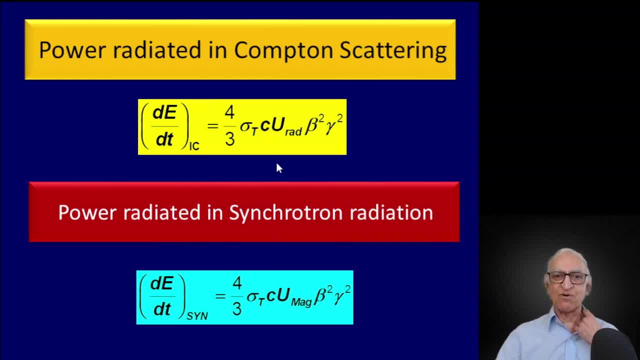 difference between these two formula is in the top formula, which is content scattering, you have the energy density of radiation field, which is interacting with the relativistic electron, and the energy density of the magnetic field, with which the relativistic electrons are interacting. the two formulas look the same. there they 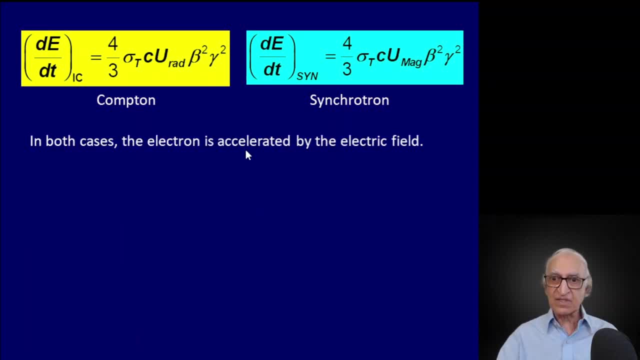 are same formulae over there. now, in both cases the electron is scattered by the electric field. now, in the case of the synchrotron radiation you will say, well, there is no electric field, it is magnetic field. but there is an electric field which is v cross b. 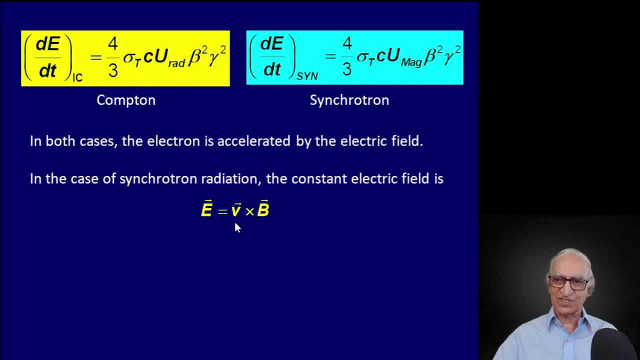 okay, because we wrote the lawrence force as e over c, b cross b, so the electric field is v cross b. in the case of content scattering, which is scattering of a radiation field with electrons, the electric field is a coherent superposition of the electric field of the incident waves. 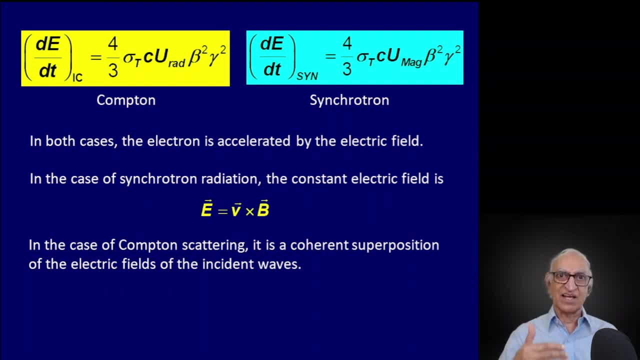 remember the incident wave? according to Maxwell's electrodynamics can be described in terms of an electric field and a magnetic field. you remember, the pointing flux is e cross h and the energy is proportional to e squared or b squared. therefore, in both cases we are dealing with an electric 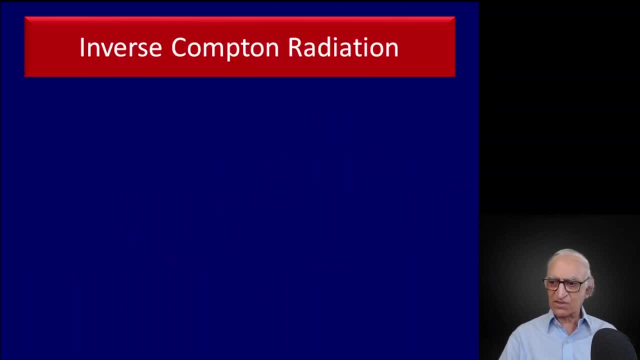 field. now let us go back to inverse content scattering. it is easy to show that the photon will gain maximum energy in a head-on collision. so if h bar omega naught is the energy of the incident photon in a head-on collision of a relativistic electron, the photon 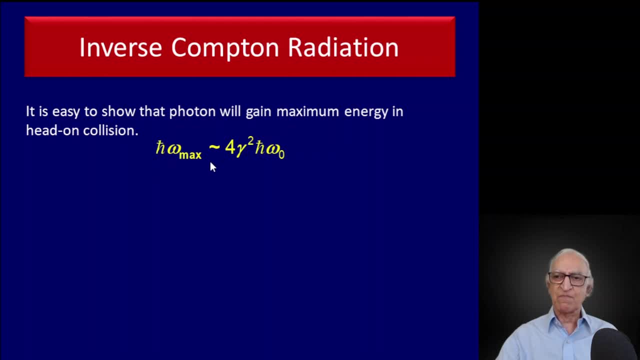 scattered photon will have an energy h bar omega max, which is four gamma squared into h bar omega naught. this is the maximum of the most favorable configuration for energy loss. now photon and electron can scatter at various angles. now if you do the average, you find you pick up. 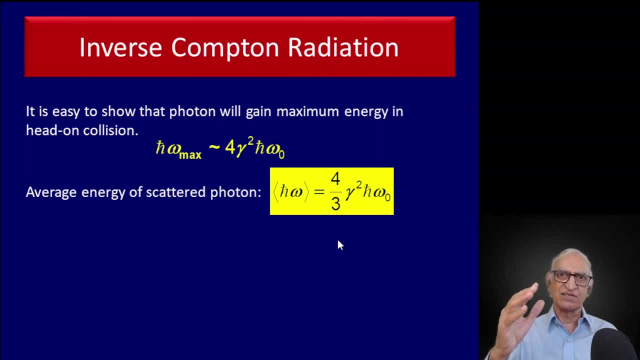 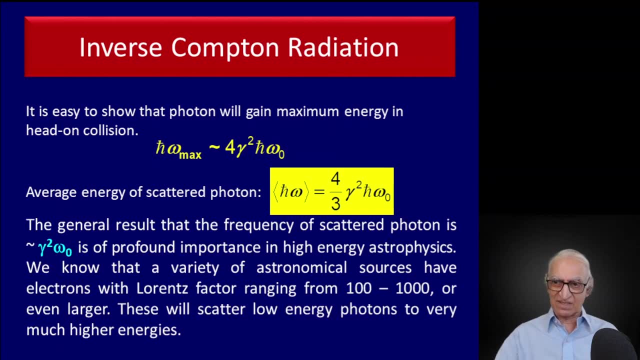 four by three times gamma squared h, bar omega naught. I leave this to you. if you are brave enough, you can do this calculation. now the general result: this is important. listen to this carefully. the general result: that the frequency of the scattered photon is gamma squared times the 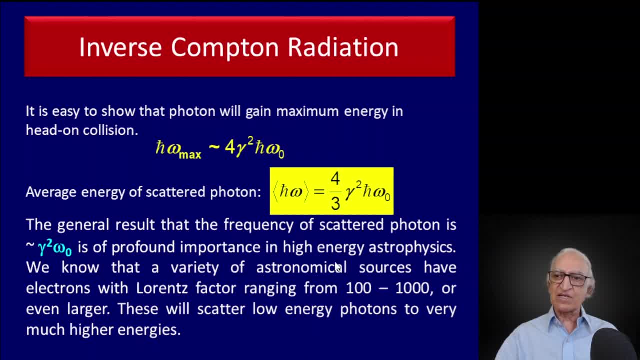 frequency of the initial photon is a profound importance in high energy astrophysics because, you know, a variety of astronomical sources have electrons with Lorentz factor ranging from ten to a thousand or even larger, and we are talking of gamma squared, so we are talking about a million. 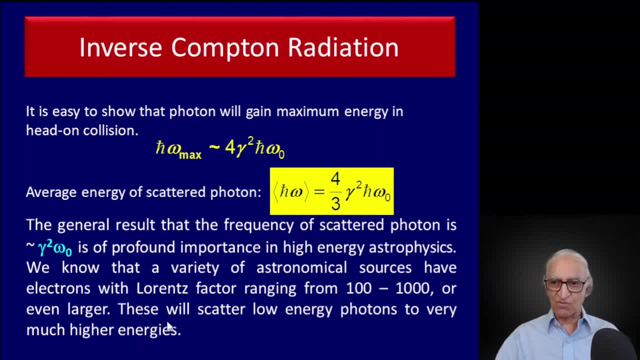 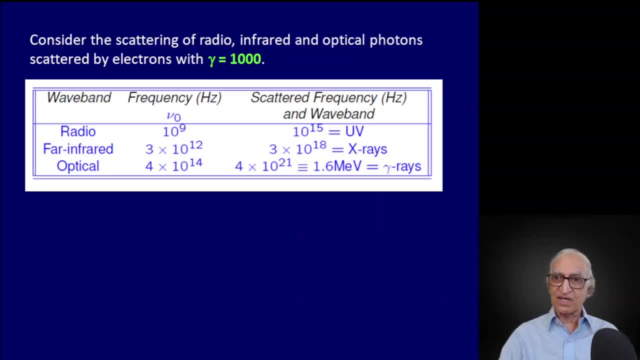 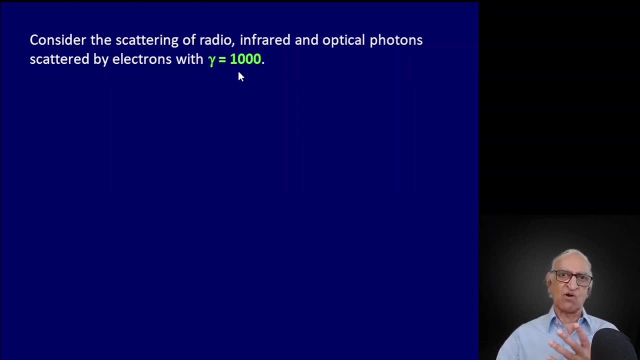 boosting of energy of the photon by a million or more. therefore, your low energy photons will be scattered to very high energy. so here is an example. let us consider an electron with a gamma of a thousand. it's a fairly modest relativistic electron. now, if you are dealing 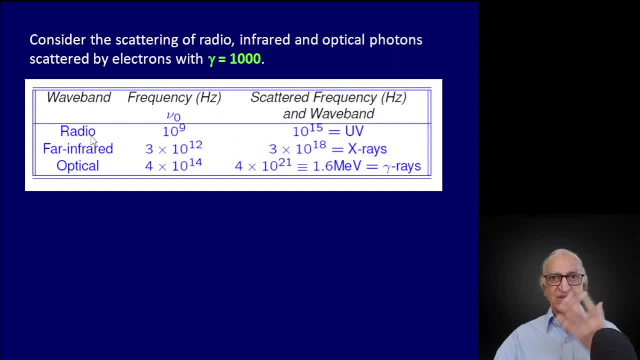 with scattering of radio waves in a radio galaxy. the frequency is about ten to the nine hertz. it will be scattered to ten to the fifteen hertz, which is ultraviolet. so radio photons will be scattered to ultraviolet energies. the far infrared photon will be scattered to x-ray. 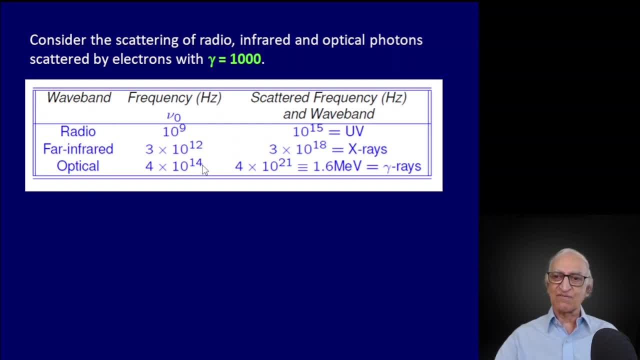 energy. an optical or a visible wavelength photon will be scattered to gamma ray energy. so this is how you produce gamma rays. you produce gamma rays not by the original process, but all I need is photons which have energy in the visible wavelength, a few electron volts and, if I have relativistic electrons, 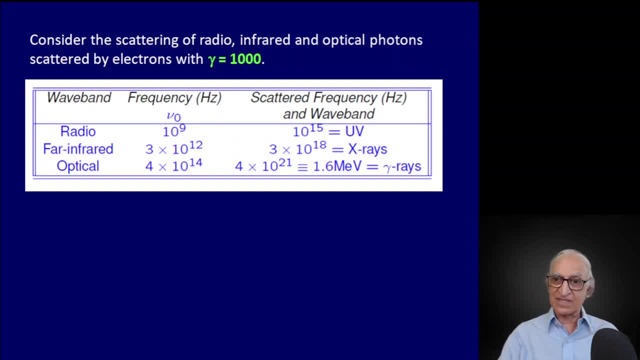 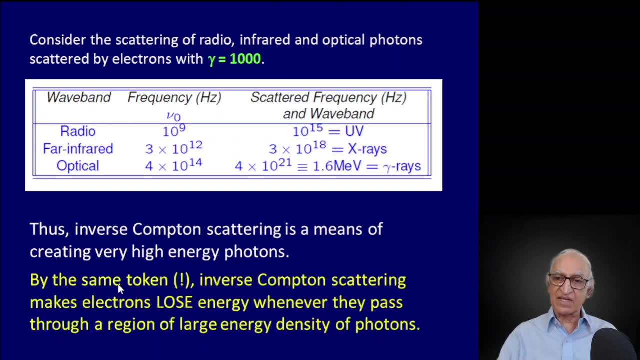 gamma squared times that energy is in the gamma ray region. thus inverse complex scattering is a means of creating very high energy photons. by the same token, the electrons are also losing energy. so inverse complex scattering is also a mechanism whereby electrons lose energy because they are giving their 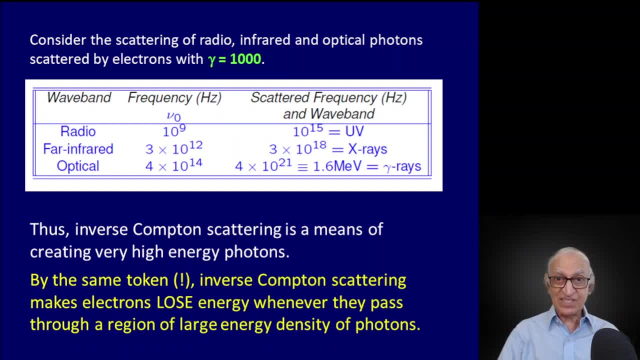 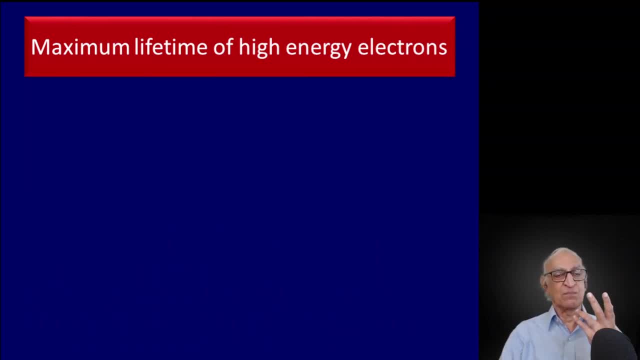 energy to the photons. now this can have very important consequences. for example, I already said cosmic rays presumably originate in powerful sources like black holes and so on, far away now. but those cosmic rays, electrons, will have to travel through cosmic microwave background radiation. the energy density of a 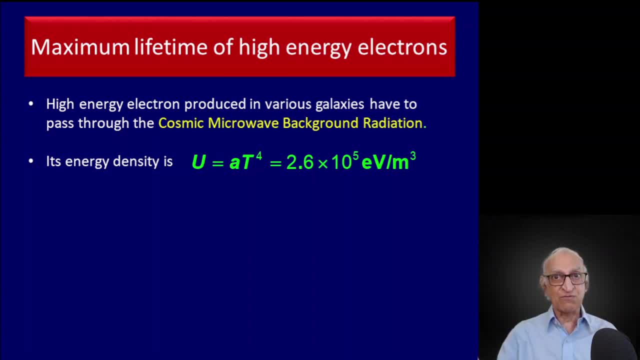 radiation field is AT to the power 4, where A is Stefan's constant and T is the temperature. now we are talking of a temperature of 3 degrees Kelvin. now the energy density of the cosmic microwave background radiation which fills the universe, about which we will discuss. 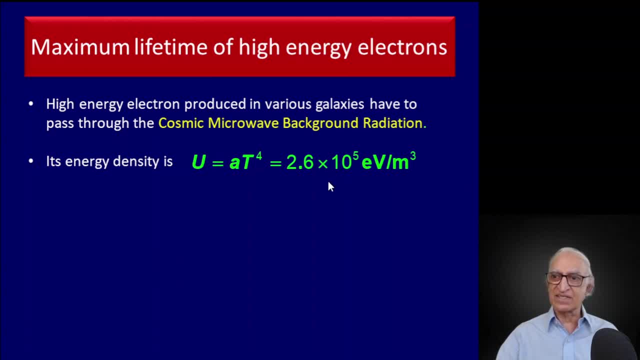 in our lectures on cosmology. has this energy density, therefore the lifetime of the electron, the same old thing? like we discussed the lifetime of the stars, we discussed lifetime in synchrotron radiation. it is the energy of the electron divided by the rate at which the electron is losing energy. 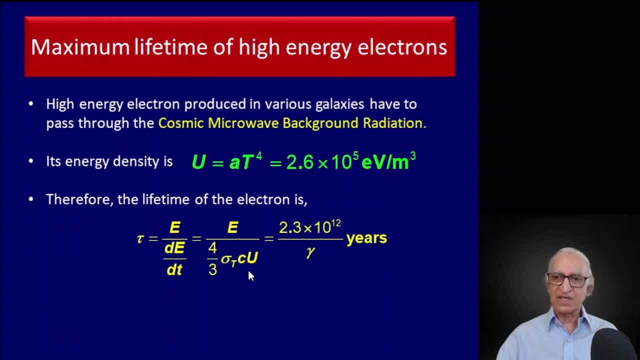 in this case, the electron is losing energy in quantum scattering and that is the formula over there and the lifetime of the electron, or the time over which the electron is lose a significant amount of its kinetic energy, is given by this formula: 10 to the power, 12 years by gamma. 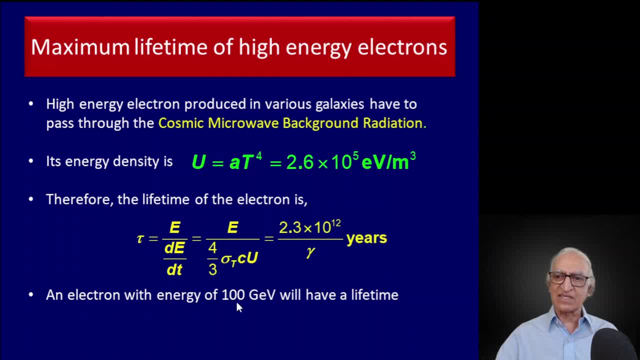 now, an electron with an energy of 100 GeV will have a gamma of 10 to the power 5. why energy of the electron is half a million electron volt, half times 10 to the power 6 electron volt. alright, that is gamma mc squared. 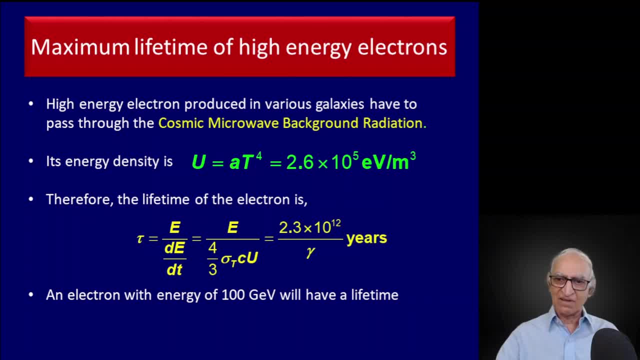 therefore, if I have an electron with an energy of 100 GeV, that corresponds to a gamma of 10 to the power 5. so if I put in 10 to the power 5 in the denominator there I will get a lifetime of 10 to the 7 years. 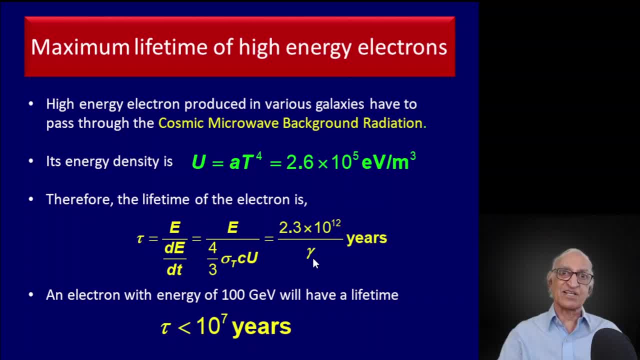 so our cosmic rays cannot come from a quasar which is at a distance of a billion light years away, because even light takes billion years to reach us and the electron needs only 10 million years before it loses all its energy. so the quantum interaction between relativistic 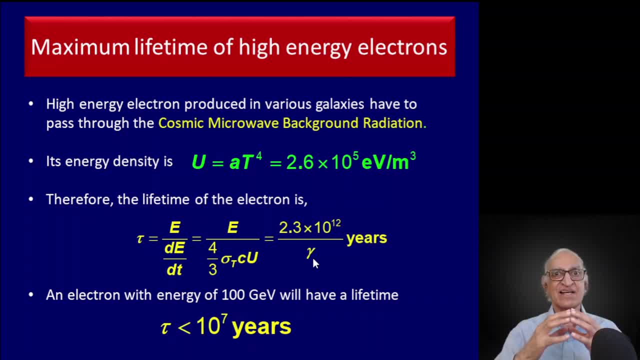 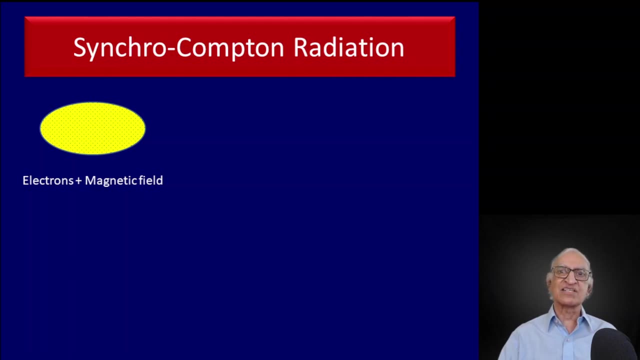 electron and the background radiation that fills our universe has very important consequences for the origin of cosmic rays that we detect here on earth. now, please permit me a few moments. I want to discuss something terribly interesting and exciting. that is, the concept of synchro quantum radiation. 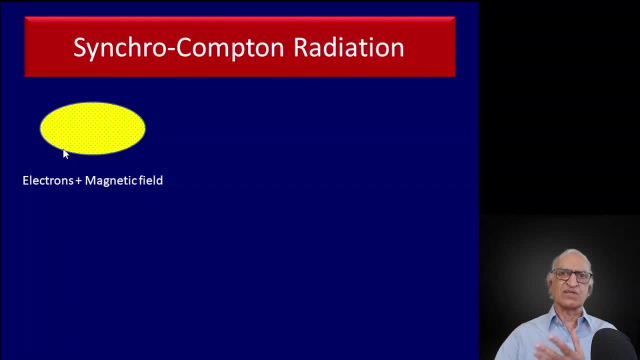 so what I have is some source, an active galactic nuclei, quasar. what have you where? the electrons and a magnetic field. these electrons will direct to the magnetic field and these electrons will produce low energy. photons may be radio radiation, may be infrared or visible radiation by synchrotron radiation. 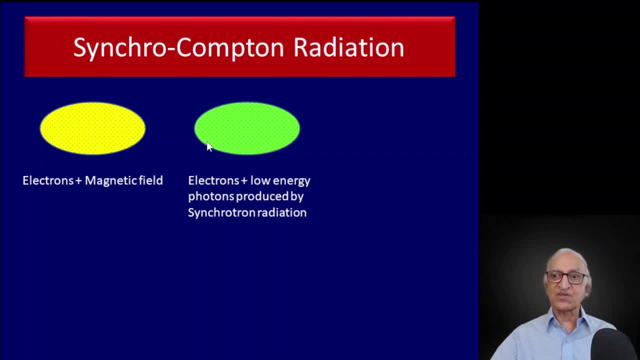 so I now have not only relativistic electrons and magnetic field, but I also have photons. now these relativistic electrons will scatter off the photons which were created by synchrotron radiation, and these electrons will be now scattered to ultra high energies by inverse content scattering. 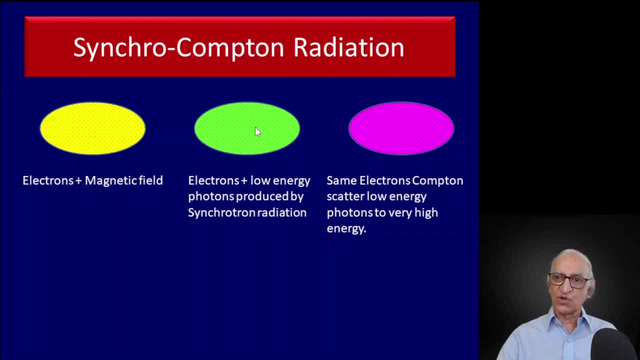 so I have synchrotron radiation, and those photons have been upgraded to very high energy by content scattering. now, when the same electrons are involved in both synchrotron radiation as well as content scattering, these electrons will transfer to a synchro content radiation. 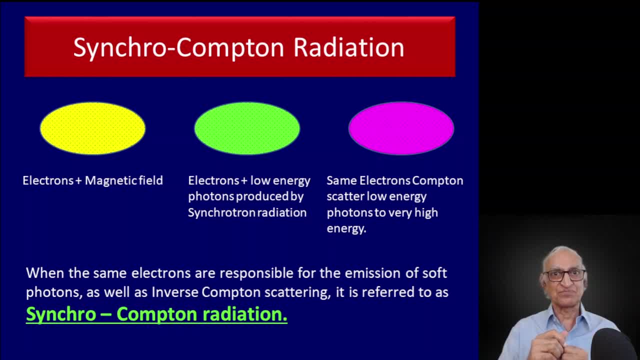 so what I have is some active galactic nuclei where there are relativistic electrons which have produced low frequency photons by synchrotron radiation. it is the same radiation interacting with the same relativistic electrons, boosting its energy to ultra high energies by content scattering, that is, synchro content radiation. 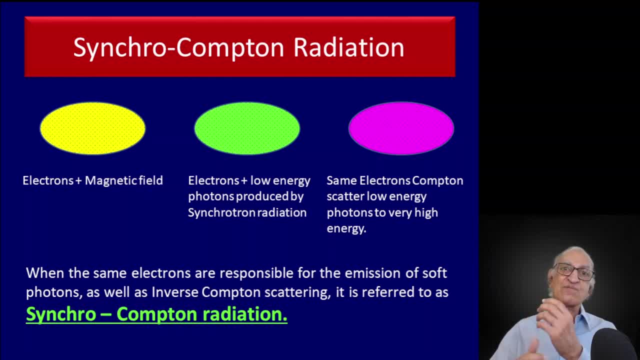 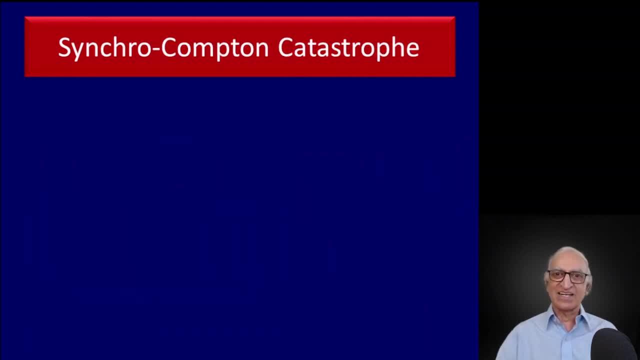 the combination, it is content radiation riding on the back of synchrotron radiation, if I might put it that way. now you can have a catastrophic situation. what do I mean by that? let eta be the ratio of the energy loss rate of an electron by inverse content scattering. 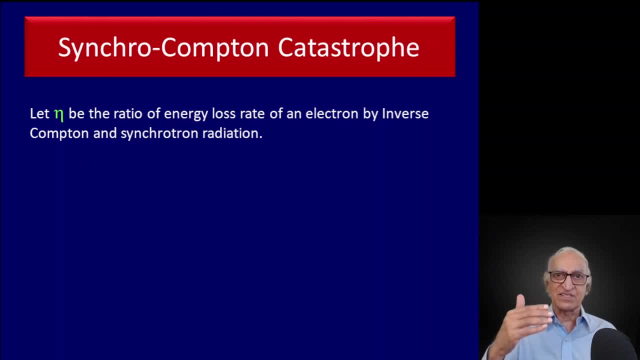 divided by the rate of energy loss rate by synchrotron radiation. remember, an electron in an active galactic nuclei loses energy both when it emits synchrotron radiation, because that energy of the photon has to come at the expense of the energy of the electron. 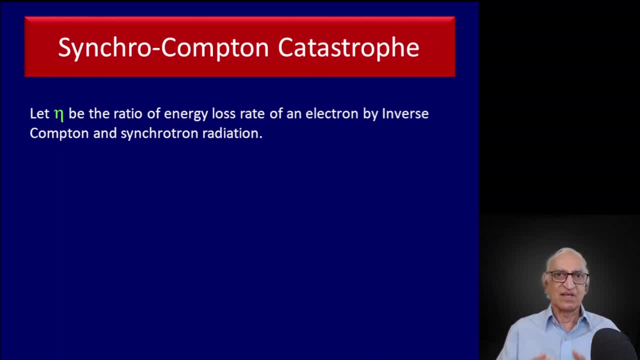 it is also losing energy by inverse content scattering the two formulae I have shown you little earlier. and let us say: this is the eta, is the ratio of this energy loss rates? now, a catastrophe will occur if gamma, if eta exceeds one, because what happens is when eta 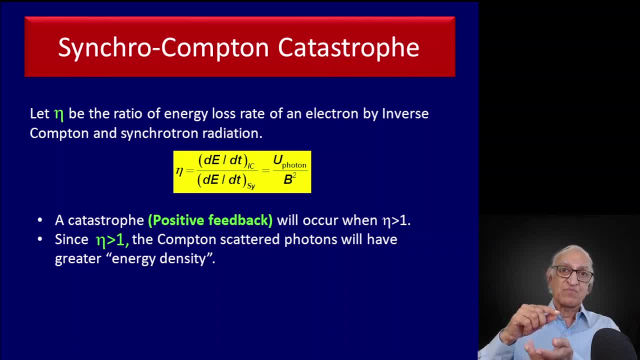 is greater than one. what it means is that the energy lost by the electron through content scattering is more than the energy lost by the electron in synchrotron radiation. so following very interesting thing will happen: the electron produces synchrotron radiation, and that synchrotron radiation 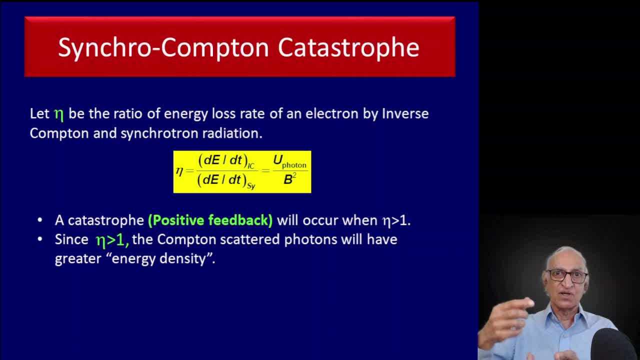 is immediately boosted to gamma ray energy, so the intensity of synchrotron radiation does not increase beyond a certain point, and what you will find is that finally, all the energy of the electrons will be lost in inverse content scattering, and there will be no more energy left. 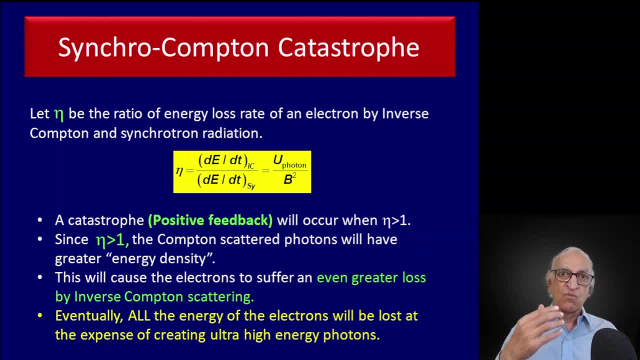 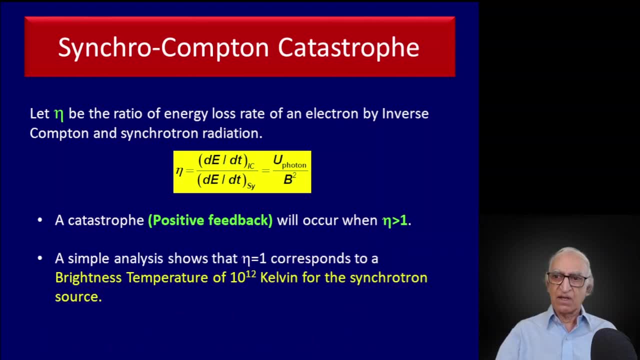 in the electrons to produce more synchrotron radiation. the implication of this is the following: if you look at compact radio sources which are seen by intercontinental very long baseline radio interferometers, you detect synchrotron radiation from quasars blobs emitted by quasars. 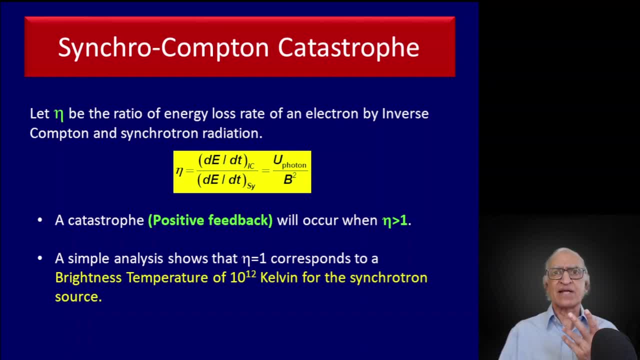 and so on. these are very high brightness temperature. brightness temperature is a measure of the intensity of radiation. it is the temperature of a hypothetical body which will emit the same amount of energy at that particular frequency. now what radio astronomers have found is that when you look at extremely 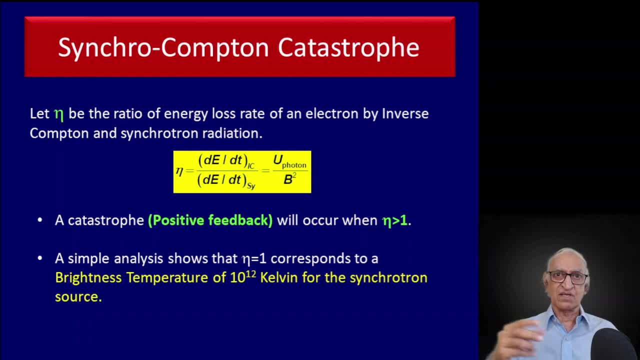 compact synchrotron sources with intercontinental baseline interferometry with an angular resolution of milli arc. second, there seems to be a limit to the brightness temperature, and the limit to the brightness temperature is around 10 to the power, 12 Kelvin. it is almost as though 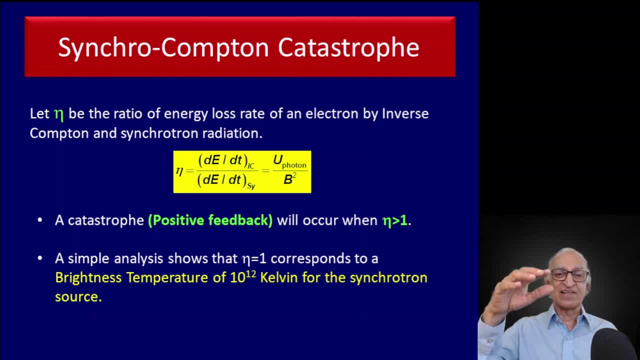 like in Chandrasekhar mass limiter white dwarfs, when the bucket fills and the mass reaches 4 solar mass, the bottom drops out and there is a collapse. similarly, if the intensity, if the brightness temperature of the synchrotron source reaches 10 to the power, 12 Kelvin. 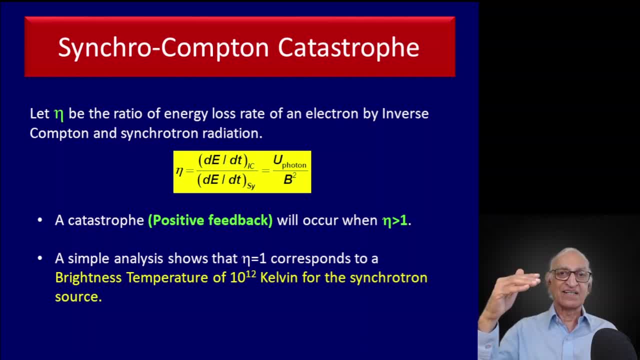 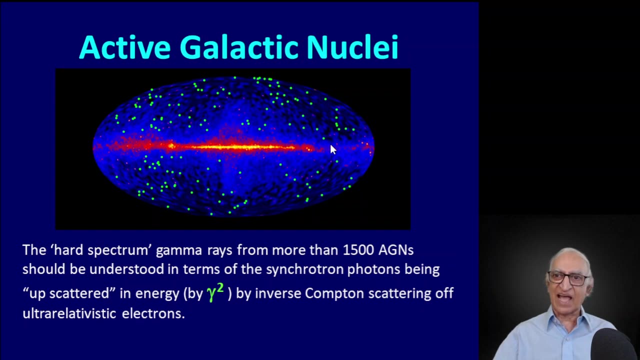 then the inverse Compton scattering reaches a catastrophic efficiency and the brightness of the synchrotron source never increases beyond about 10 to the power 12 Kelvin. and now this active galactic nuclei, seen in gamma rays by the Fermi Large Area Telescope, one believes 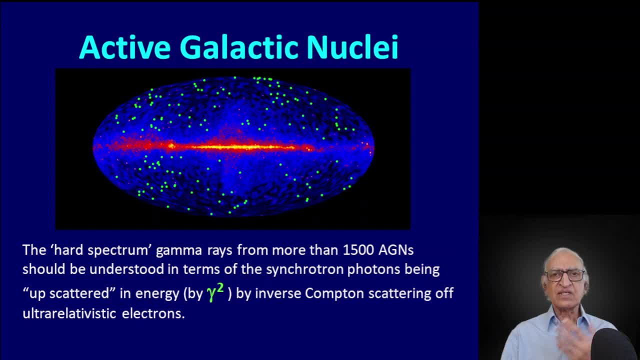 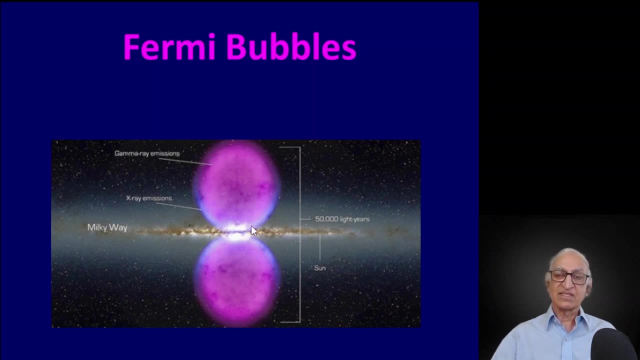 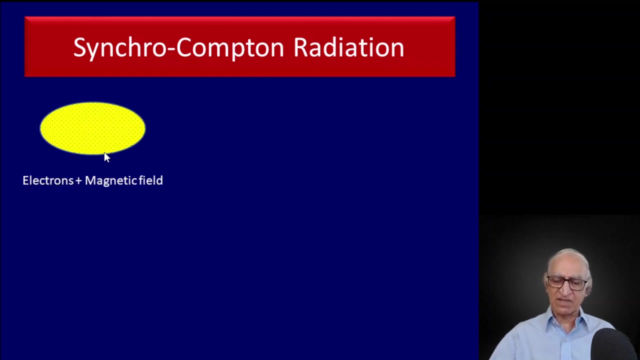 that the only possible mechanism is inverse Compton scattering of synchrotron photons, of relativistic electrons. finally, to conclude, let us go back to this giant gamma ray bubble near the center of our galaxy. as I said, there are electrons and the magnetic field, the electron gyrating in the magnetic field. 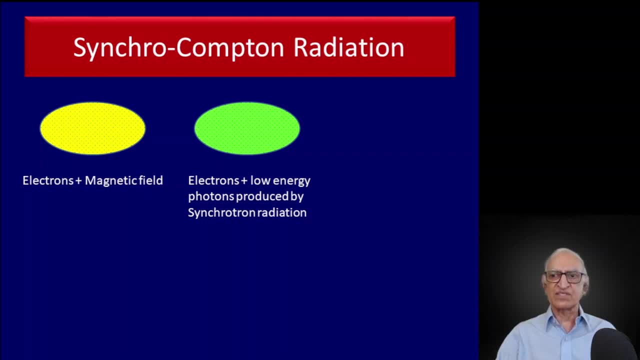 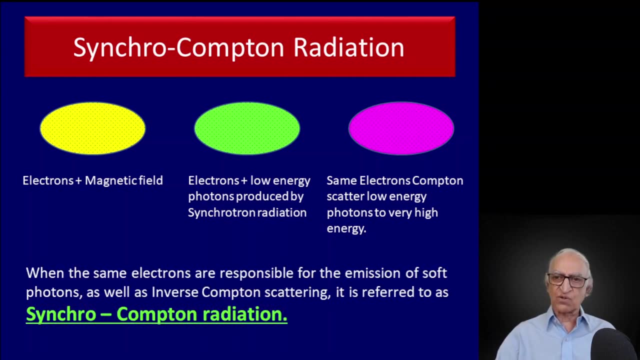 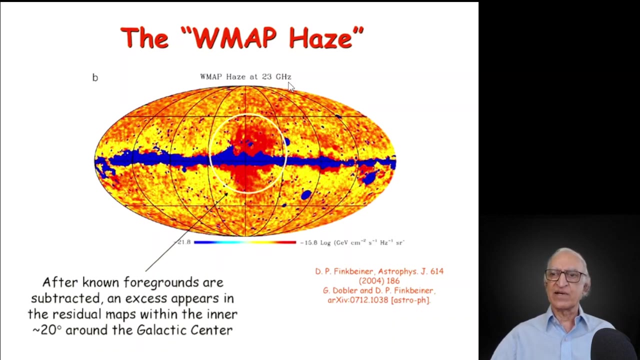 produce synchrotron radiation. the electron scattering of the synchrotron photon produce ultra high energy Compton scattered photons- synchro Compton radiation. now here is our galaxy in the microwave spectrum at 23 gigahertz, taken with the satellite known as WMAP. 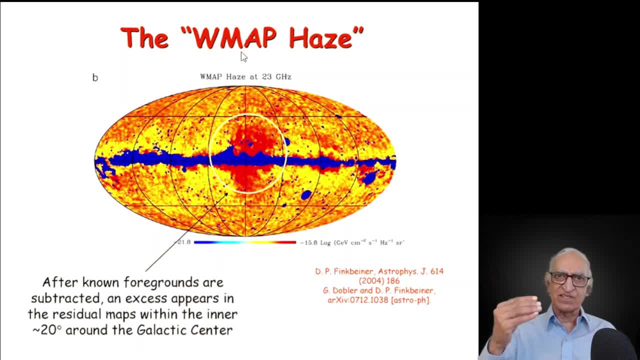 we will discuss this at length when we discuss cosmology. all I want you to see is that, looking straight near the center of the galaxy, you see something like the bubble. this is synchrotron radiation produced by electrons emitted by from the vicinity of the central.